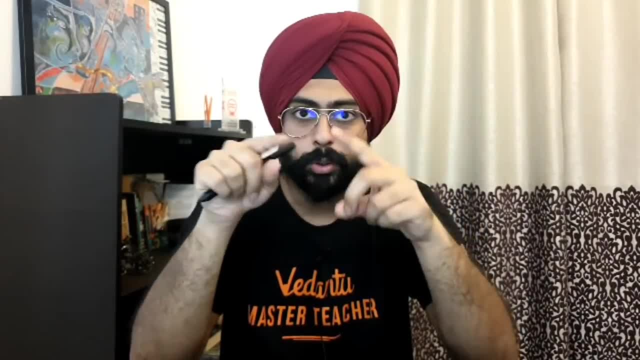 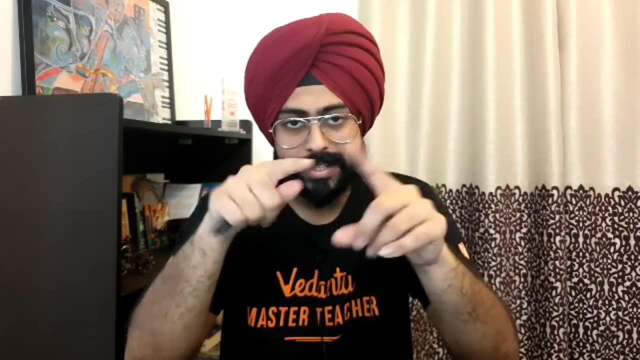 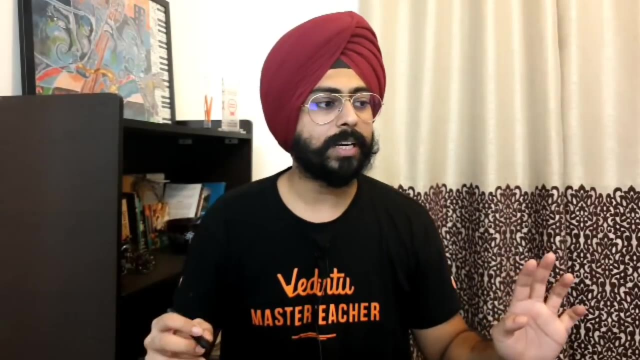 just two formulae. There is one formula where you write: dr by dt is equal to k times R0 to the power n Yes, And the other formula is: k is equal to Rrhenius into e, to the power minus ea by RT. That's all. These are the two formulas in this chapter of Chemical Kinetics. 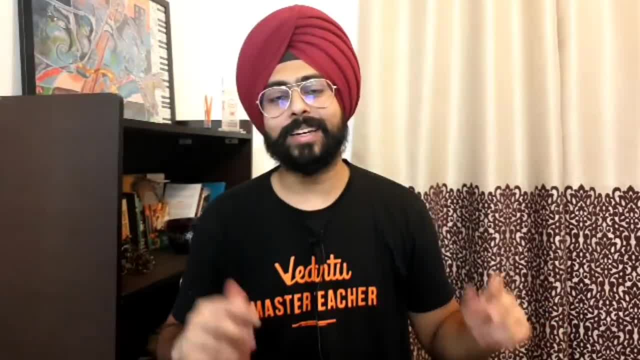 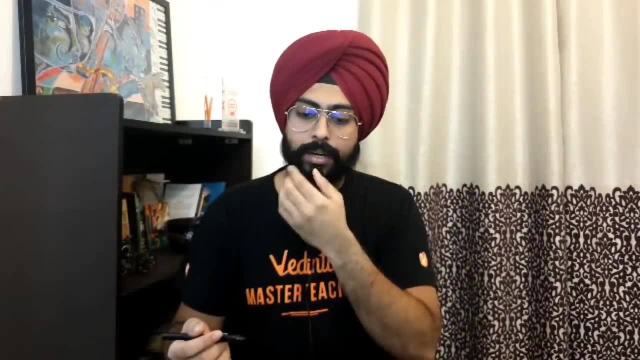 In case you want to leave, you can leave right now. Quickest revision ever: Five minutes and we are done. But there are a few more details that you can derive out of these things and the theoretical analysis. So today's revision class is going to be very chilled. And the good thing about 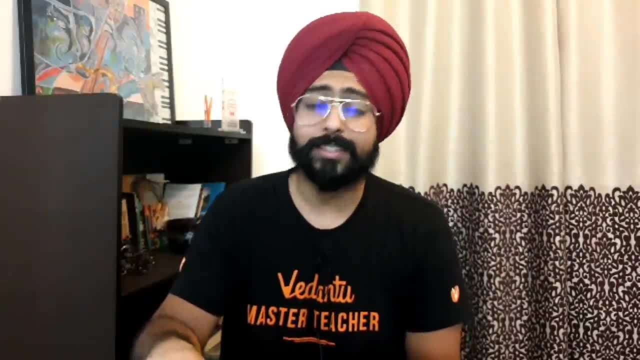 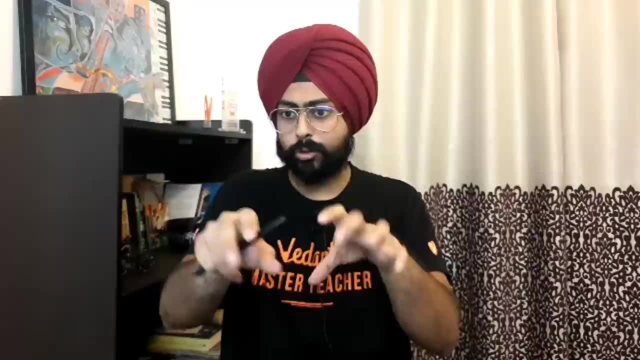 Chemical Kinetics is that it's not a very difficult chapter. It's a very easy chapter And the questions that come out of it have a lot of numbers etc in them. You have to analyze a lot of numbers. Sometimes there is a lot of trial and error involved, And 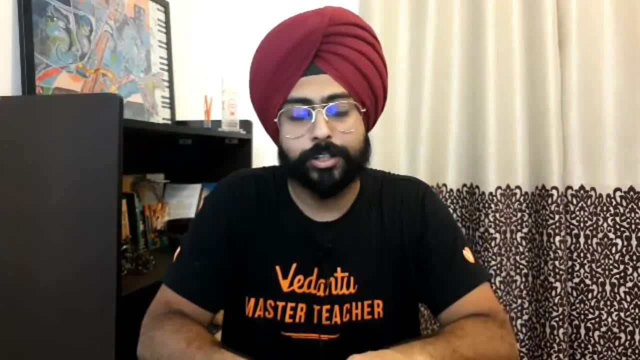 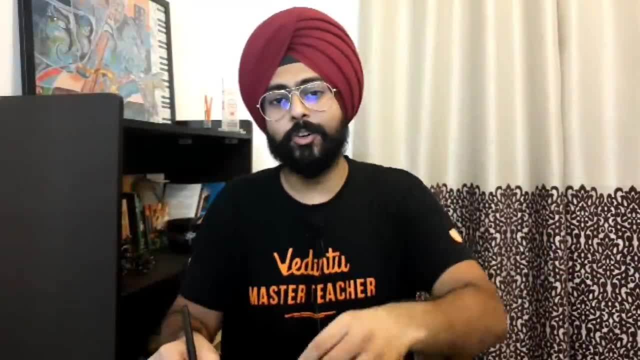 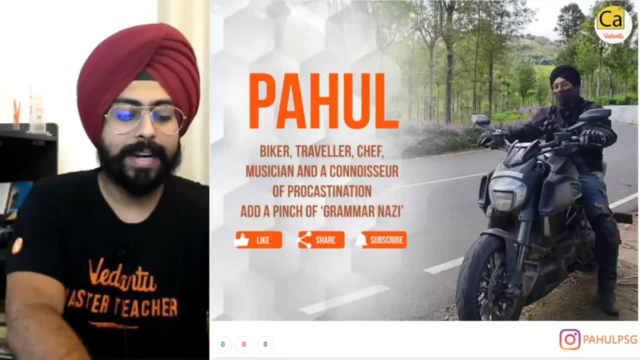 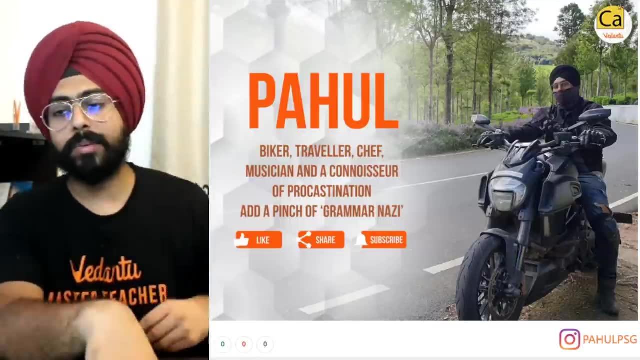 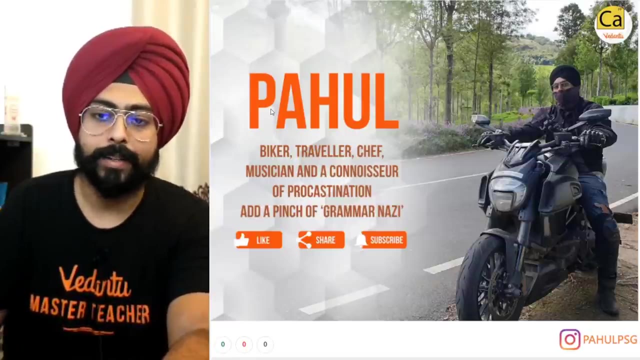 to the channel. please welcome to catalysis by Vedantu. My name is Pahul, I am an alumnus of IIT Bombay And I've got lots of hobbies. One of them is traveling around on my motorcycle, which I'm not able to do because of the lockdown. Sadly, I can't do anything. What can I do? 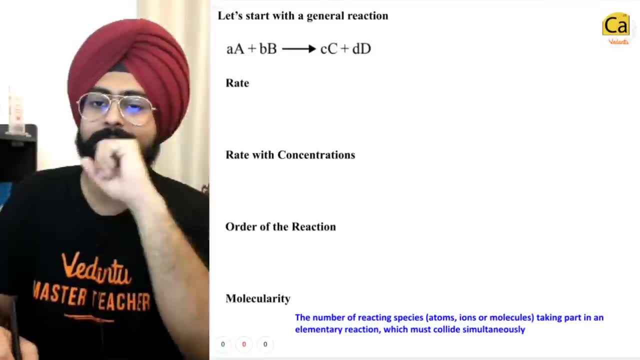 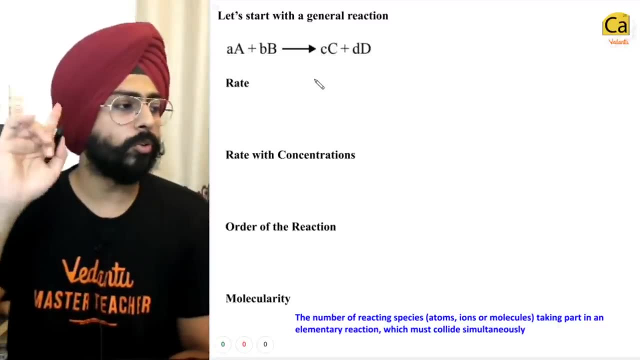 So let's get into chemical kinetics now. Very quick revision. Hardly it's going to take us 15 minutes. So let's start with a general reaction. AA plus BB goes to CC plus DD, Very simple: What's the rate of this reaction? Rate of this reaction can be written as minus. 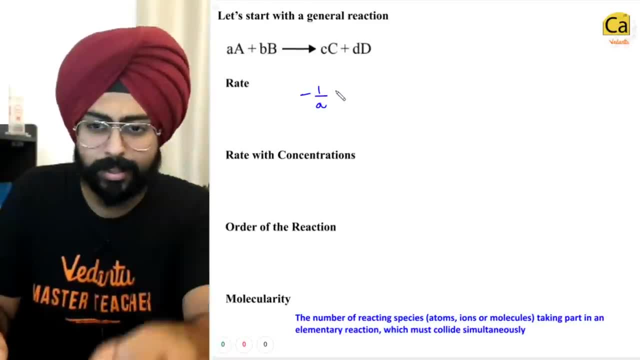 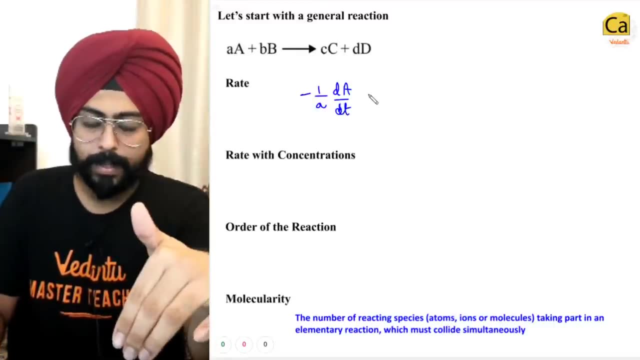 1 by A DA by DT. This is something that we did in chemical equilibrium as well. Yeah, because the reactant will be decreasing. This is equal to minus 1 by B DA by DT. This is equal to minus 1 by B DA by DT. This is something that we did in chemical equilibrium as well. 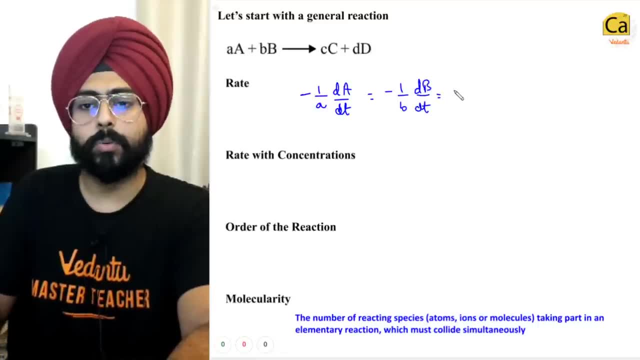 Yeah, because the reactant will be decreasing. This is equal to minus 1 by B, DA by DT. This is equal to plus 1 by C, DC by DT. Why plus? Because the product is increasing, which is also equal to plus 1 by small d into D of capital, D by DT. Very simple, This is how you write. 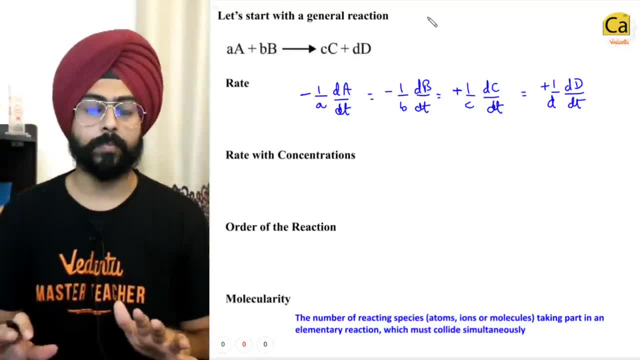 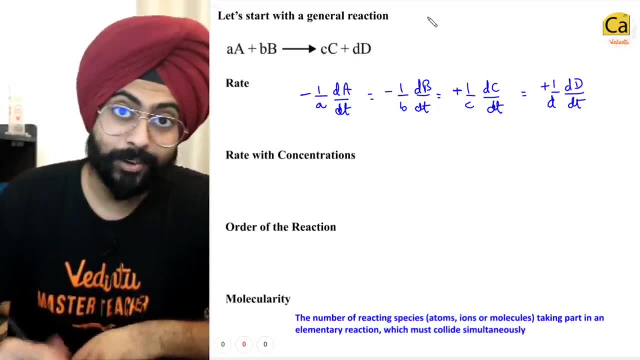 the rate of the reaction. Rate of the reaction is like speed of the reaction. Equilibrium is attained after the reactions have done themselves. That is something that we discussed in chemical equilibrium, Yeah, but our reaction is now talking about the speed at any instantaneous point of time. 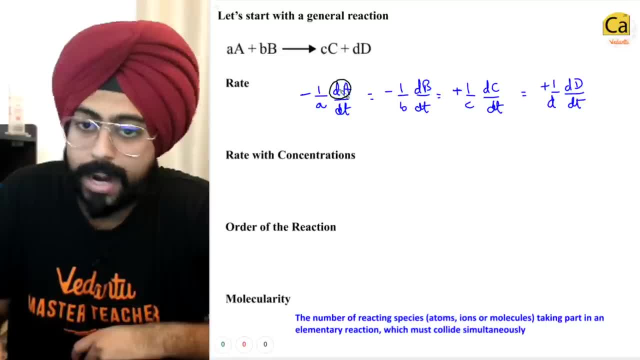 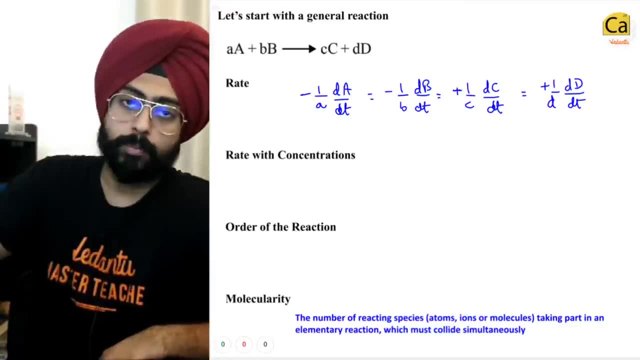 in the reaction. So over here do you notice we have taken DA and not delta A. If this was delta A by delta D, then that would be average rate. DA by DT is instantaneous rate at any point of time inside the reaction. okay, Now if you want to write the rate law. 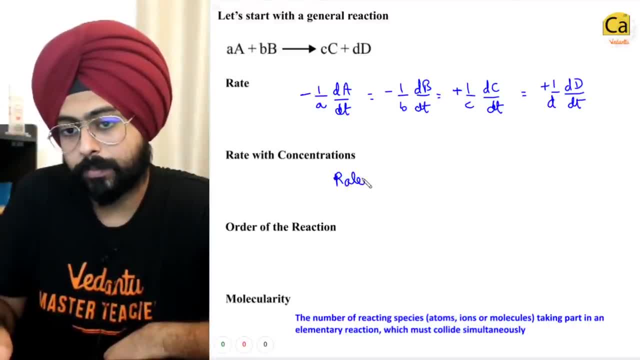 with concentrations. I can write: the rate is equal to. okay, the rate is equal to. what can we write over here? K? What is k? K is the concentration of the rate. The concentration of the rate is equal to. you can write: the rate is equal to the rate, which is the rate. 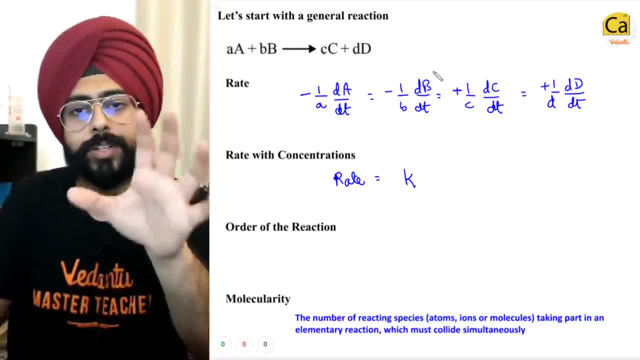 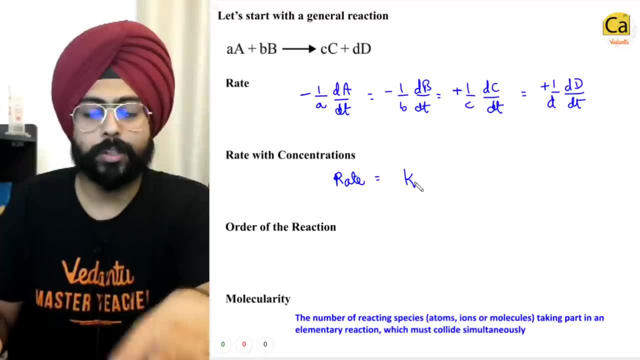 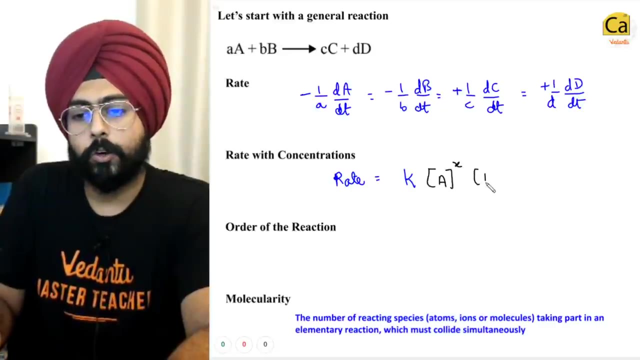 What is K? K is the rate constant. This is determined experimentally or it is determined by putting values in the rate equations. Yes, rate law jitne bhi hota hai. So K into the reactants, let's say A to the power X, into B to the power Y, assuming that the reaction 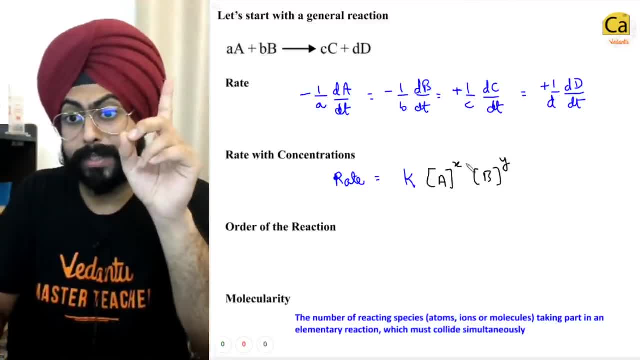 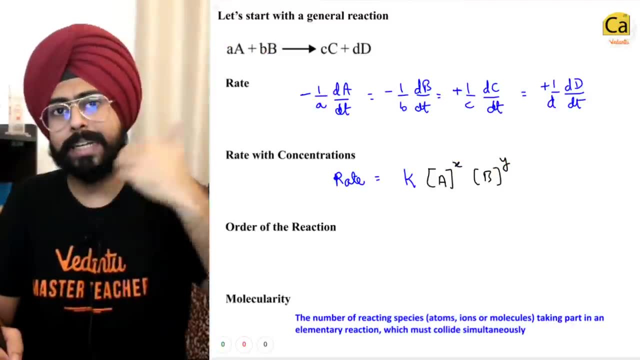 is going forward from A and B In equilibrium, you notice that these X and Y turn themselves into these stoichiometric coefficients A and B. that is applicable for the equilibrium, but in general in a rate law. this is what you can write overall. X and Y are coefficients. 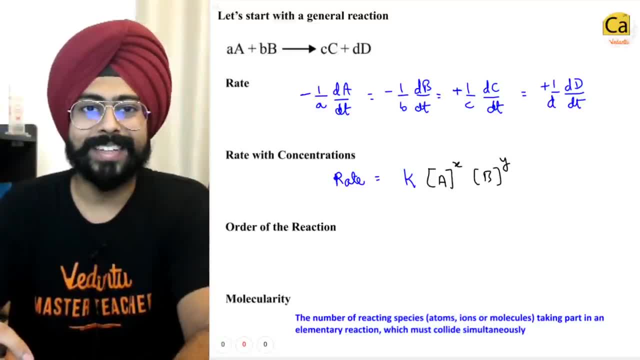 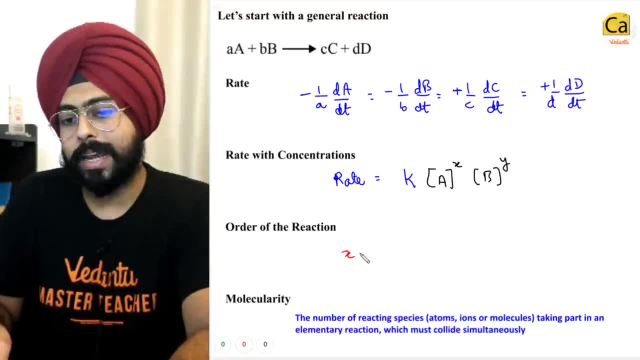 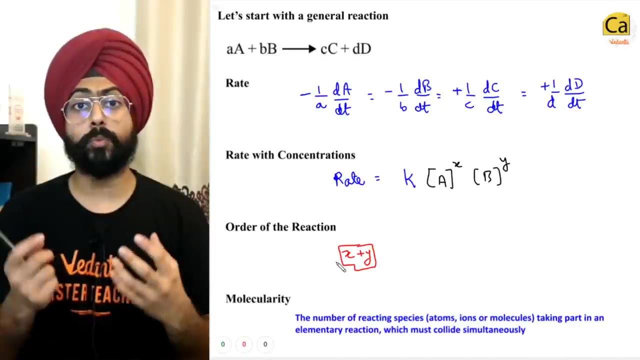 that are determined experimentally. Okay, Okay, X and Y are coefficients that can be determined experimentally and order of the reaction is nothing but X plus Y. Okay, Order can be defined for an elementary reaction. Elementary reaction would be one step reaction. 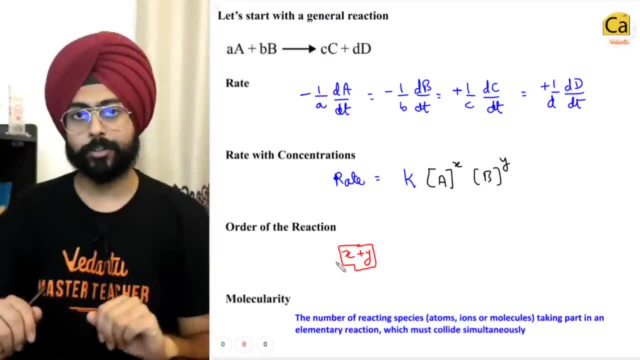 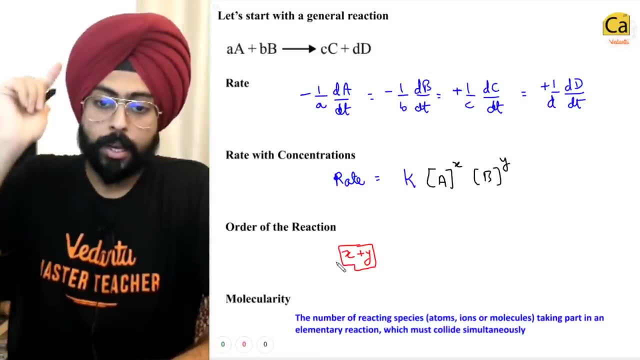 Multiple one-step reactions combined together to form our complicated reactions. yes, and over there as well. for the overall rate of the reaction, you could define an order of the reaction fine. On the other hand, molecularity of the reaction can be defined only for elementary reactions. 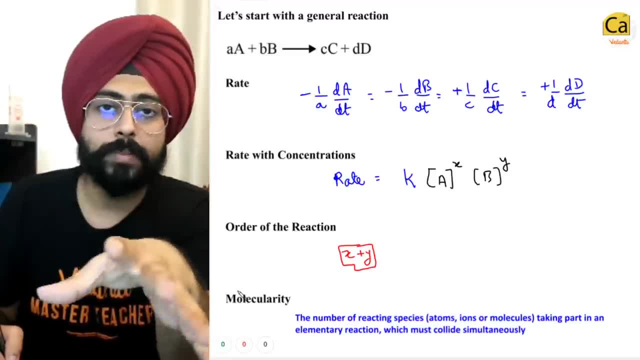 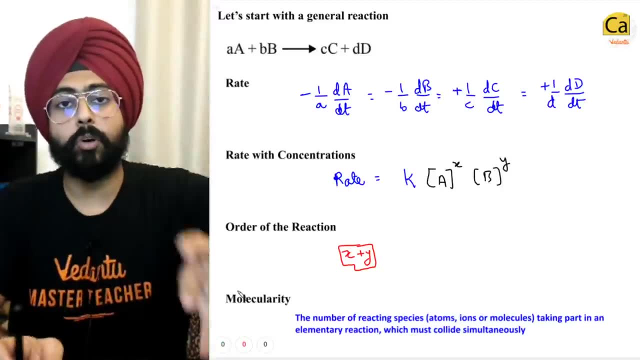 only for single-step reactions. molecularity does not make sense for overall complicated reactions. even if someone says that this is a huge complicated reaction with 5-6 steps and the molecularity is 2, it means that in the rate-determining step 2 molecules 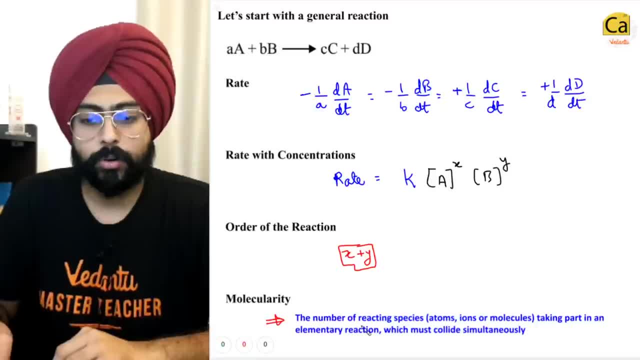 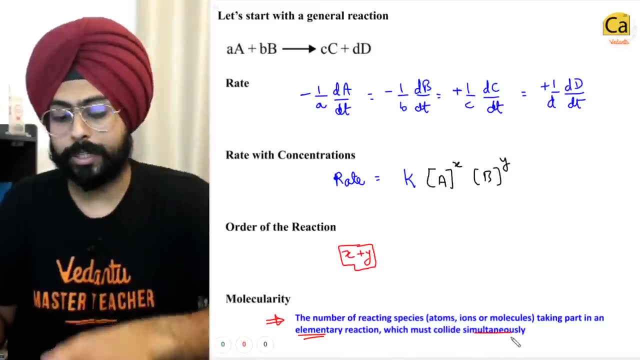 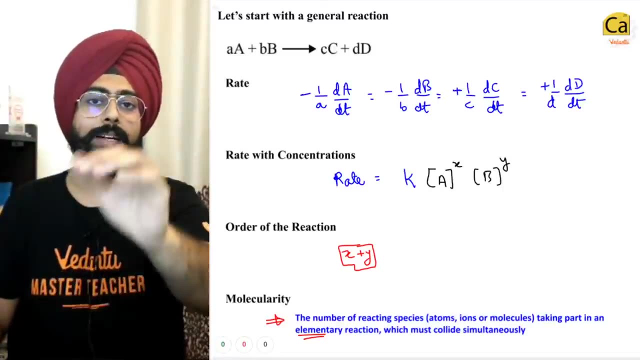 are colliding with each other. okay, so molecularity is the number of reacting species, atoms, ions or molecules taking part in an elementary reaction which must collide simultaneously and more often than not. more often than not, the order of a reaction is equal to the molecularity. 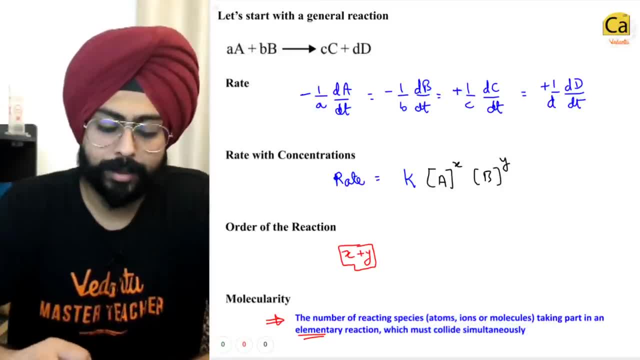 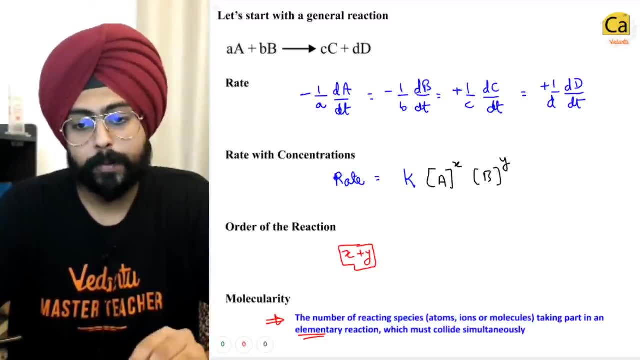 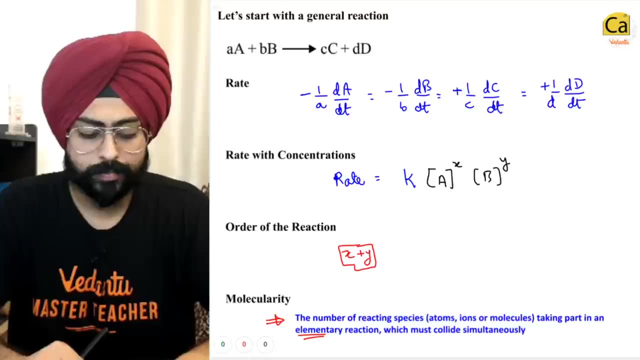 of the elementary step or the rate-determining step. now, that is true almost always, not every time. okay, sometimes the order is absolutely different, like 0th order: reactions: yeah, the order is 0, but molecularity: obviously at least 1 molecule has to be involved. order: 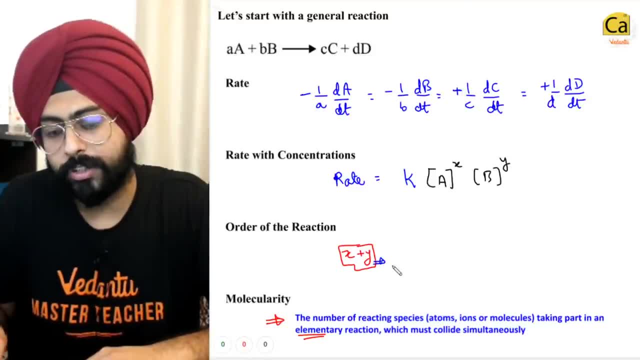 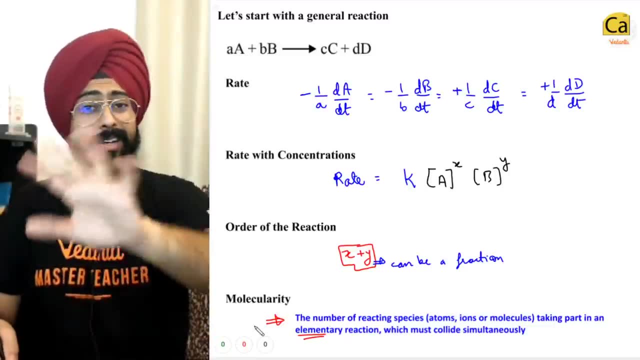 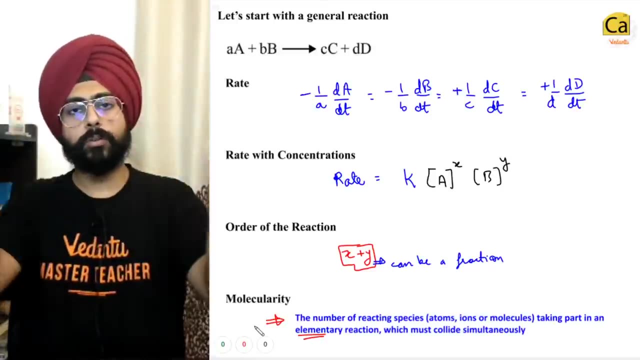 of the reaction can be a fraction as well. okay, order of the reaction can be a fraction, can also be 0, we know that. but molecularity can't be 0, it has to be a whole number. either 1 molecule is there, or 2 molecules like SN2, or 3 molecules, so on and so forth. 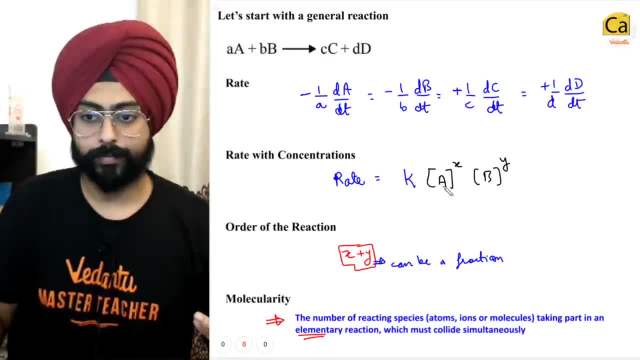 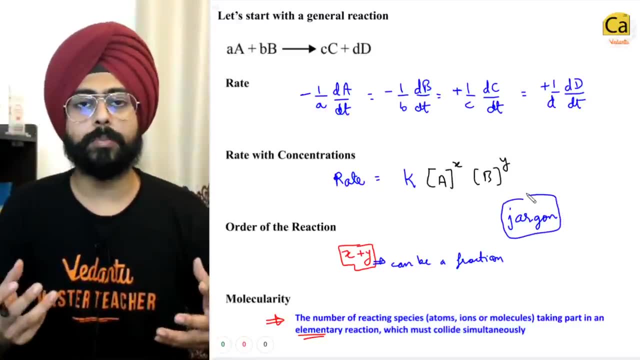 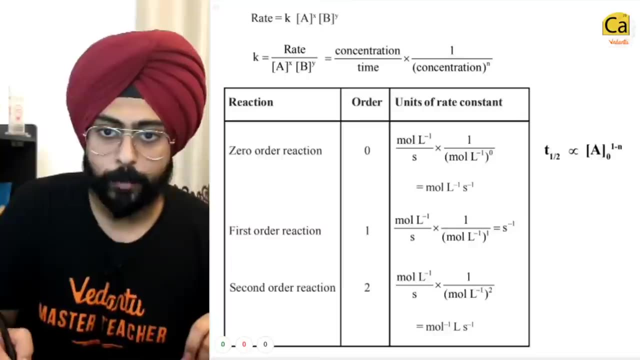 So this is the basic idea behind the jargon. okay English with Pahul sir. what does jargon mean? Jargon is a fancy word for vocabulary that people of a certain profession use. so since we are chemists, we have just learnt the jargon of chemical kinetics. fine, 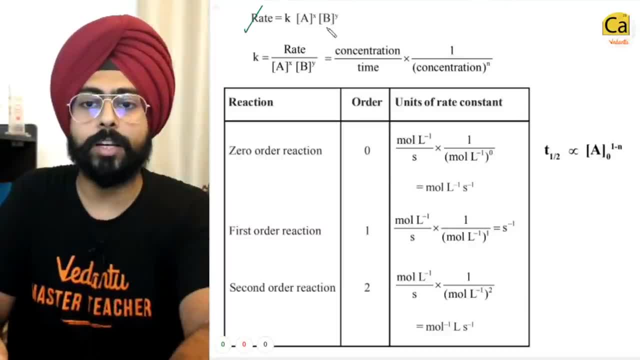 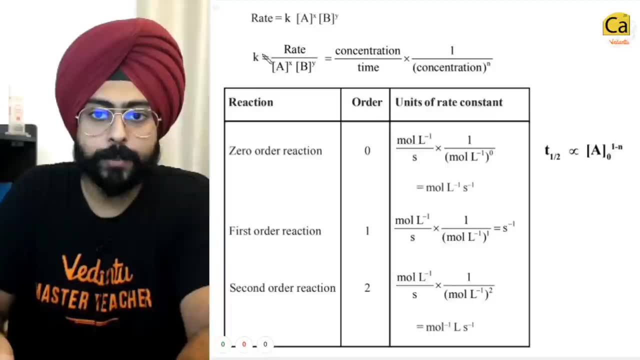 So now, my dear friends, we know that rate is equal to k times a to the power x, b to the power y, and the order can be determined by looking at the units of the rate. constant, yes, So rate is equal to rate upon Ax. By fine, so rate, kya hoga? rate is speed of the reaction. 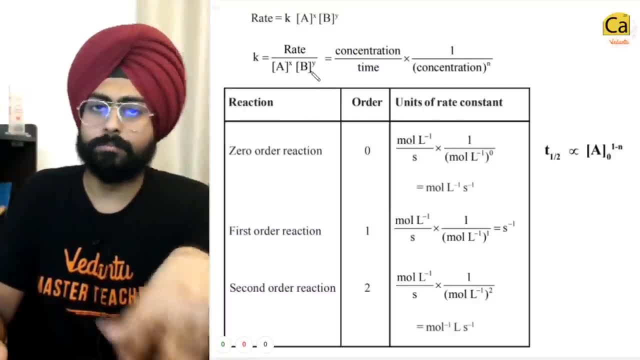 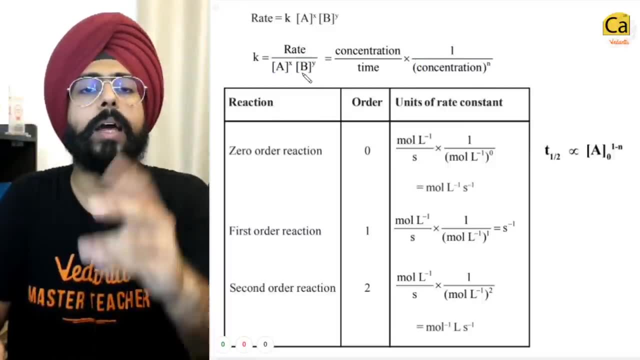 rate will be concentration upon time, as simple as that: dA by dt. concentration on time. what will be the rates of? I mean, what will be the units of Ax and By that depends on the order of the reaction. so you can say that this N over here. 1 by concentration. 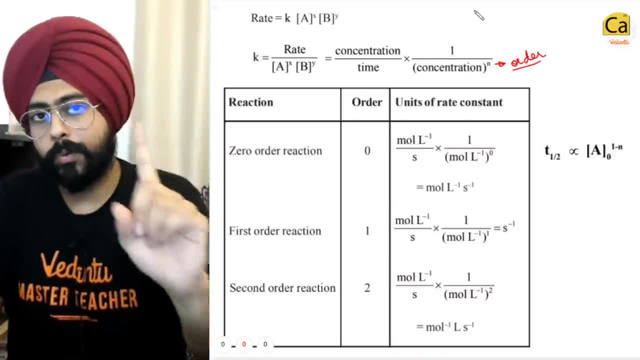 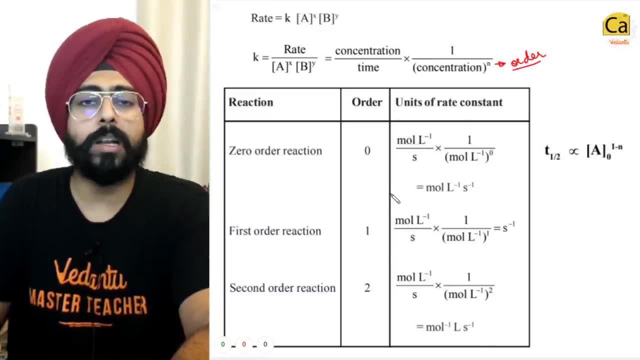 to the power N. this is the order of the reaction. so one way to determine the order of the reaction is by looking at the units of the rate constant. zeroth order reaction: mein. the rate constant units are moles per liter per second. first order reaction: mein. the units are per second. 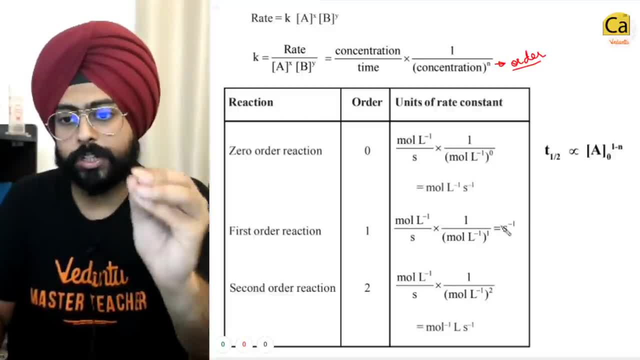 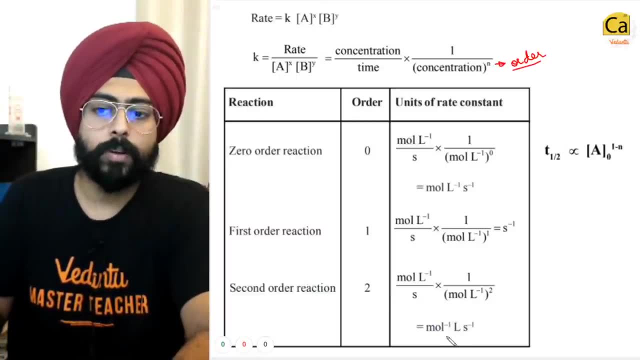 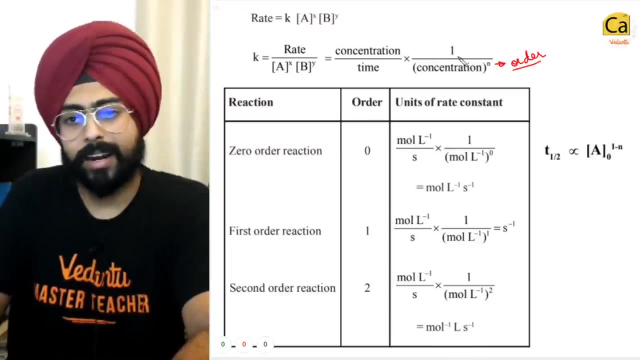 very easy to determine. okay, if it is given that the rate constant is equal to something, something per second, it's a first order reaction. second order reaction implies that the units will look like this: per mole liter per second, okay, and you can put different. 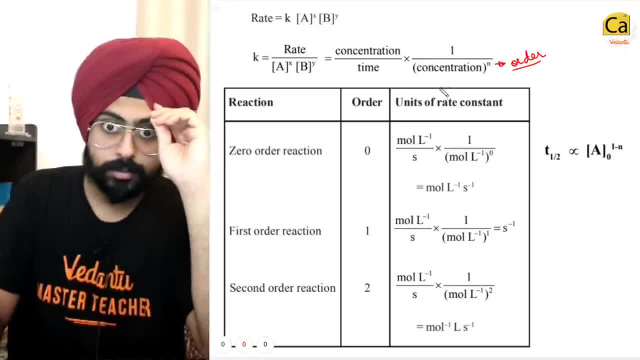 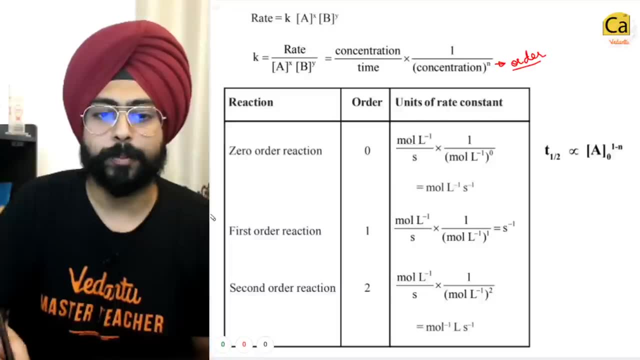 different values of N. over here too. Over here, to figure out what's the, what's the unit of the rate constant for different, different orders of the reaction. fine, very simple. Now, moving on to the zeroth order reactions: okay, tikka. zeroth order reaction: pe jaatein. 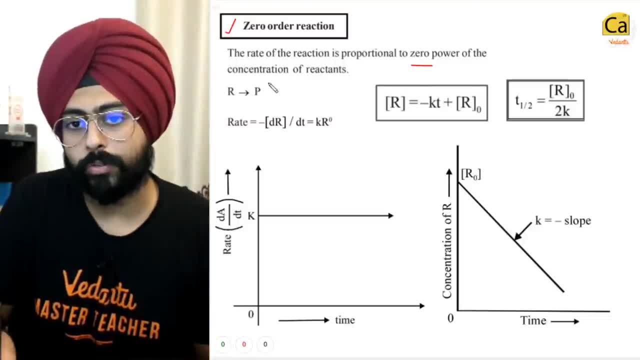 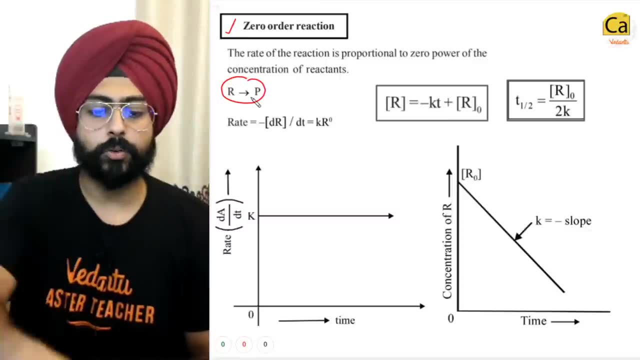 the rate of the reaction is proportional to zeroth power of the concentration of the reactants. so if you think of a very simple way of writing reactions, that is, R going to P, reactants going to products, I can write: rate is equal to minus dR by dt. 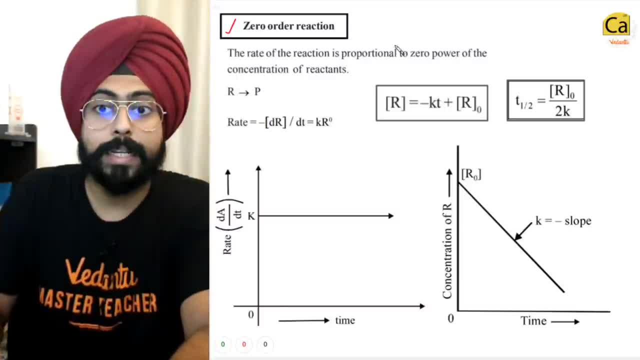 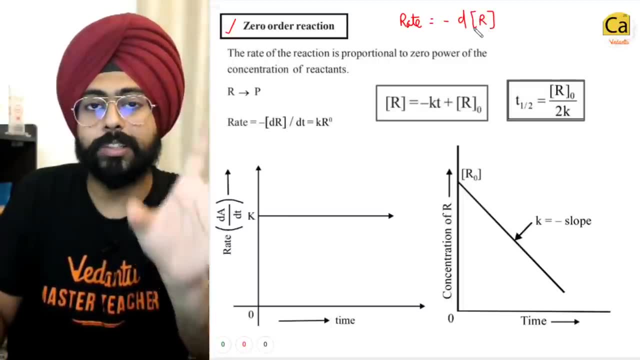 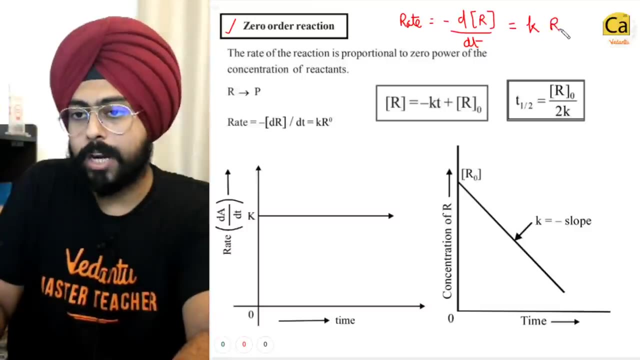 Why is there a minus sign, people? Because reactants will be decreasing. okay, so rate is equal to minus dR. what is R? R is the concentration of the reactant at any point upon dt. this is equal to rate constant k into R to the power: zero. okay, theek hai toh yahan pe kya aa gaya R to the power. 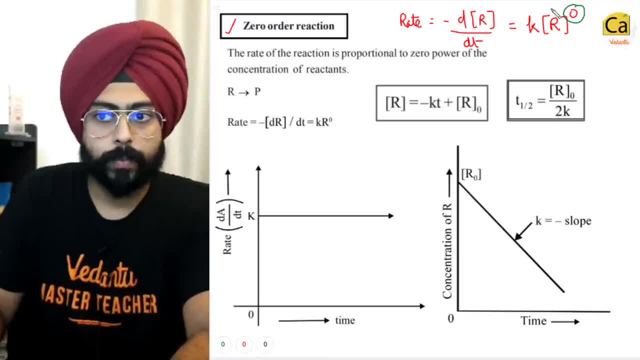 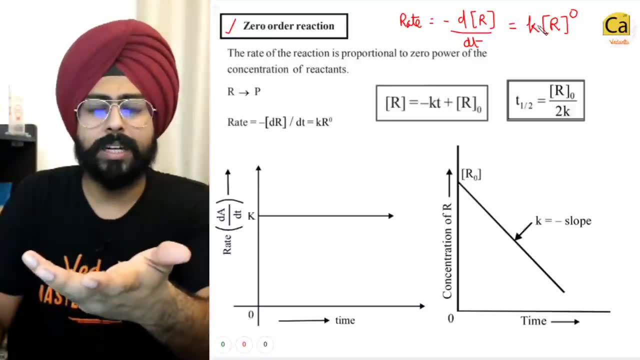 zero aa gaya. this zero is the order of the reaction, okay. R is the concentration of the reactants and zero is the order of the reaction. Now, once you do integration on it, okay, you know how to do the integration, isn't it? 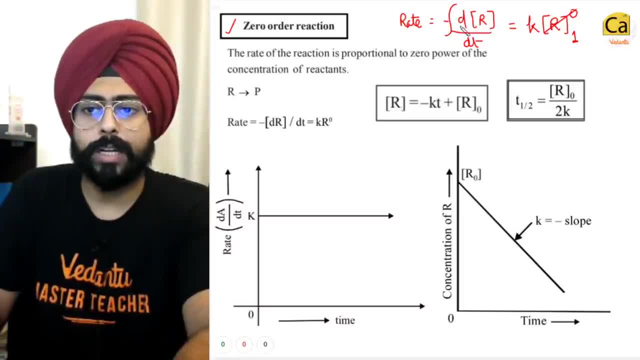 R to the power zero is just equal to one. so integrate both sides. you will get R equals to kT, plus integration constant. once you solve for the integration constant, we are not going to the derivation- you get this rate law. okay, this is the equation that 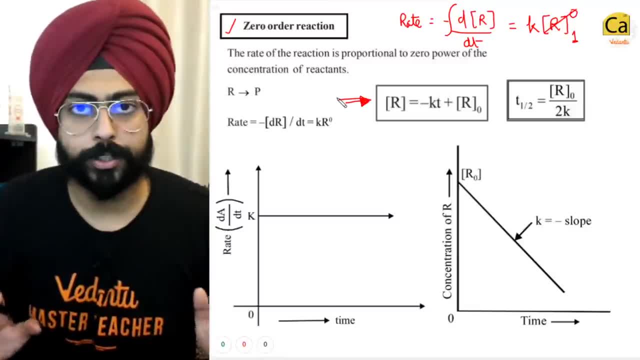 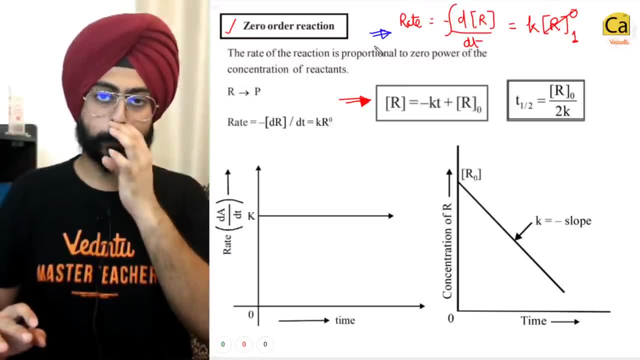 you get for zeroth order reactions. you do not need to remember this equation. this equation can quickly be derived. You can derive any time you want using the basic rate law. that's the good thing about chemical kinetics: that you do not need to remember anything. but if you remember, then 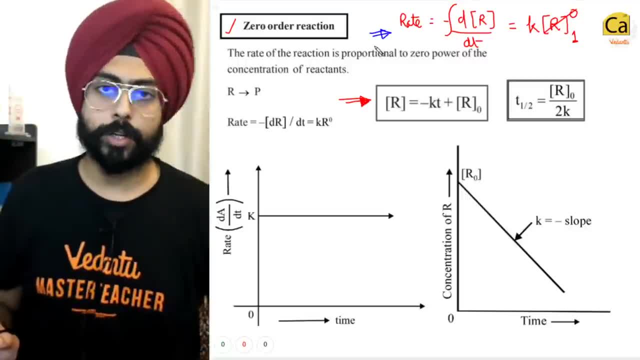 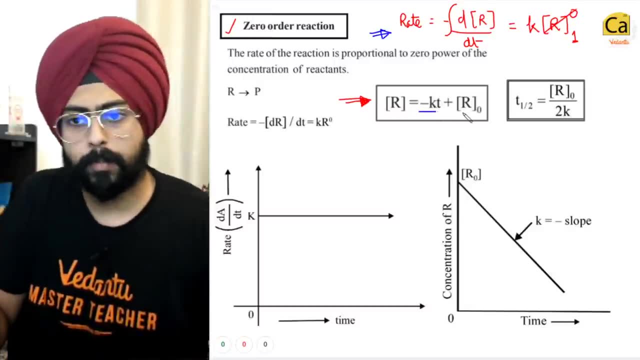 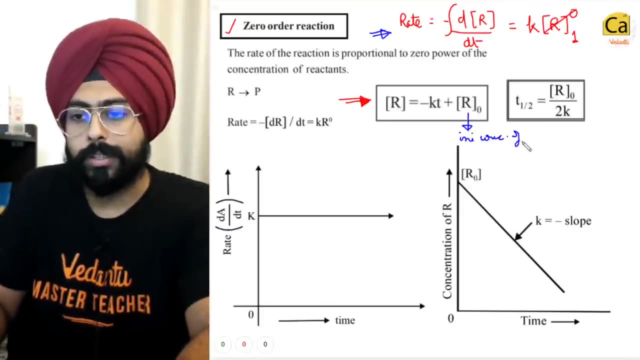 you will save anywhere around 2 to 3 minutes every question of chemical kinetics. if you don't remember, you will have to derive everything. yeah, so R is equal to minus kT plus R0, what is this R0?? R0 is the initial concentration of the reactant. as simple as that. 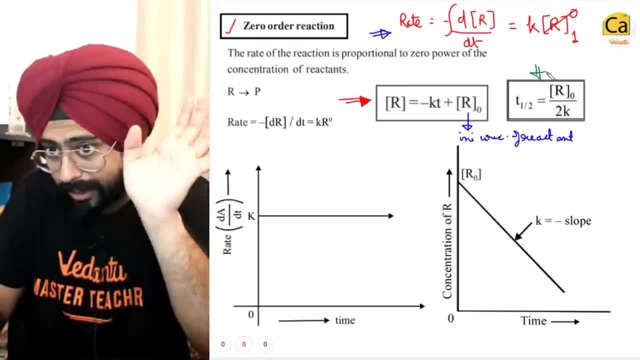 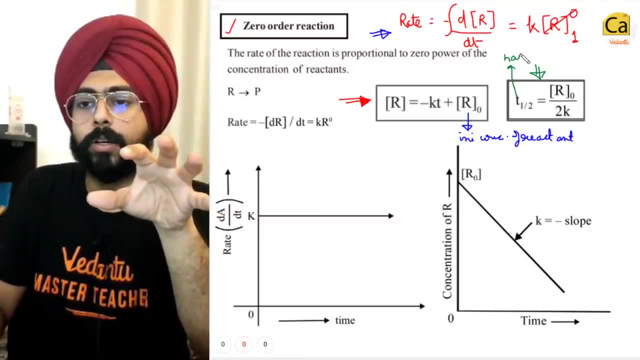 This chapter is mathematics, not chemistry. Now, what I have written over here is T half. can you tell me what T half is? in the chat box, T half is known as the half-life. okay, T half is known as the half-life of any reaction. 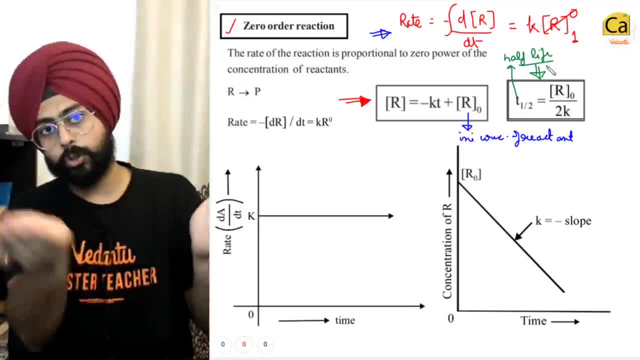 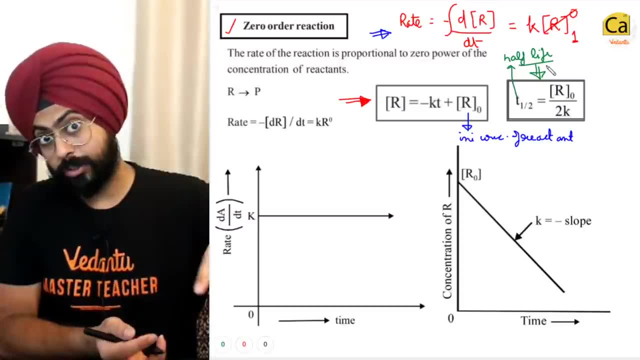 what is half-life? Half-life is where the concentration of the reactants has reduced to half the initial value. okay, so two half-lives, one-fourth of the initial value. three half-lives, one-eighth of the initial value. four half-lives, one-sixteen of the initial value. yeah, initial ka half. 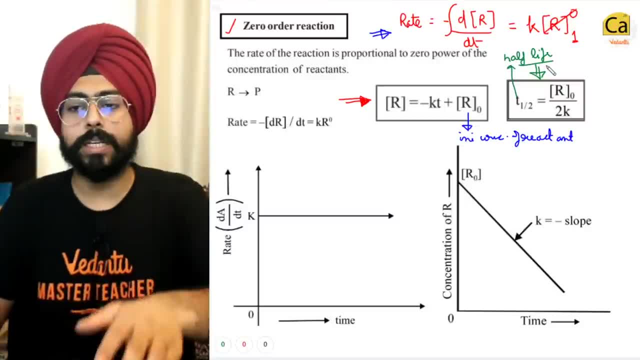 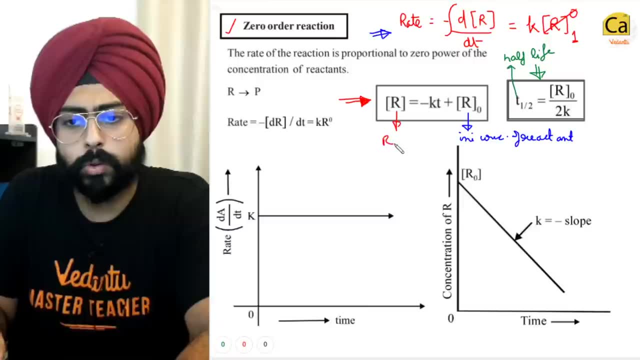 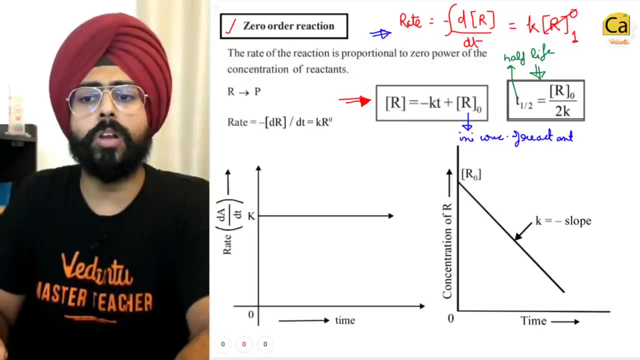 half, half, half. That is your T half. and how would you calculate it? Very easy: just put R equals to R0 by 2 and then you can calculate T. yeah, So calculating the formula for half-life is also very easy. in case you do not want to, 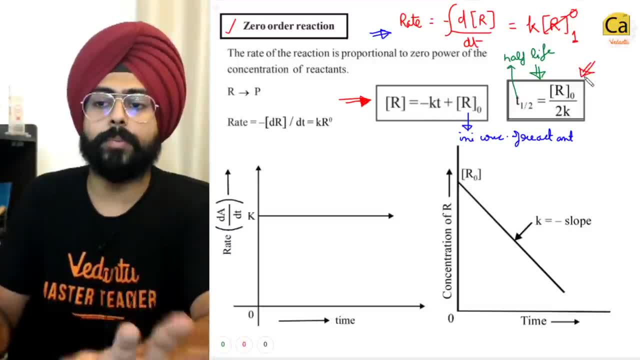 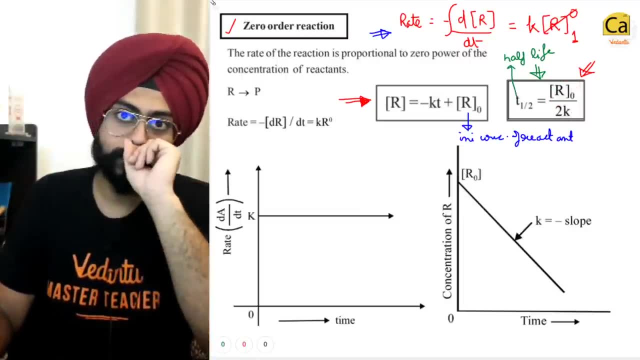 remember it, it's your choice entirely. for zeroth order reactions it looks something like this: R0 by 2k, initial concentration of the reactant upon two times the rate, constant Fine, very simple. Then comes the first order reaction. now, first order reactions are very important for us. 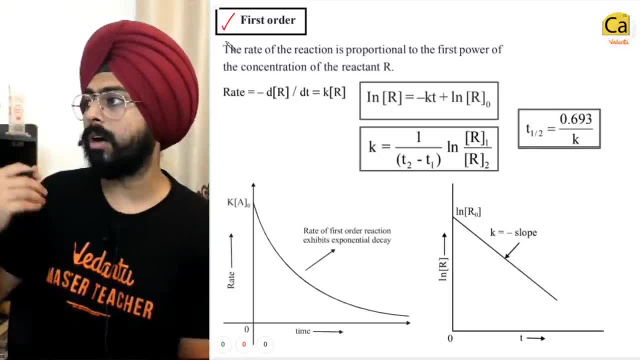 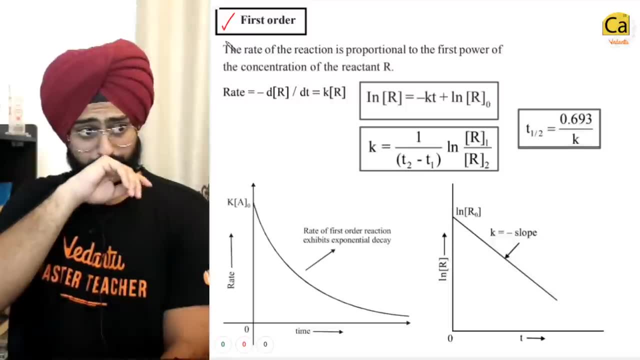 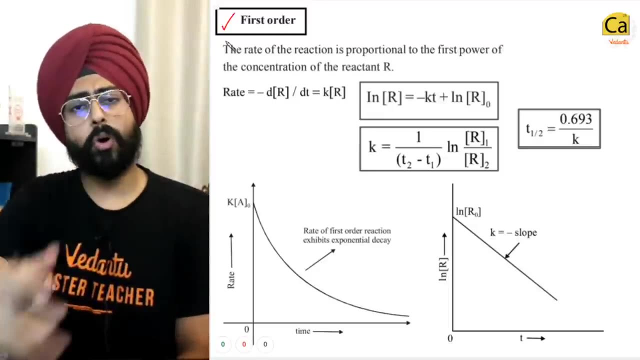 why so? Because first order reactions are found in abundance in nature: Nuclear reactions, nuclear decay. it's first order reaction. okay, so if you understand, if you understand first order reactions, you automatically will be able to do all the questions of nuclear decay that are there in physics and sometimes in chemistry. 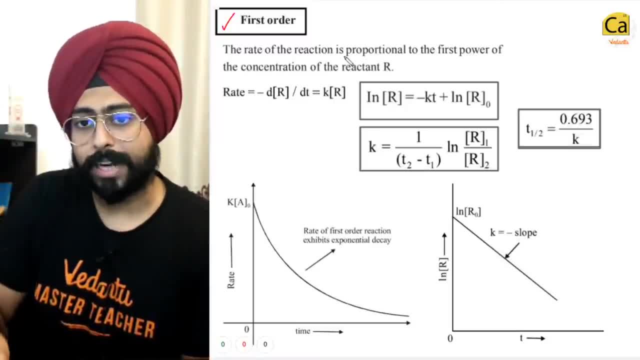 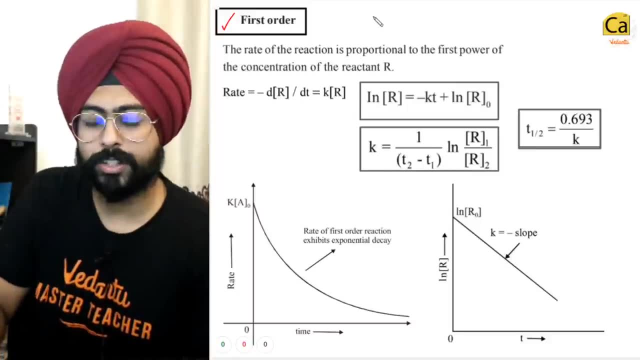 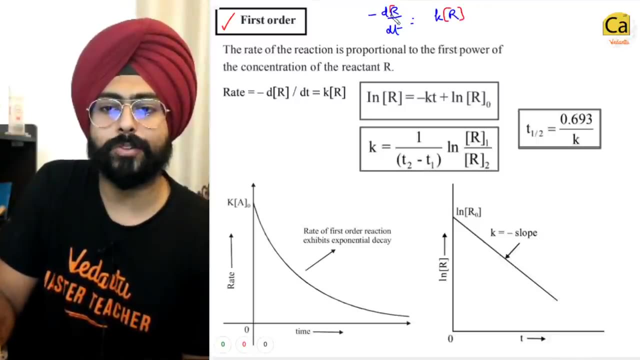 So rate of the reaction is proportional to the first power of the concentration of the reactant: R. okay, first power. So what does this mean? That minus dr by dt is equal to k times R. you can put brackets over here Now. you just have to do integration on the left hand side. you will have minus dr by R. 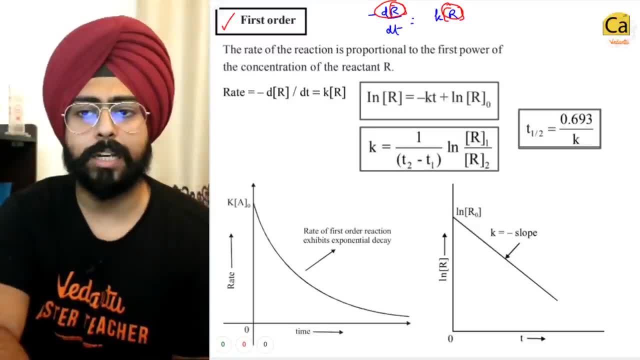 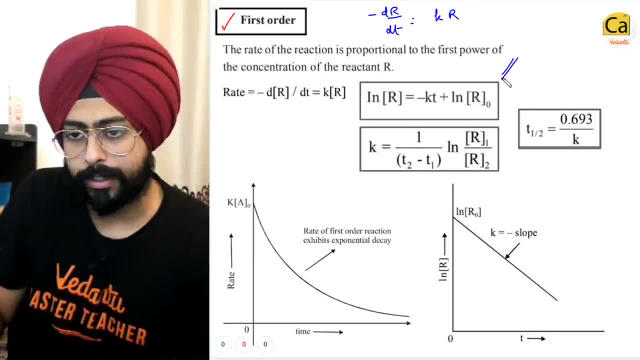 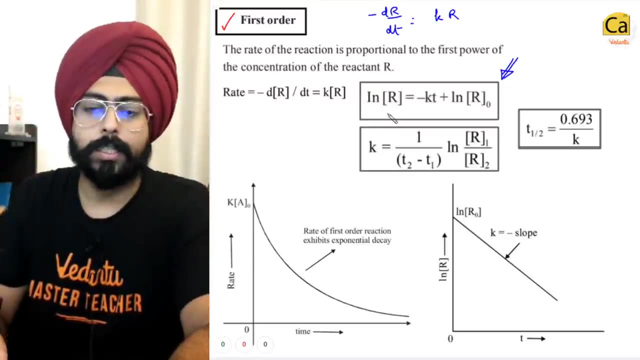 on the right hand side, you will have kdt, so it becomes: ln R equals to minus kT plus integration constant. When you solve for the integration constant, you get this. you get ln R. okay, this is ln ln natural log. okay, ln R is equal to minus kT plus ln R0,. okay. 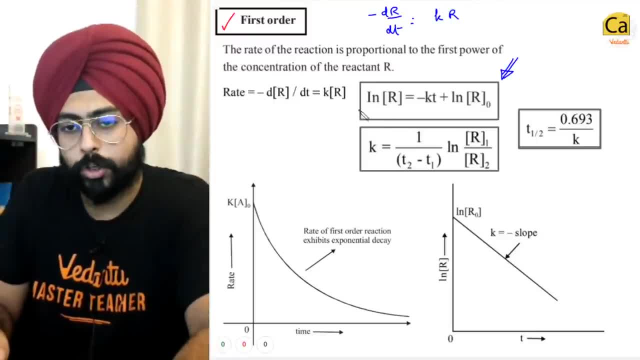 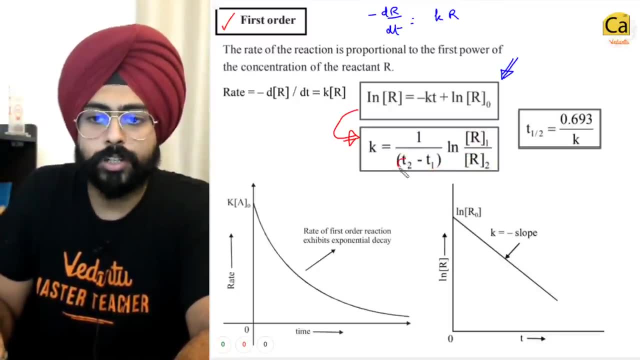 You can manipulate this equation. okay, you can manipulate this equation to get a formula for k. If R1 is the concentration at T1 and R2 is the concentration at T2 of the reactant, then this is the formula for the rate constant. 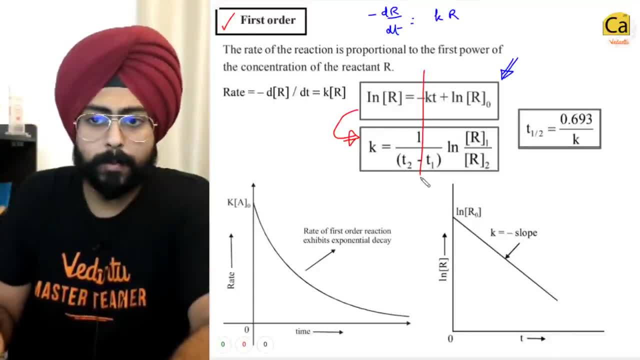 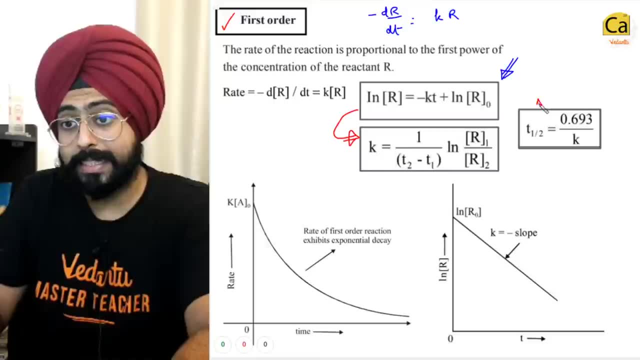 It is very easy. yeah, You don't need to remember all of these formulae once again, because you can derive them from scratch. Also, look at T1, T2, this is something that you should remember because T1's questions from first order reaction are in plenty okay. 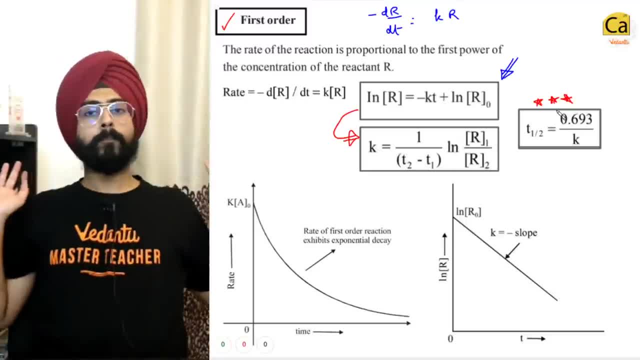 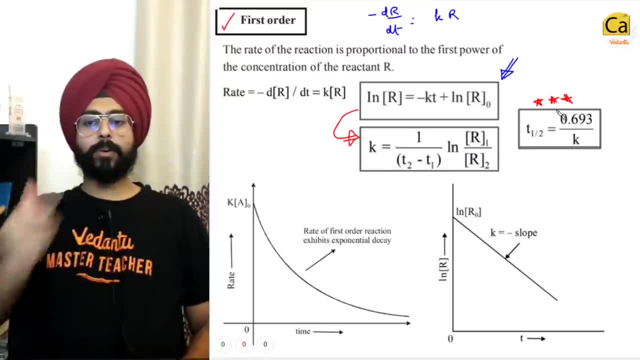 T1 for a first order reaction is equal to 0.693 by k. as simple as that, yeah, as simple as that. okay, It becomes very simple. Okay, Because you know there is a ln over here. so if you put this as R0 by 2, ln, R0 by 2. 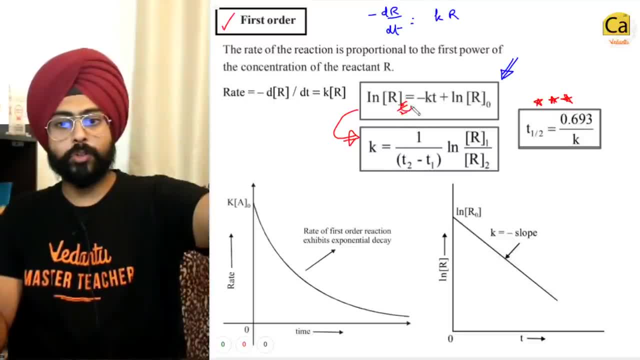 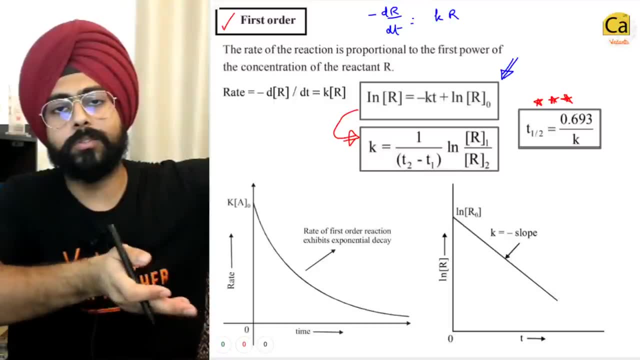 minus ln R0, both will be cut. yes, because you can bring 2 away. yeah, You can write it as ln R0 minus ln 2 minus ln R0, ln R0, ln R0 will get cancelled, So you will get T1, independent of the initial concentration. 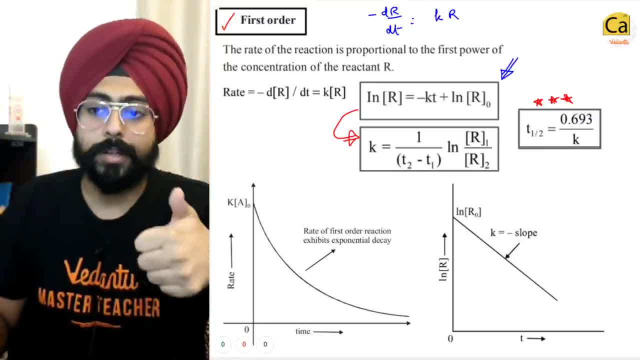 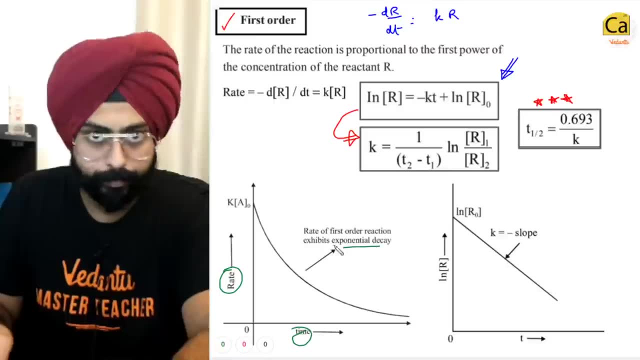 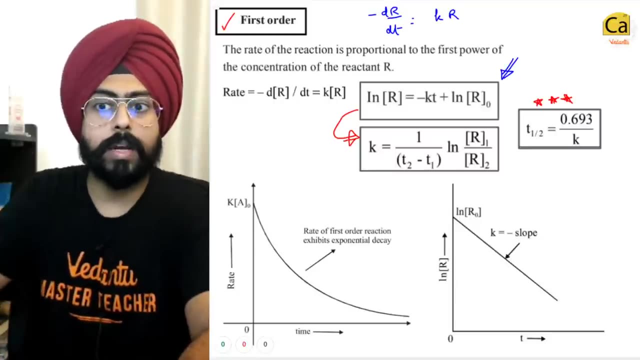 That's the best thing about the first order reactions. T1 is independent of the initial concentration. okay, So Rate versus time is an exponential decay. okay, Rate versus time exhibits an exponential decay because R is reducing at an exponential rate. yes, 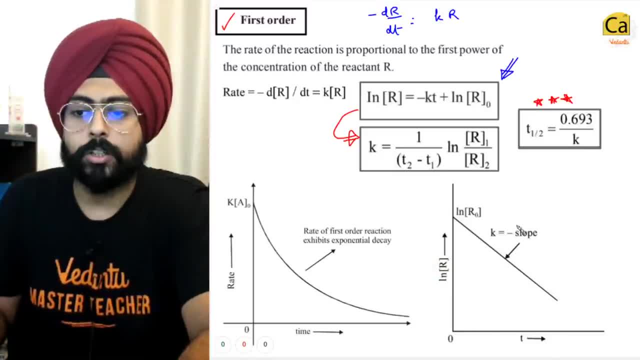 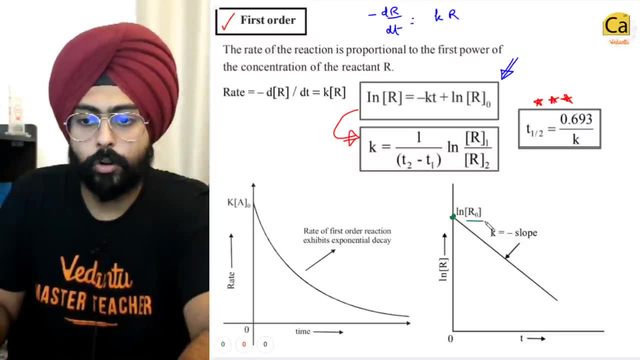 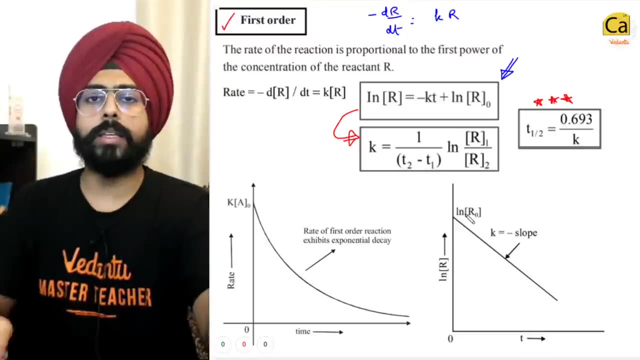 And if you take the slope of ln R with T, the slope is equal to minus of k. okay, fine, This is the initial amount: ln R0, and this will be a straight line. Very simple ideas. You can anytime pause the video if you want and look at these graphs. 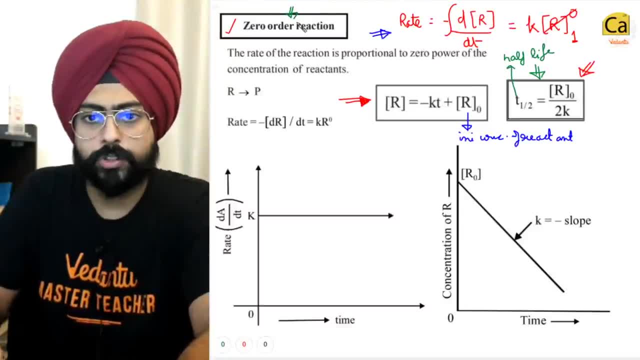 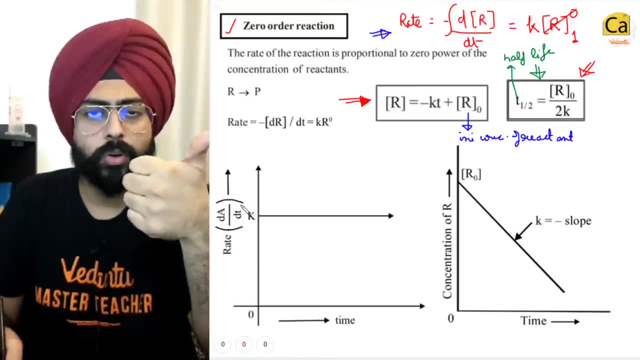 Okay, In more detail. okay, Similarly, we will go back to the graph. so zero order reaction. see, It is independent of the yeah. rate is just a constant value. rate is just a constant value. k it is independent of anything else. so rate is just a constant value depending. 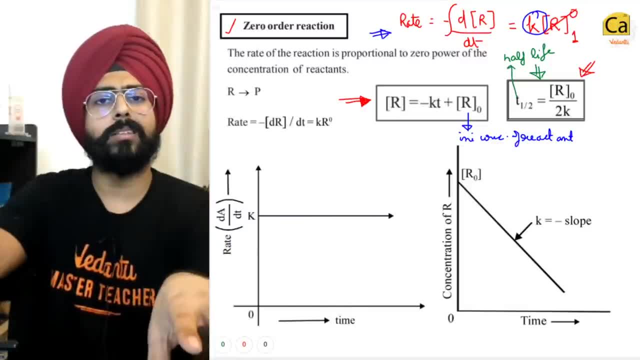 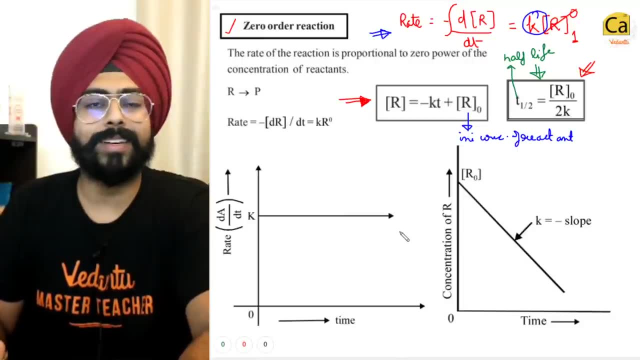 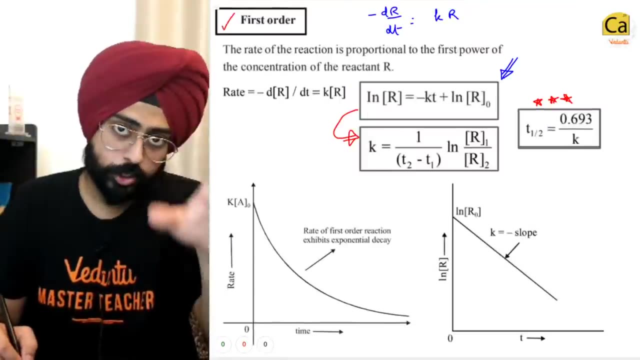 on time. yeah, Rate versus time: constant value, the same rate. it won't change ever. and R0 will decrease linearly with time, with the slope of minus k. as simple as that, okay. So first order and zeroth order are important. 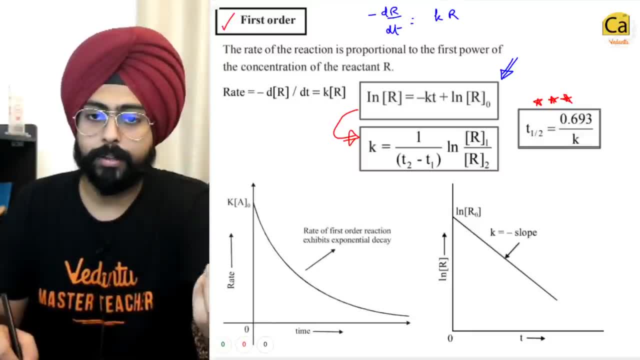 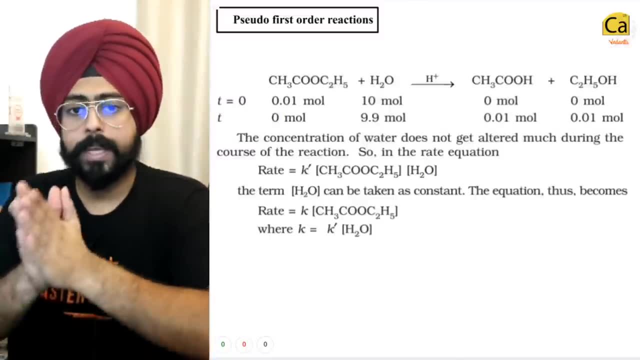 You can do the derivations on your own after today's class to revise them better. You can do them for second order as well. you can do them for nth order as well, but first and zeroth order are the most important, okay. 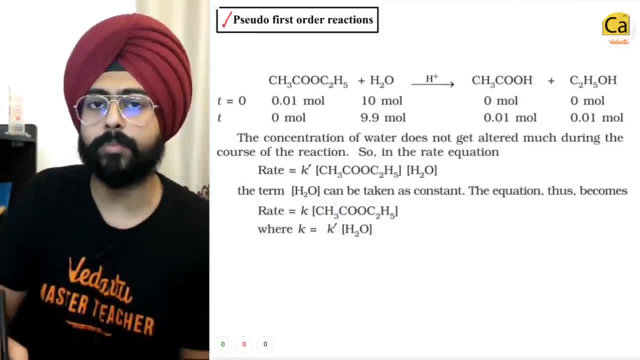 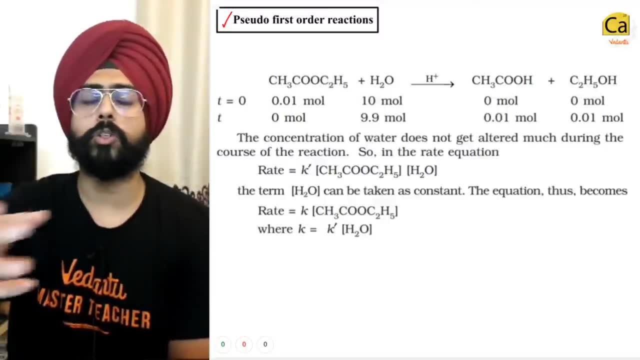 Then you have pseudo first order reactions. Now, these are really, really important for us, because these are where the questions get formed out of, and these type of reactions happen in nature in abundance. bohot sare reaction. hote hai nature mein. So what's happening is: 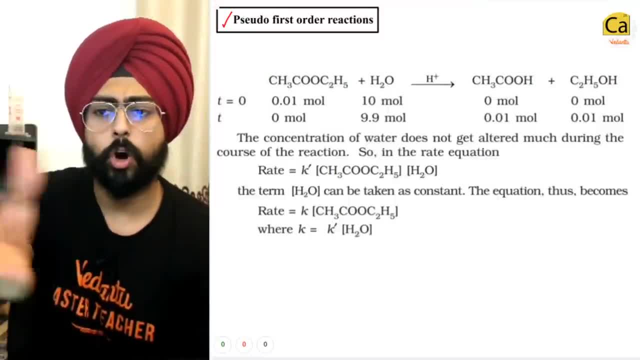 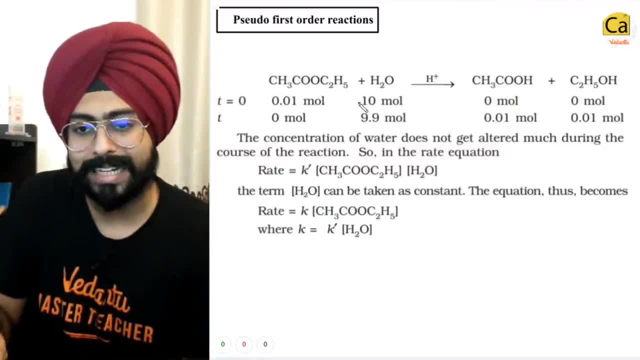 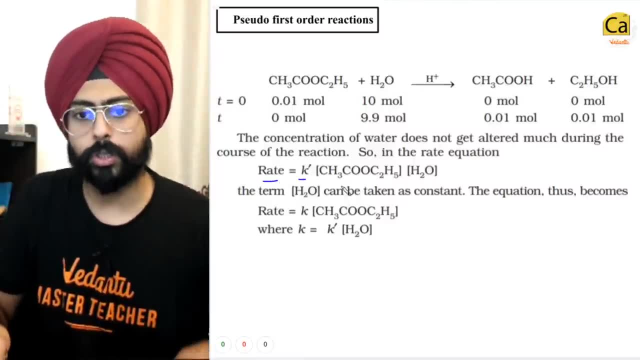 What happens is that in this case the concentration of water decreases, very less minuscule decrease in the concentration of water. So in the rate law, if rate law is equal to k dash times CS3COOC2H5 into H2O, my dear, 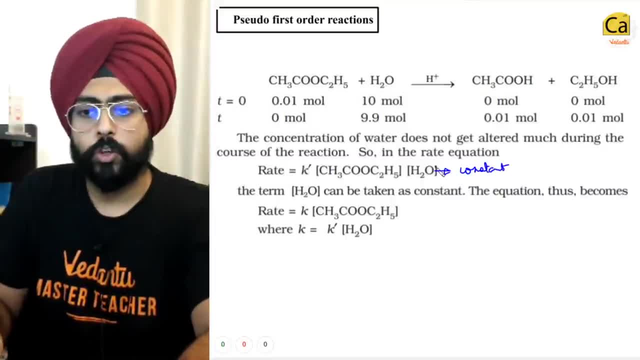 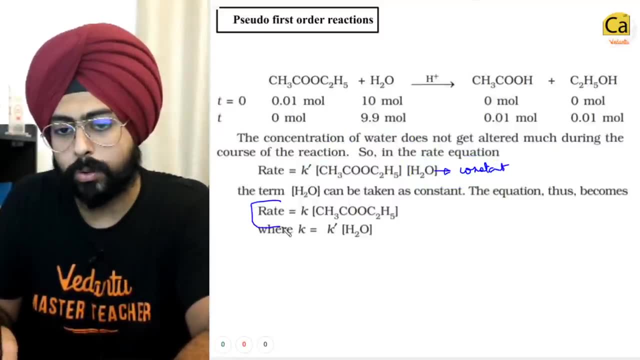 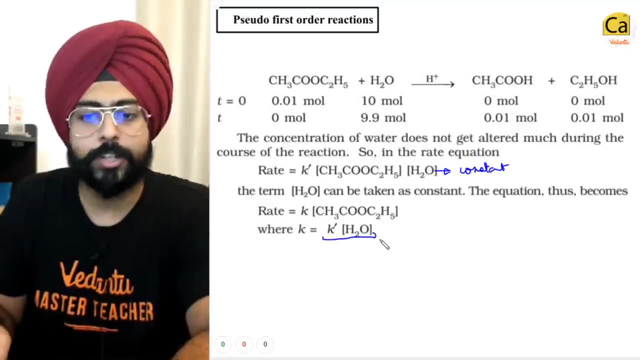 friends, do you realize that this idea is also constant? So why don't we club this with k dash And then get the final rate law, which is equal to rate, equals to k times just the concentration of the ester, where your new k is equal to k dash times H2O's concentration? 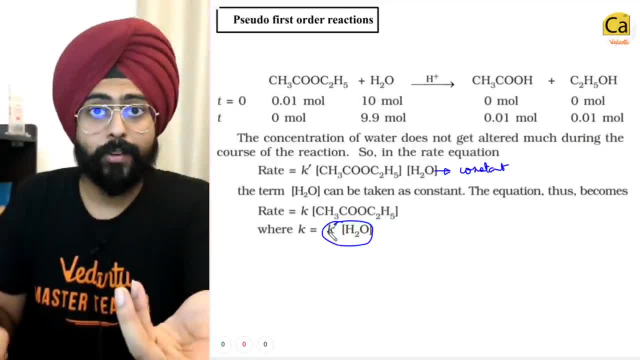 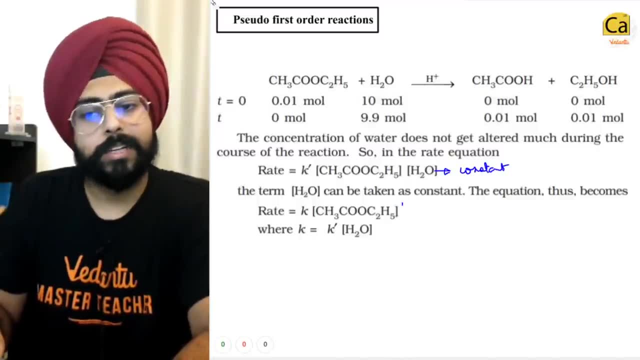 So this is the new rate constant. now, fine, And this absolutely is a first order reaction reactant to the power 1, first order reaction. So all the analysis that we did over here can be applied to questions of this reaction as well. 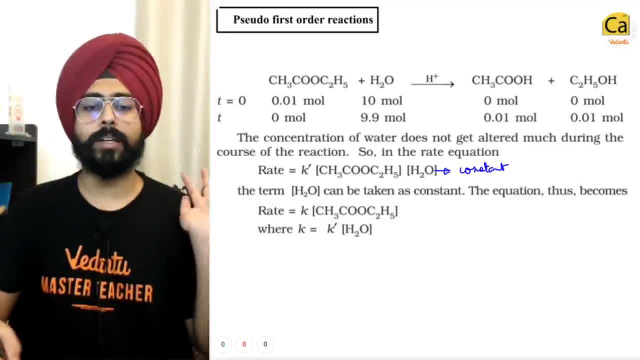 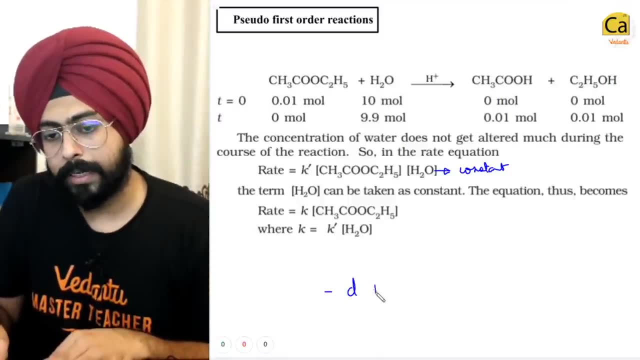 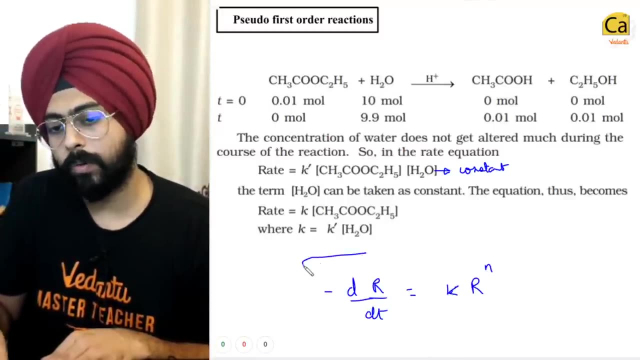 This was about rate law, how to manipulate it. all you need to do is just keep in your mind this equation. you have to remember. this equation minus dr by dt is equal to k into r to the power n. that's all. 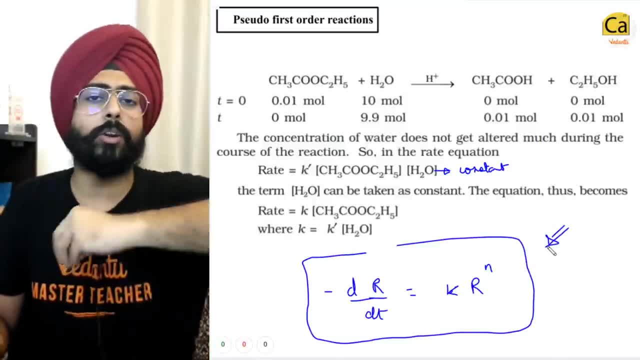 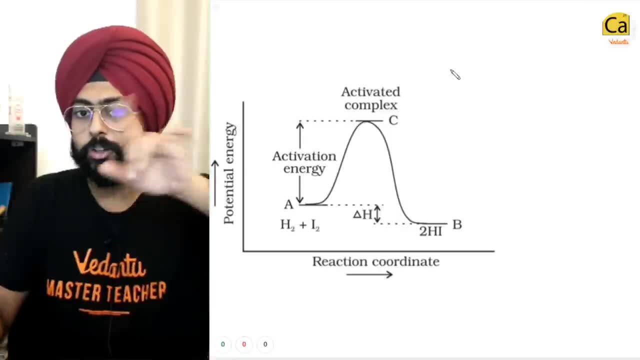 Do integration differentiation on this guy and you can get the rate law for any order whatsoever- Order rate law done. Now let us go into the energetics. yes, So this is a graph. Yes, This is very important. 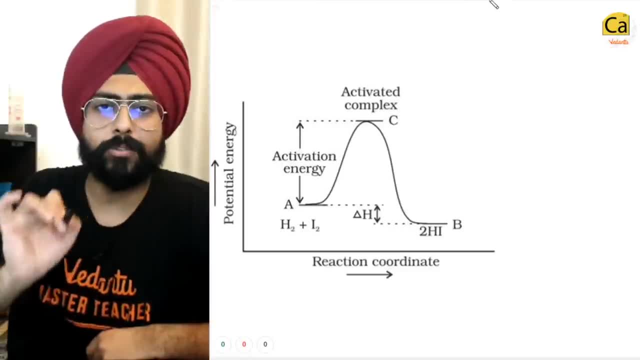 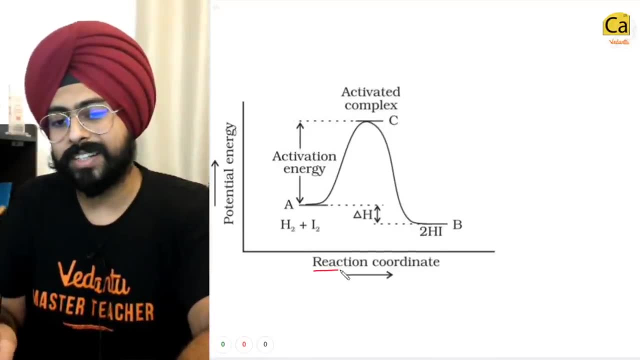 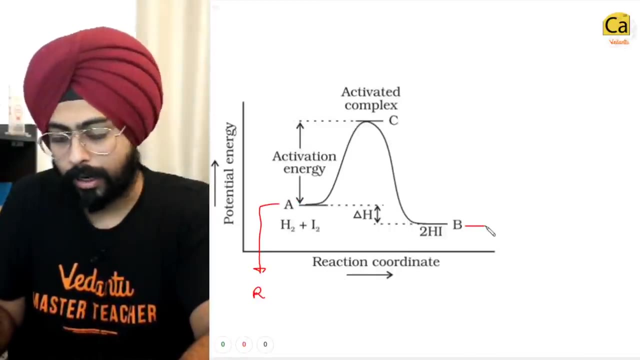 It comes time and again in organic chemistry as well, and this is the easiest graph to understand in chemistry. What is it telling us about? It is telling about the potential energy of a reaction versus the reaction coordinate: A- over here are the reactants and B- over here are the products. very easy, yeah. 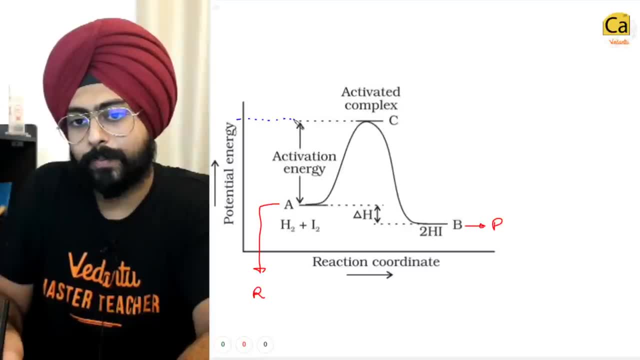 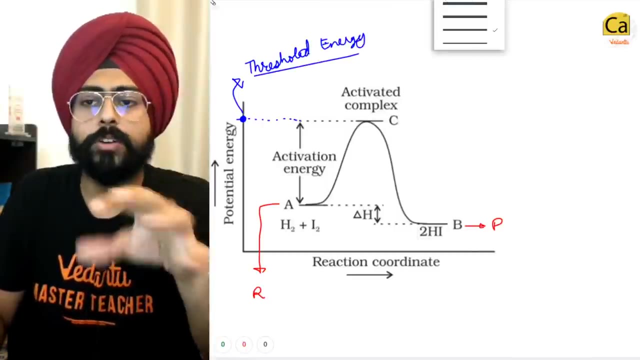 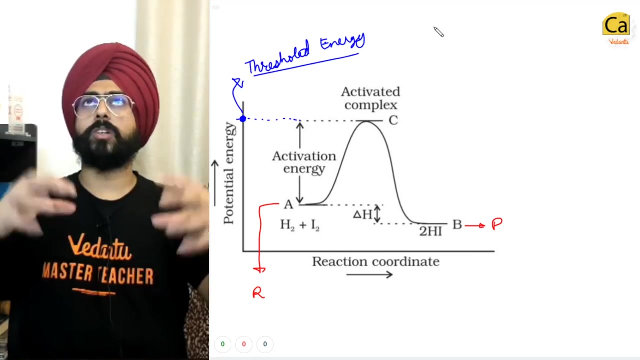 Now, my dear friends, this energy that is here, okay, this amount of energy that is here, is known as the threshold energy. okay, threshold energy. This is the minimum energy required for the reaction to happen. What happens is think about it. reactants are there in the reaction mixture. 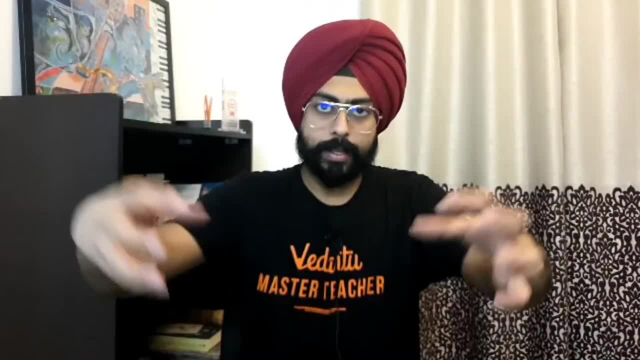 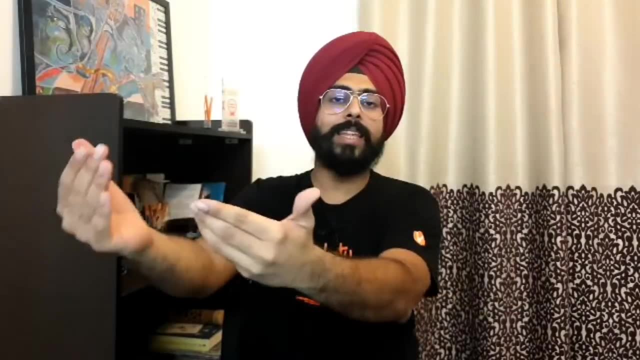 You might assume a gas, you might assume a solution. okay, So now, when they are reacting with each other, they have to collide with each other. yeah, Now the collisions, if they happen with a certain force, only then they will be able. 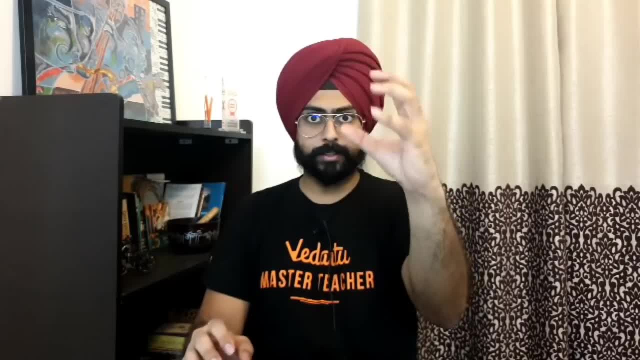 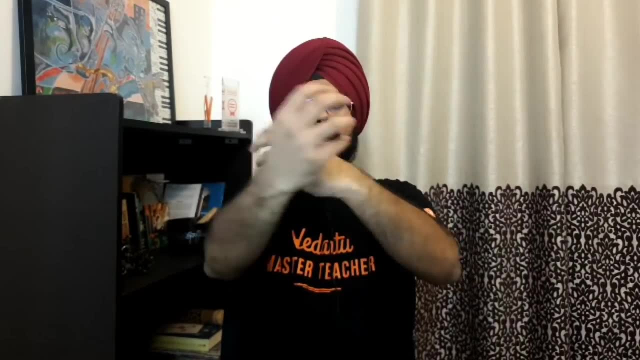 to go to the products. Okay, Okay, Okay, Yes, fine, so let's say: this is one reactant, this is one reactant. they have to collide with each other. So they can be colliding with each other in different, different manners. yes, 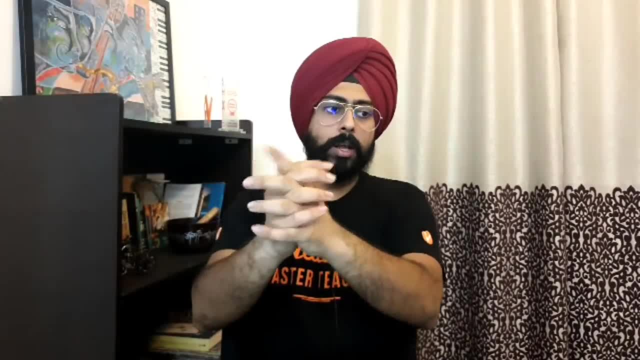 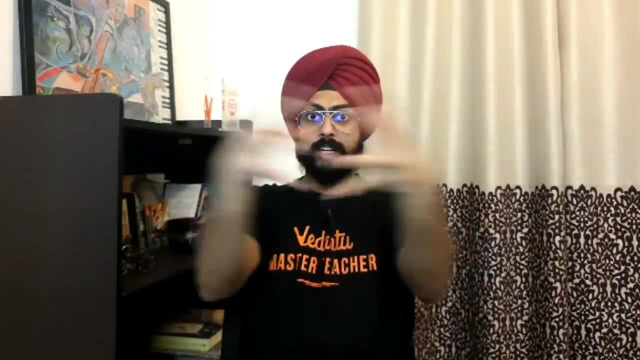 Only when they collide in this direction they can form a product. But let's say, their velocities are not enough, their energies are not enough. no collision, no good collision, no good collision. but only if they have enough energy, good collision. 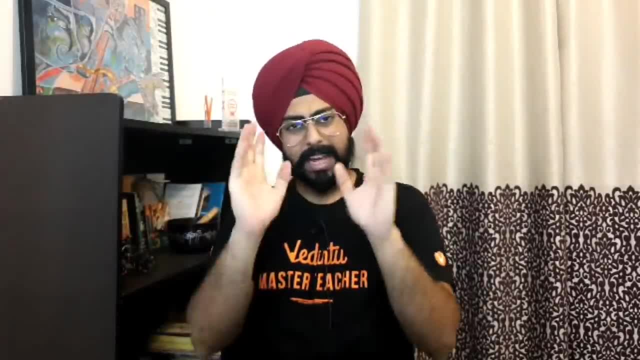 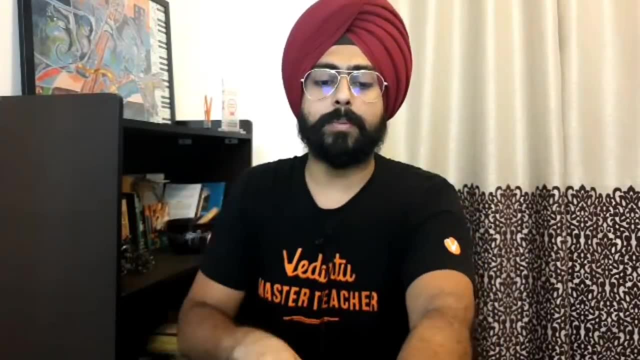 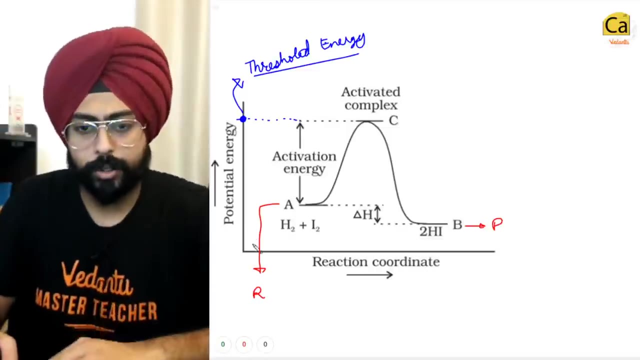 and then they can form the product. okay, fine, Everyone understands this basic logic behind reactions, how things are colliding with each other. okay, So now let's get back to the board, or let's understand this fine Threshold: energy is the minimum energy required, so this value over here is known as your threshold. 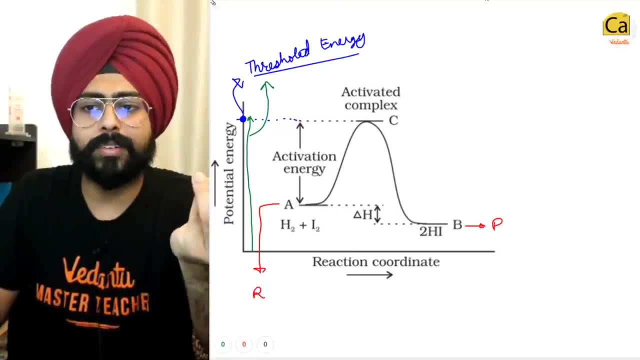 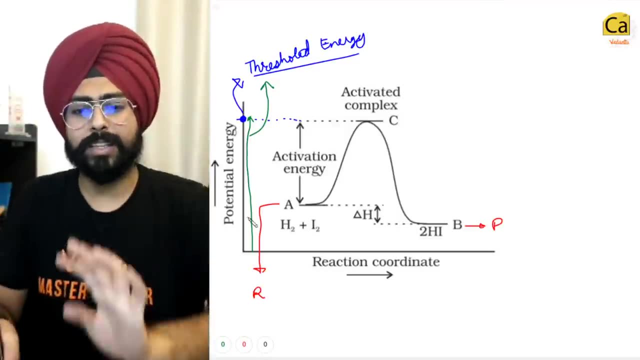 energy Now, since you have energy already existing, because there is a lot of temperature. if it was absolute zero, there would be zero energy by default. By default, there is some amount of energy. see, this is the potential energy of the reactants, to begin with. 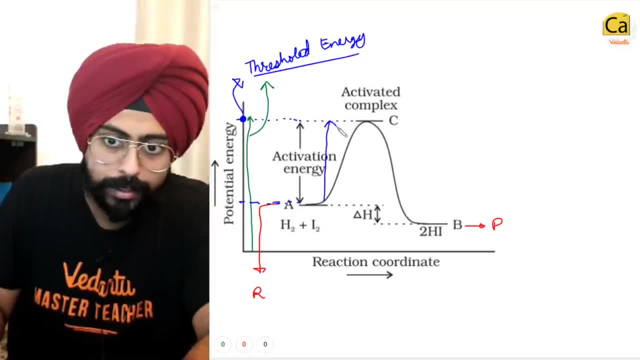 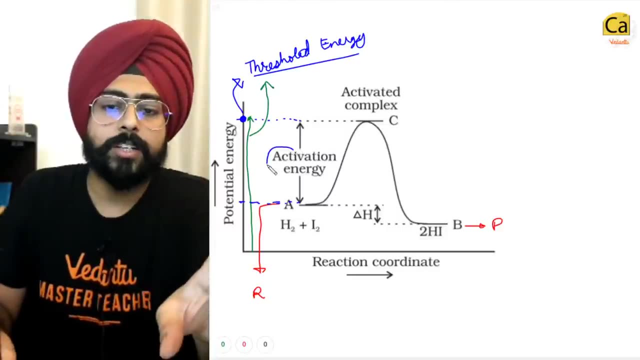 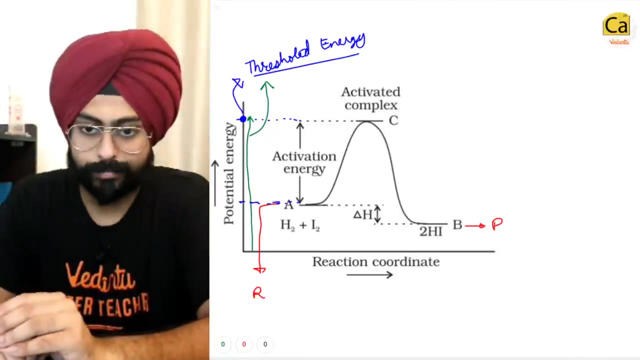 So if you have to take them to the reactor, To the threshold energy, you have to provide them some more energy, and that energy is known as activation energy. Every reaction in nature needs some activation energy. sometimes it is provided by the ambient temperature itself. sometimes you have to heat it or shake it or etc. etc. yeah, 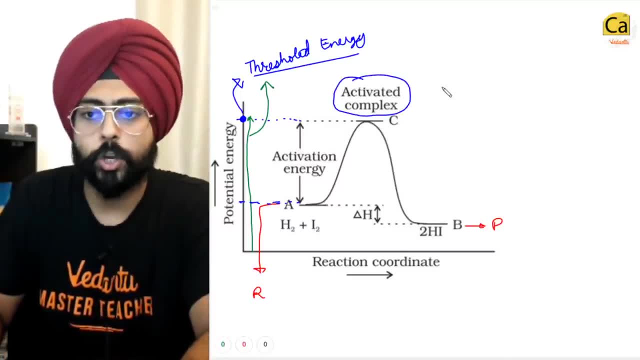 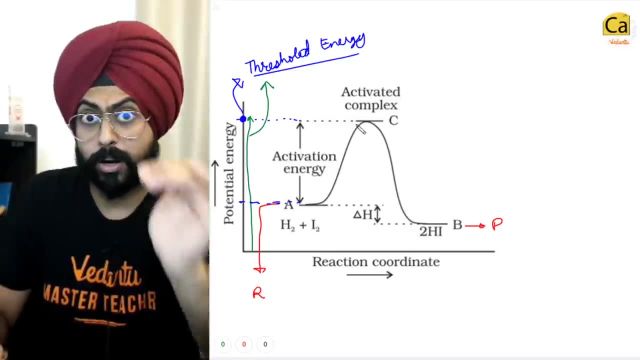 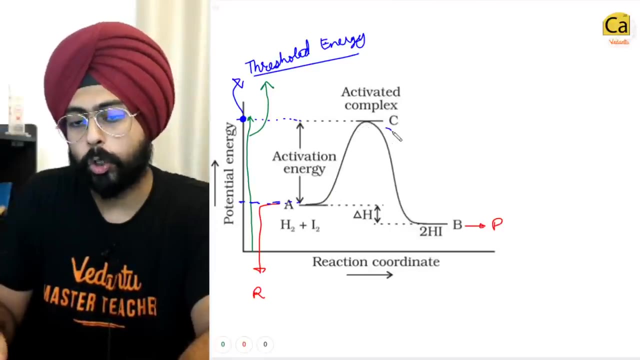 So this is the activation energy and then you reach the activated complex, also known as the transition state, remember from organic chemistry. So activated complex is the most unstable part of the system. This is your unstable equilibrium. From this unstable equilibrium you can go back to the reactants or you can go forward. 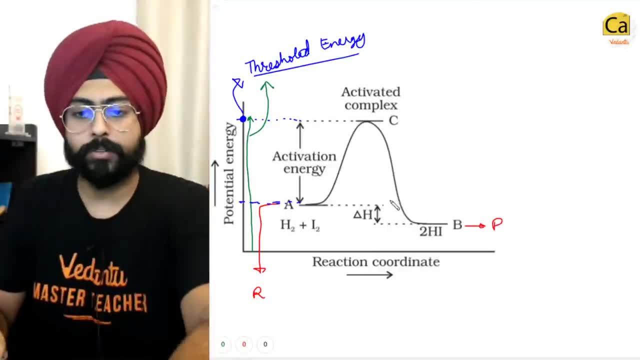 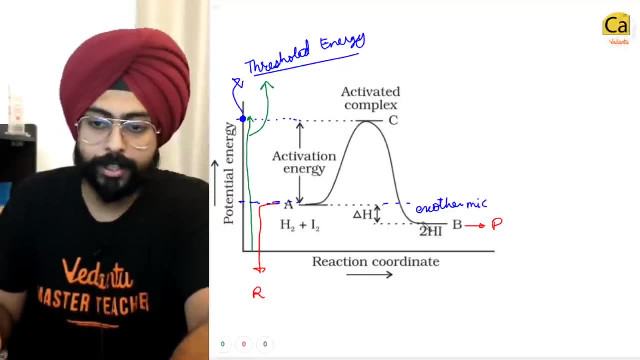 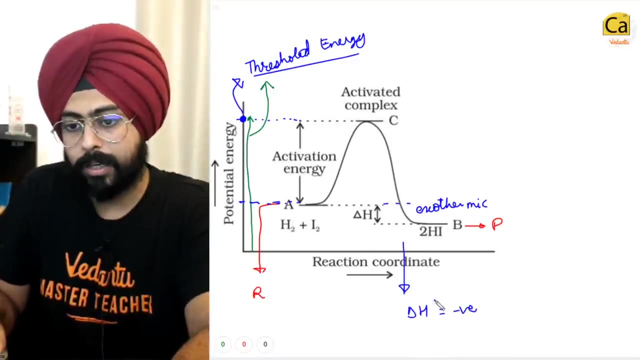 towards the products. This diagram that we have drawn shows an exothermic reaction, because the energy, the potential energy, of the products is less than that of the reactants. So over here, in this particular reaction, delta H is going to be negative. 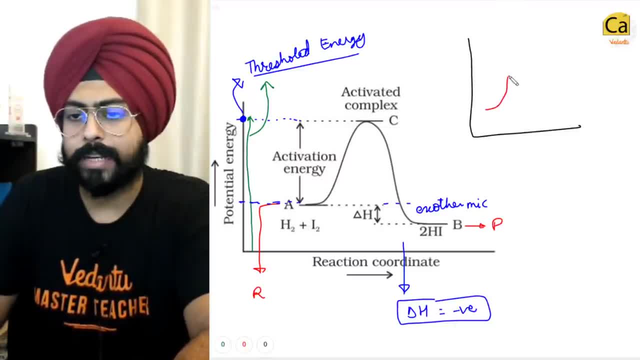 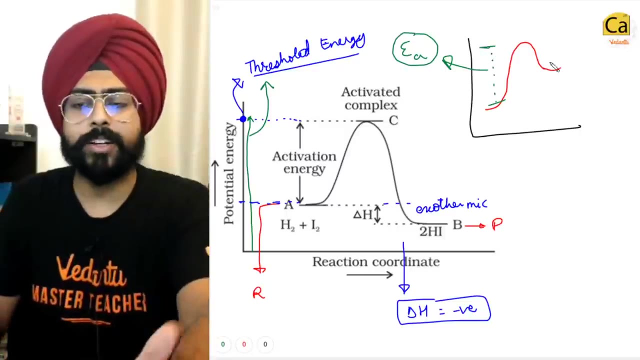 There could be delta H equals to positive as well. You could have a reaction diagram that looks like this: Once you reach the unstable equilibrium, once you provided the activation energy- I will write it as Ea- Ea means energy of activation- Once you provided the energy of activation, it can form a product that is more unstable. 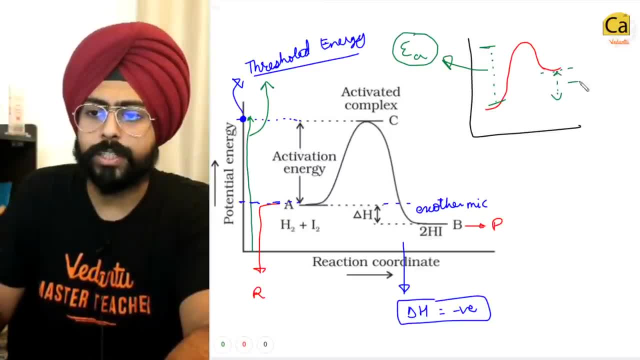 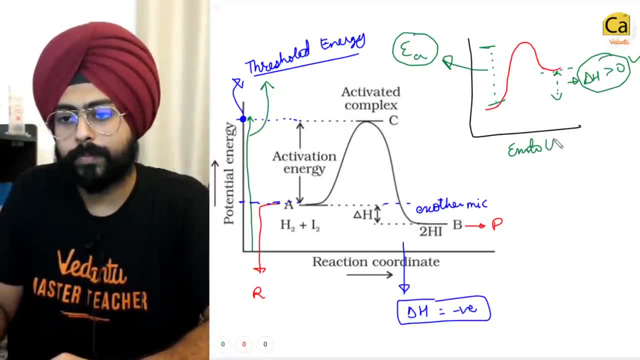 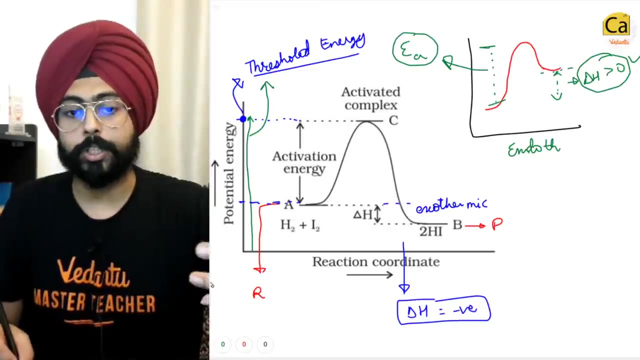 than the reactants. So over here, this value of energy will be your delta H, and this is greater than zero. This is for the endothermic reaction. as simple as that. Now, more details of this graph And how the rate varies with temperature is given by the Arrhenius equation. 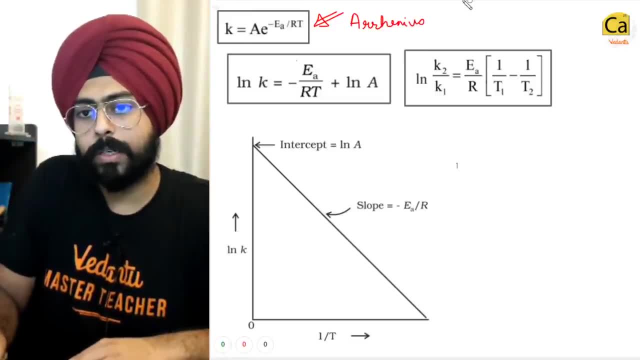 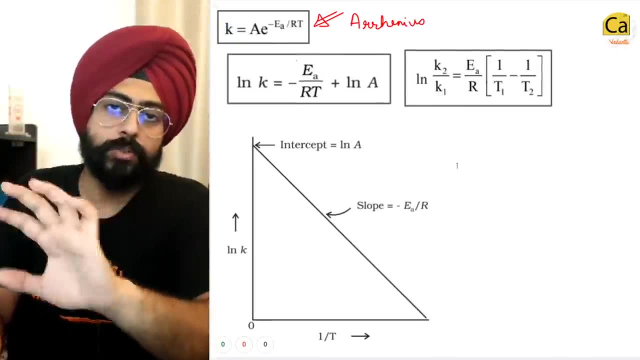 Remember Arrhenius equation, Very simple equation. So in the Arrhenius equation k is equal to A. It is the Arrhenius constant. It depends on the reaction. It is different for different reactions And in the few next pages I will try to separate this into two different terms. 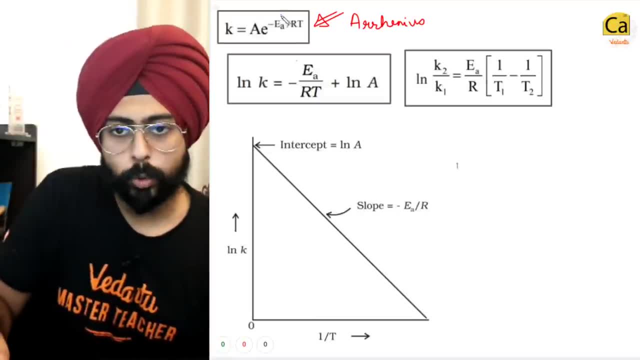 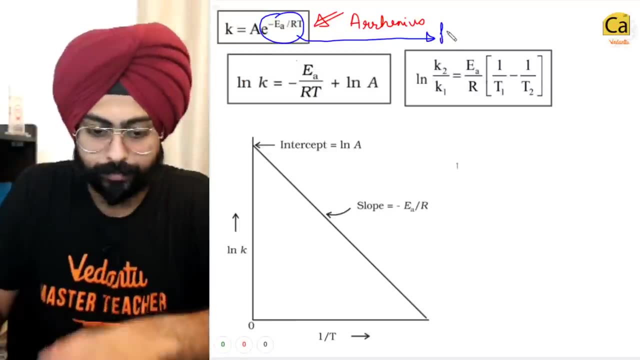 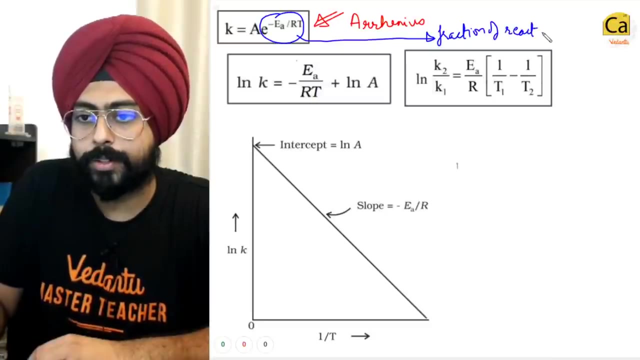 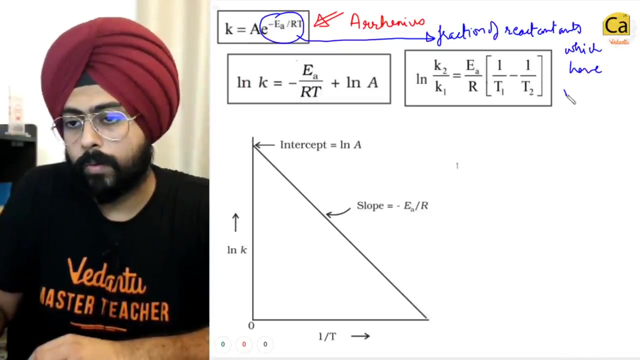 Pretty sure you remember what I mean: A into e to the power minus ca by RT. What does this mean? See, this term is accounting for. this term is accounting for the fraction of reactants, I would say, which have activation energy or more fine. 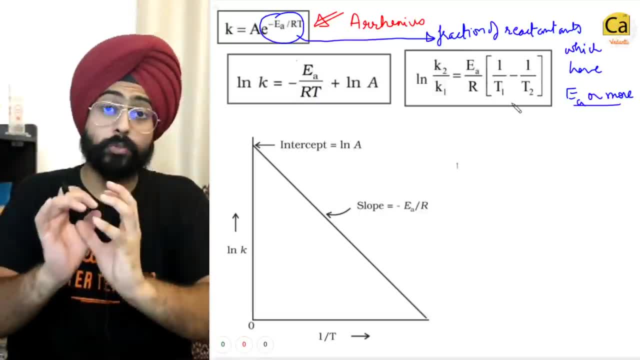 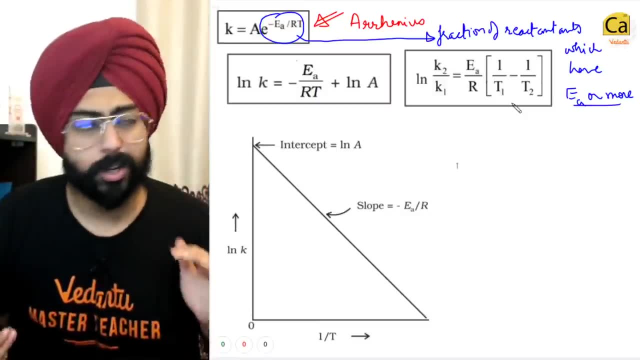 So this is accounting for the reactants which already have the amount of energy required for the reaction. This e to the power minus ca by RT comes from Maxwell-Boltzmann distribution. don't need to know why and how it comes from that distribution. 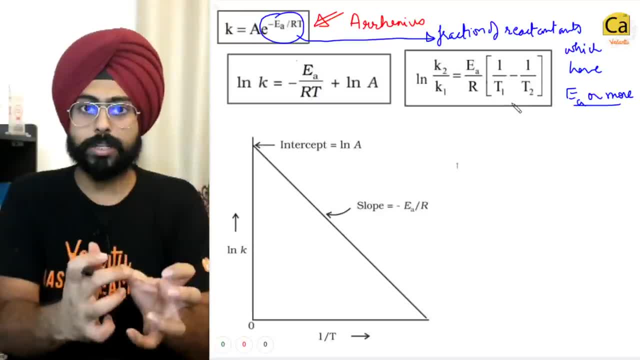 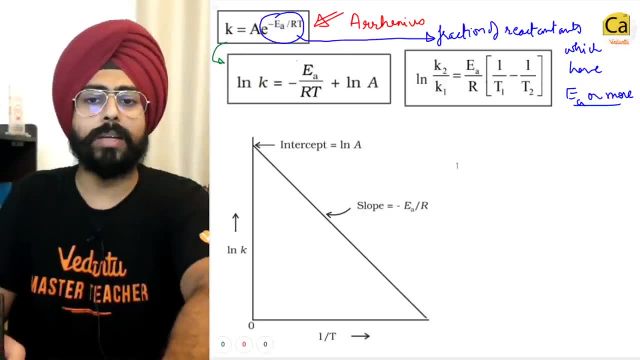 All you need to remember is that this denotes the fraction of molecules that already have the energy for the reaction to happen. So, once you manipulate this guy, if you take a lon, if you take T1,, T2, etc. etc. you 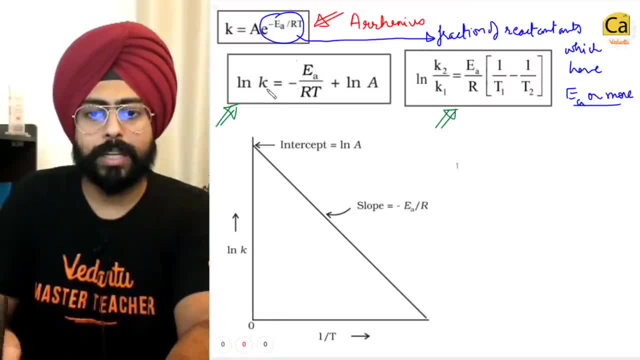 get these two forms, So you can get: lon k is equal to minus ca by RT, plus lon a. Yes, Then you also get lon k2 by k1 equals to a by R, so on and so forth. What is the inference over here? 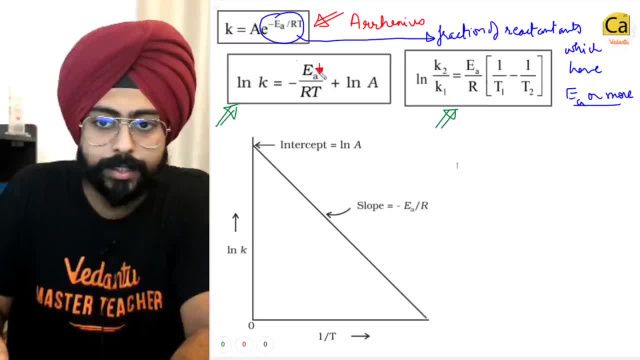 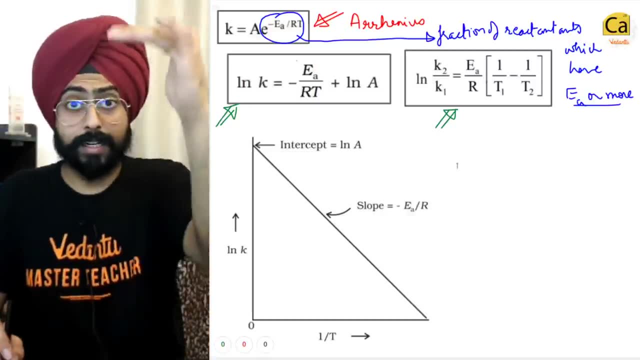 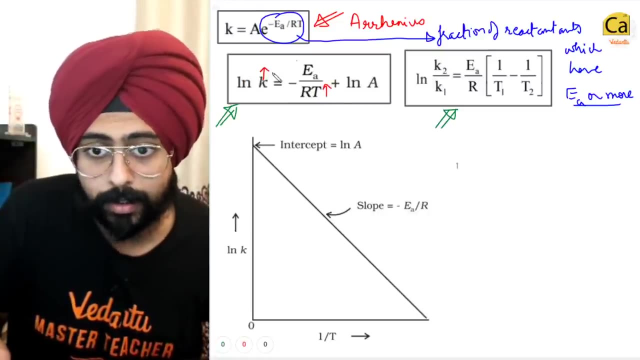 Inference is that if my activation energy decreases there's a minus sign. activation energy decreases implies k increases. Obviously right. if I decrease the activation, energy, reaction will happen faster. Very obvious: If I increase the temperature, k will increase. reaction will happen faster. 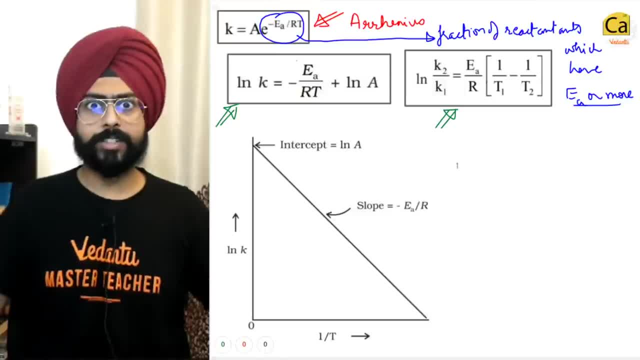 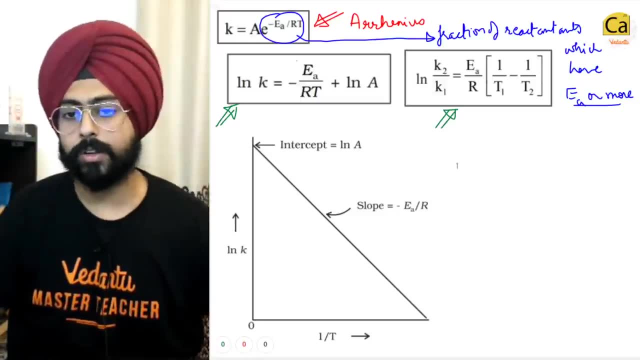 Notice the minus sign over here. yes, Obviously, If I increase the temperature, I'm automatically giving a lot of energy to my components, so my reaction will happen faster. Very nice, If you plot this on the graph, this is what it looks like. 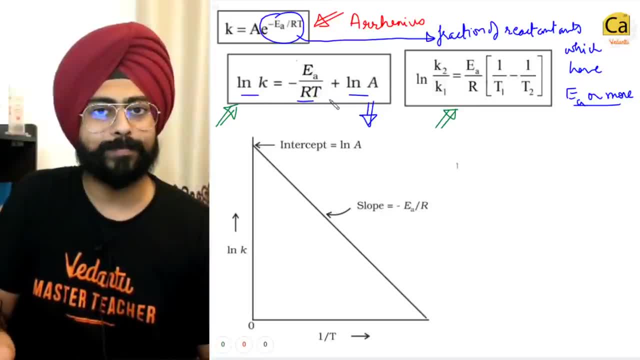 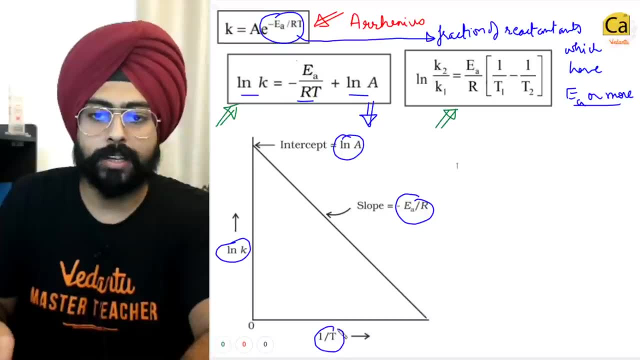 This is a straight line equation: y equals to mx plus c, The slope is equal to minus activation. energy by R intercept is lon a and this is lon k, versus 1 by T. the graph Very nice, And this is another equation that you might want to remember. the only thing that you 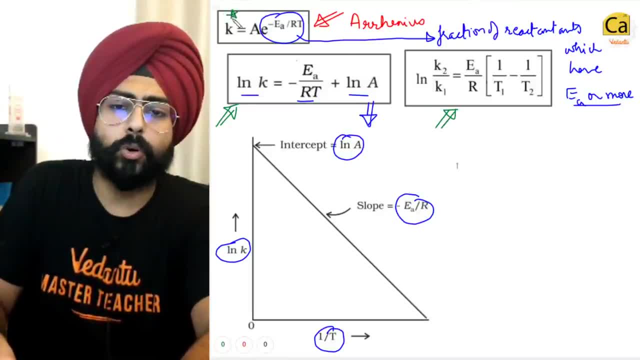 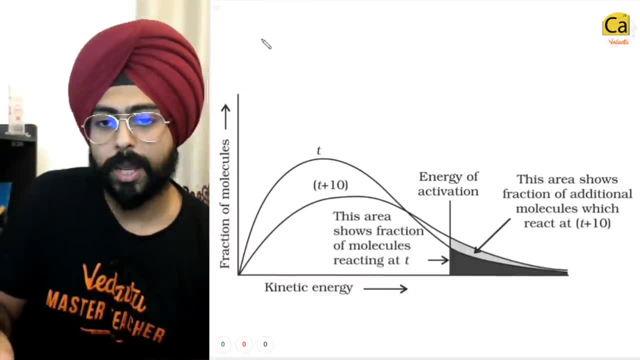 have to remember in this phase is this equation, Yes, This equation, which I'm pretty sure you already do, Very nice, Let's go forward now. This, my dear friends, is your very famous Maxwell Boltzmann's distribution. yes, 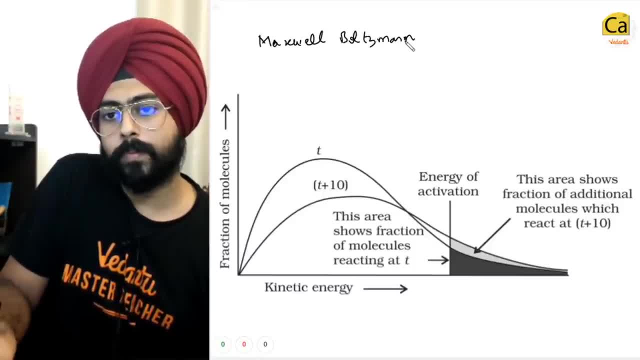 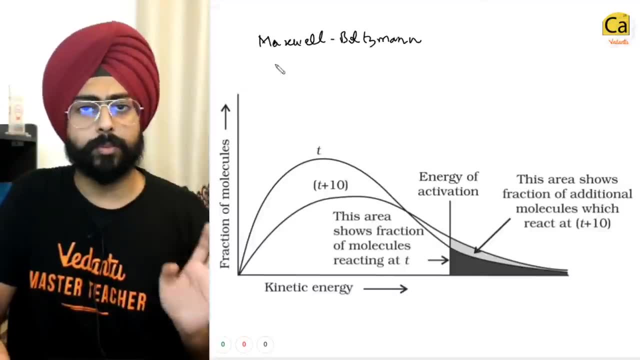 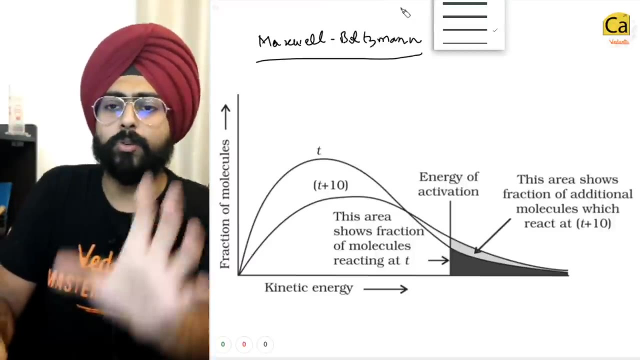 Cool, Boltzmann's spelling has become weird, but I'm pretty sure you know what it is. Maxwell Boltzmann. distribution- okay, it's a probability distribution function. Okay, More details of this. You might have learnt about them. you might have known about it in mathematics, but no. 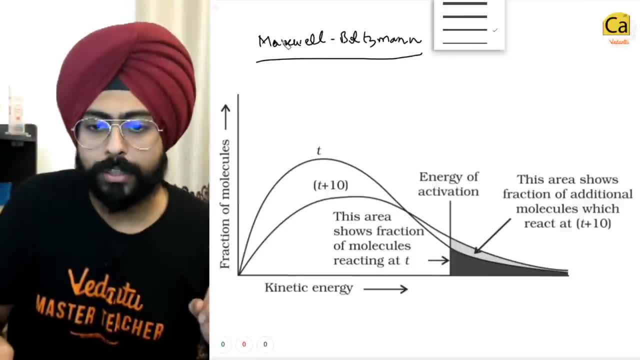 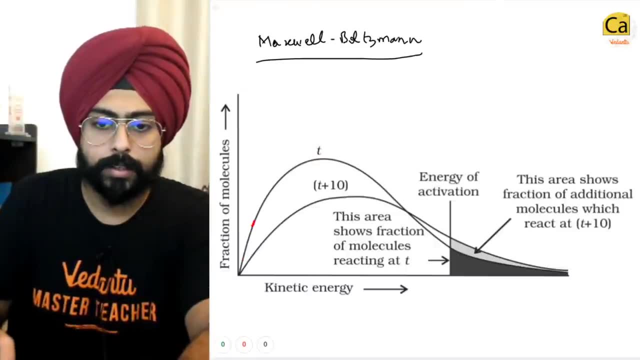 need to learn about the nitty gritties of it in chemistry. All you need to know is: all you need to know is that the graph at T- okay, look at what it is at T See a very tall graph and it dies down, fine. 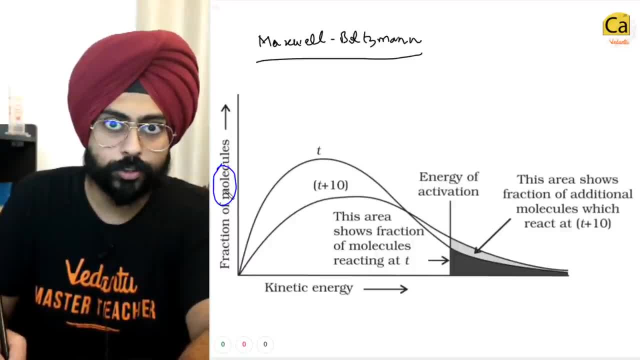 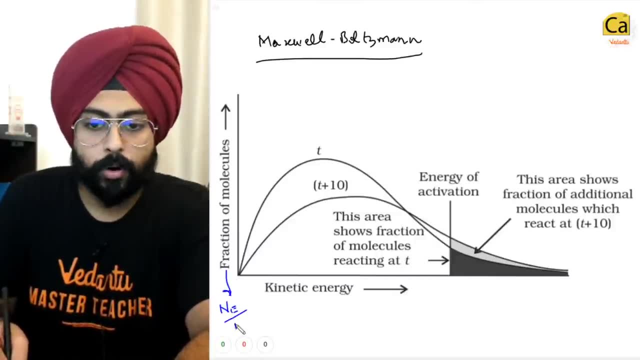 So what are we plotting over here? We are plotting the fraction of molecules. fraction of molecules, okay, fraction of molecules is n of a certain energy Upon n total n? e. y n t means n with a certain energy. let's say, for example, this fraction: 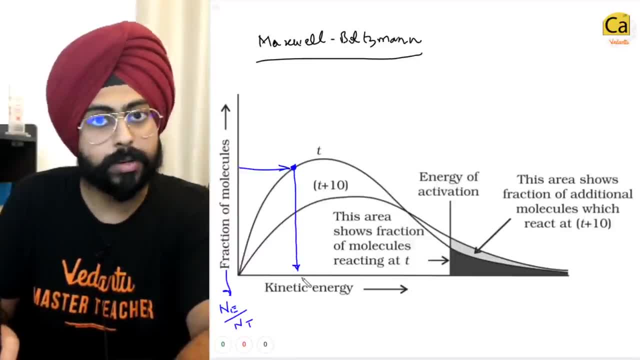 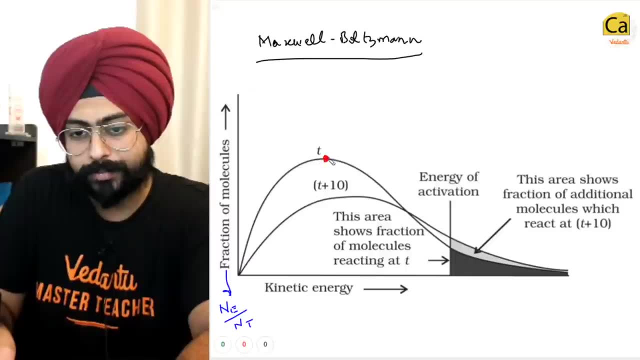 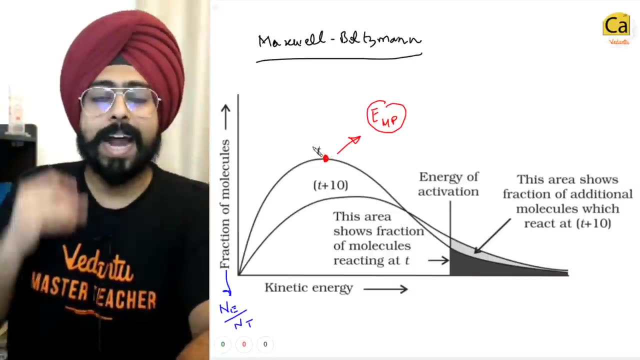 has this much energy. okay, this fraction has this much energy, So n of a certain energy upon total number of molecules. So, my dear friends, everyone knows what is this energy called? This energy is called the energy most probable, most probable kinetic energy. 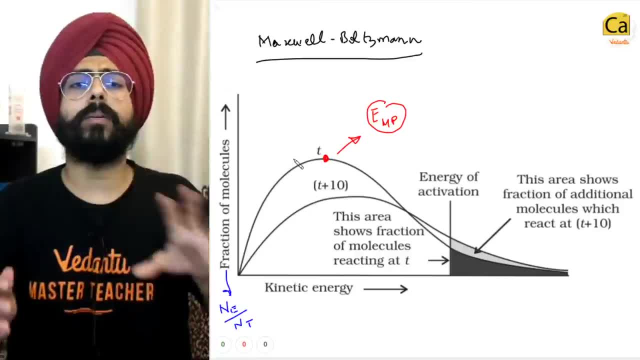 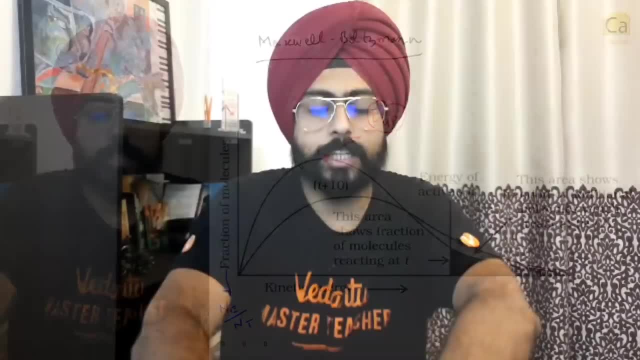 At lower temperatures the peak is higher. Yeah, Imagine something like this. This is the example of a classroom. Maxwell Boltzmann distribution is best understood as a classroom of students. okay, So let's say you are sitting inside a classroom, everyone, 50-60 students and then everyone. 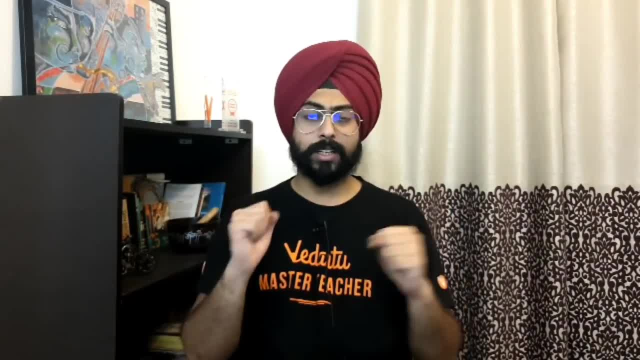 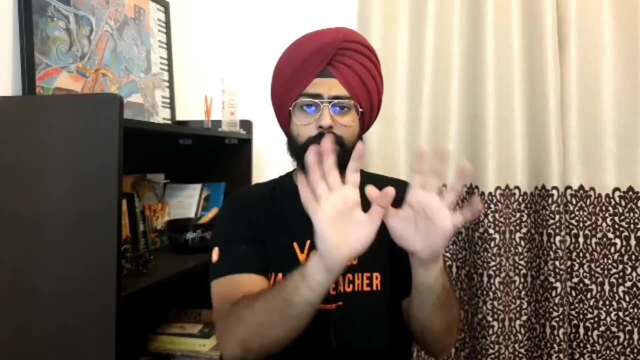 is at lower energy. okay, So some people are always there which are energetic. they will be talking to each other. some people are just doing this and chilling, not doing anything. yeah, That is the usual distribution at a normal temperature. fine. 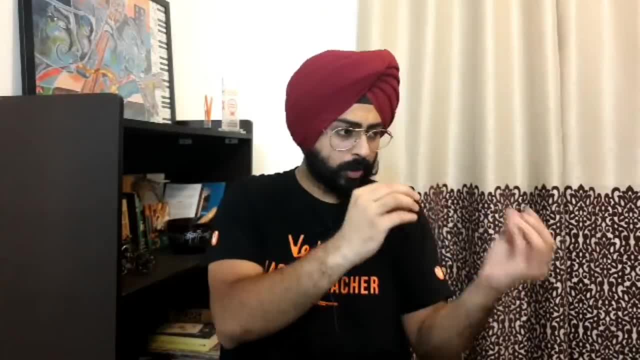 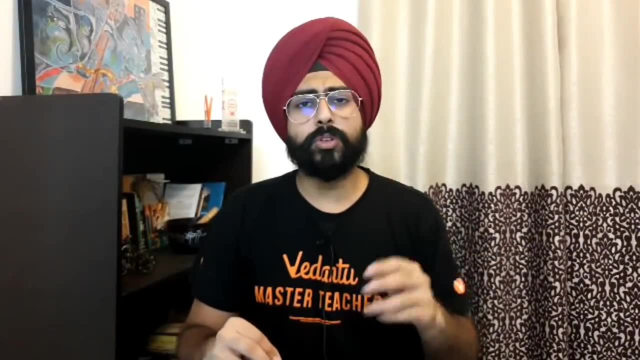 So there are only a few people with high energy. yeah, so a few people with very high energy. sorry, There is one guy who is just running around all over the place. yeah, But most of the people are just chatting with each other. 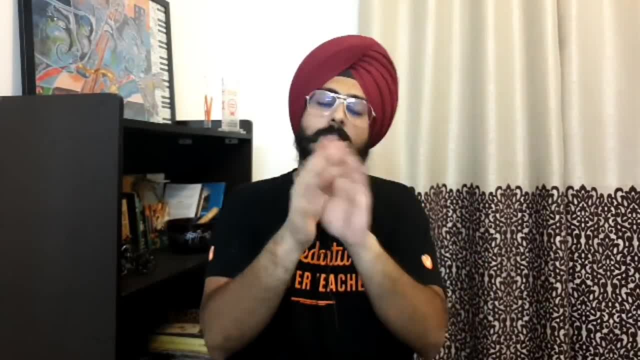 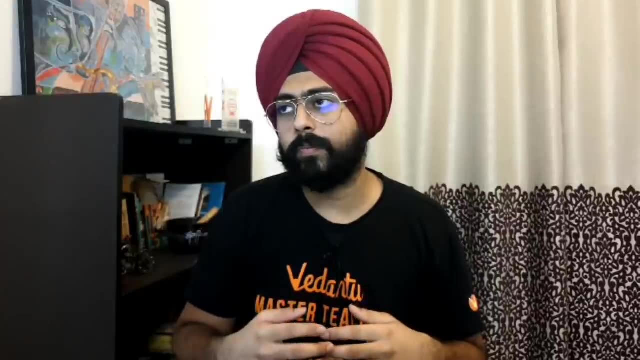 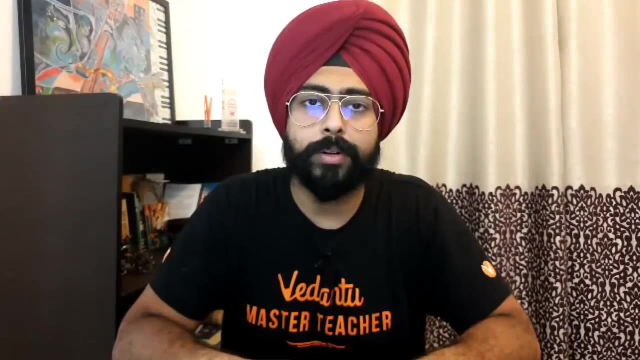 So that forms the most probable energy. Most people are chatting with each other and some people are just lying down, fine. Then if the teacher comes into the class and starts singing a song perhaps, or if the teacher comes in and says there is a quiz today, there is a surprise test today, what will happen? 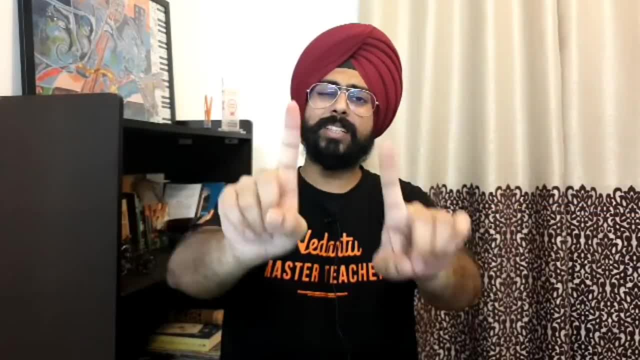 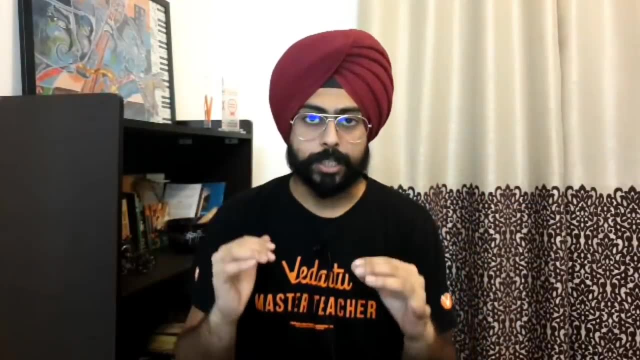 The energy of the entire class will suddenly increase. There will still be someone who is sleeping. Yeah, The person who was running will start shouting and running now, And a lot of people who were chatting earlier, with this much amount of energy, their energies. 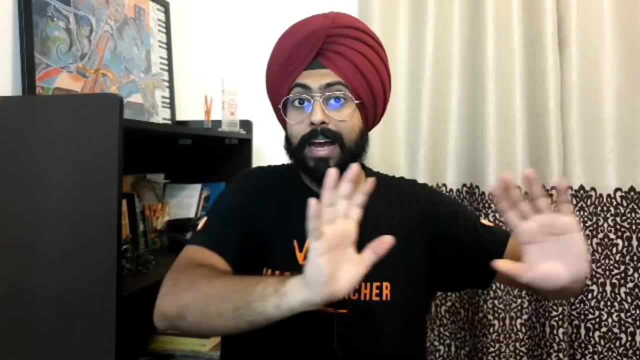 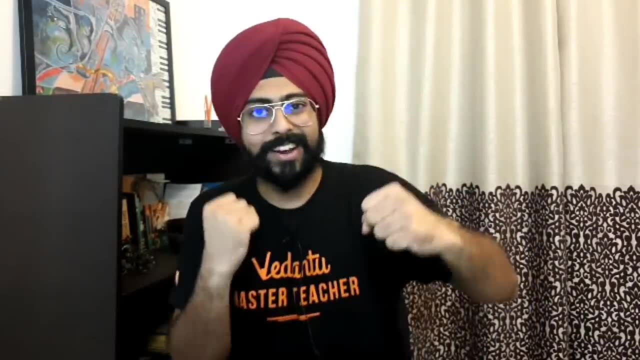 will also spread apart. yeah, More people will have higher energy, and everyone's energy will be different. Someone will say, oh, I haven't prepared for the test. someone will say, yes, I have prepared for the test, so on and so forth. 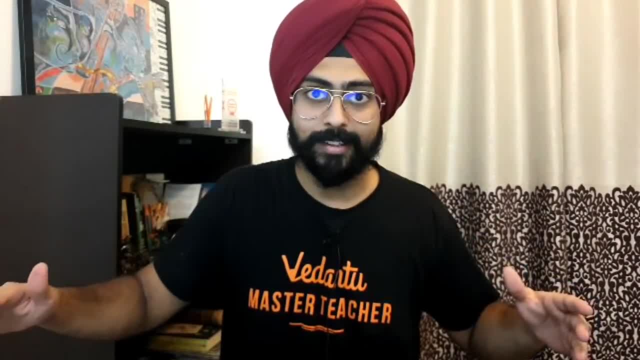 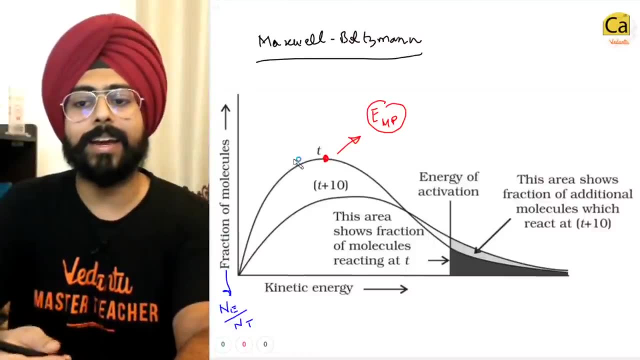 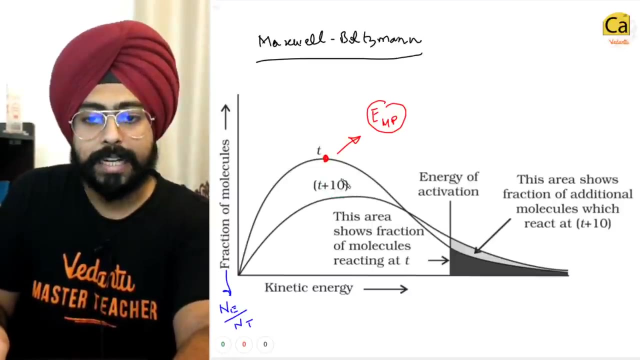 So now everyone's energy is a little more different from each other and everyone has a little higher energy than the earlier case. Yes, So the same is depicted over here in the diagram that we have fine At temperature when it is increased by 10 degrees Celsius. okay, temperature ko maine. 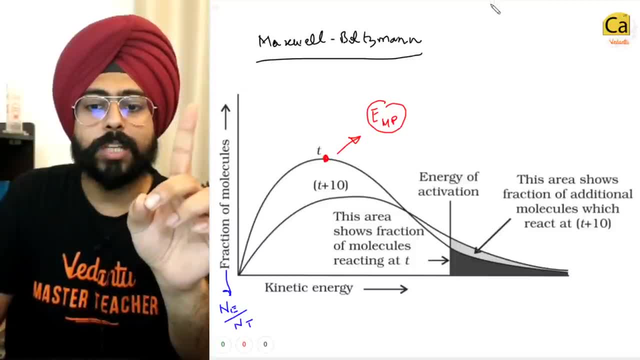 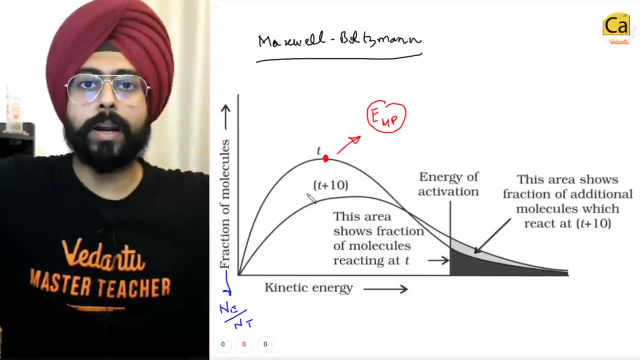 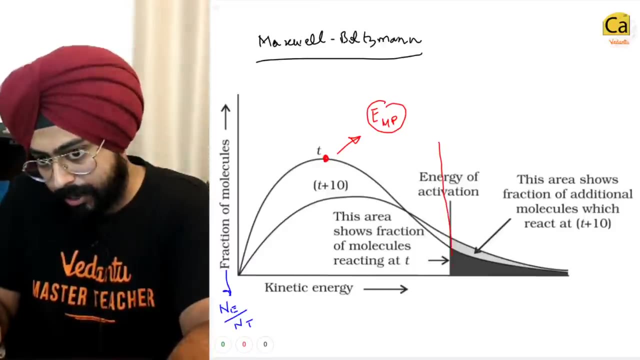 sirf 10 degrees Celsius. se increase, kiya. what's happening over here, Do you see? the curve gets flattened. Everyone's energy is now more different. The curve is now more spread out. Everyone is acting a little different now the curve spreads out, and if this energy is, 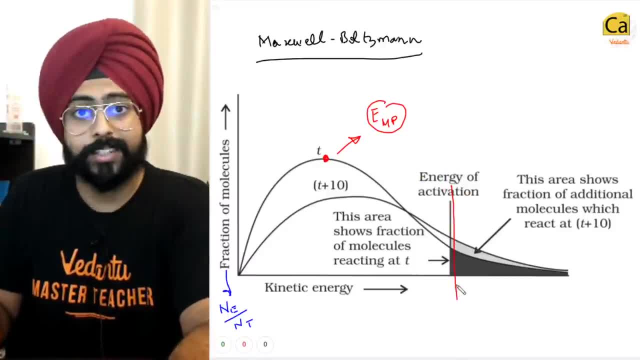 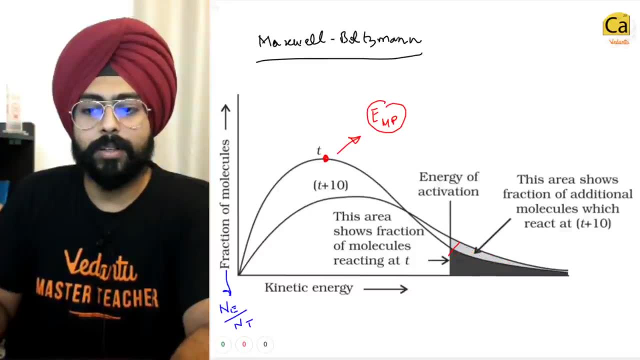 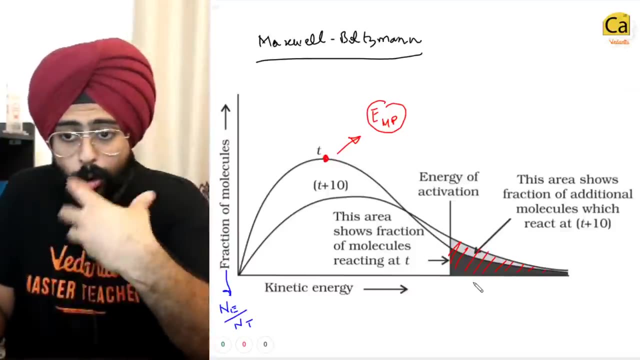 the energy of activation. If this is the amount of energy that is required for the reaction, now more number of molecules have that energy. yes, pretty simple. Do you see the part that I have shaded in red? It is higher than the part that is shaded in that dark, grey, black colour. 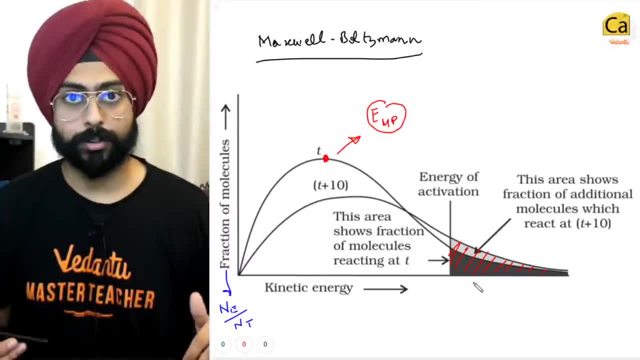 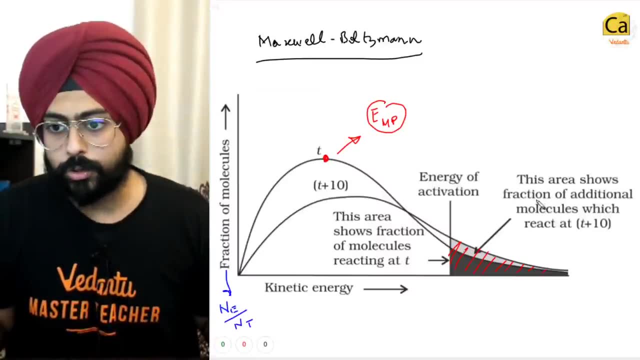 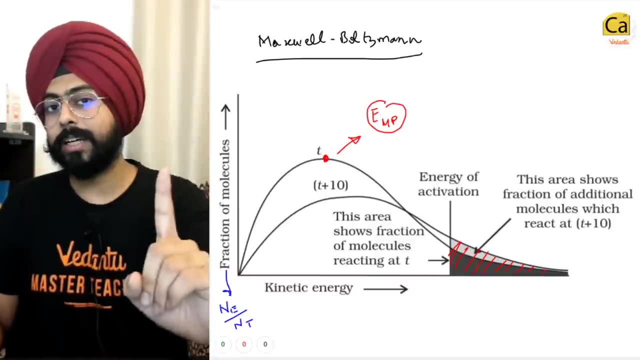 More molecules now have energy, more than the energy of activation. So Maxwell-Boltzmann distribution best understood by that classroom example. okay, So this light grey area shows the fraction of additional molecules which react at T plus 10.. This is why rate constant increases with the increase in temperature, because now there 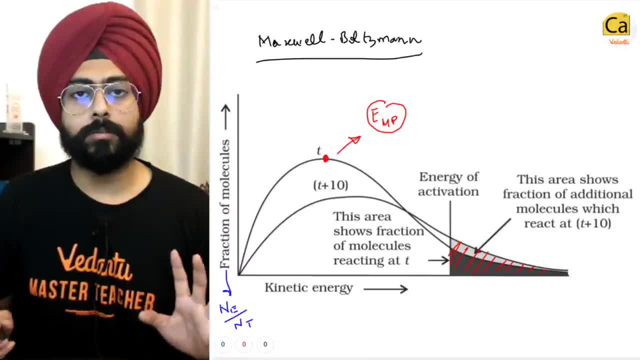 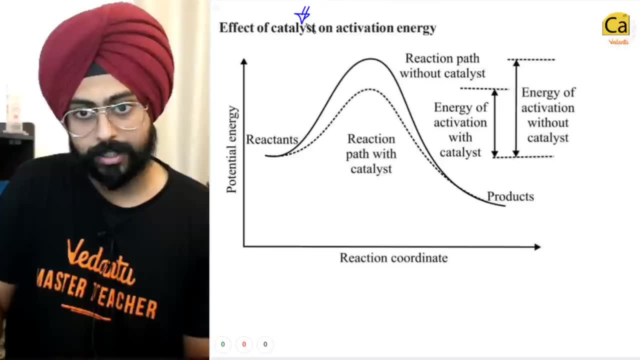 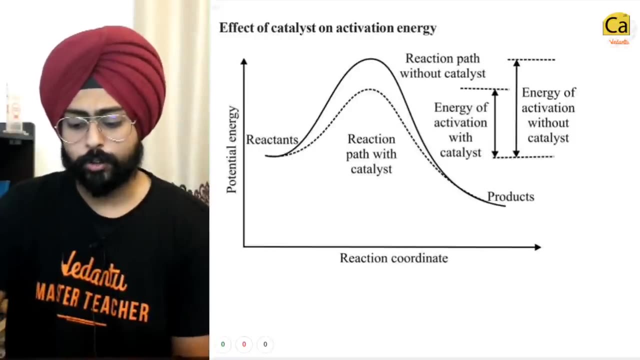 are more molecules that have the energy to react. as simple as that, fine, nice. Now let us think about the effect of a catalyst on activation energy Catalyst is like beach ka bandar, it's like the middle man. okay, It's like this: you want to eat mangoes, but you are in lockdown, so what you will do is 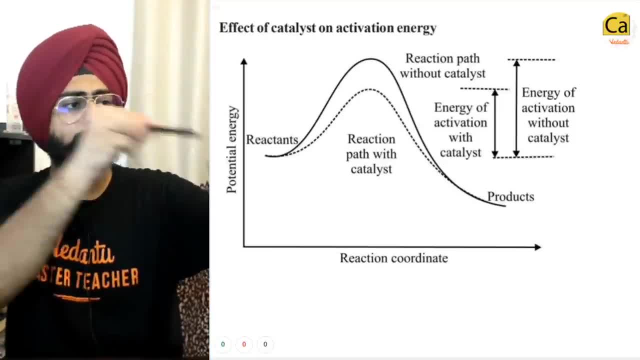 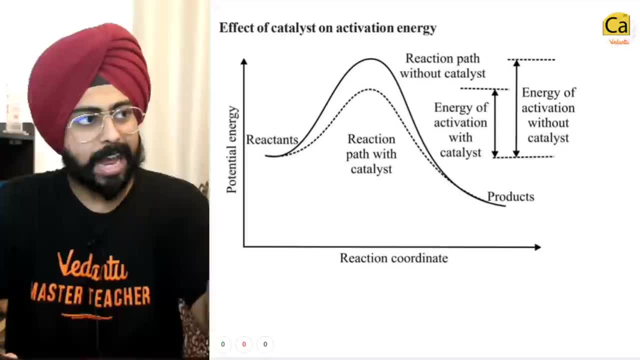 you will open an app online, some grocery app. You will put: I want mangoes and two days later you will get the mangoes. maybe one day later, depending on wherever you are in the lockdown. So what that app has done, what that middle man has done, is that it provided a pathway. 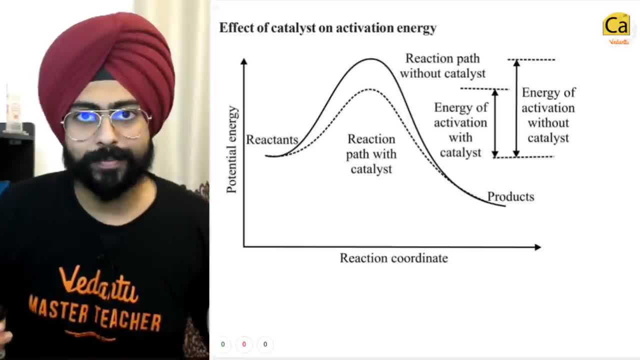 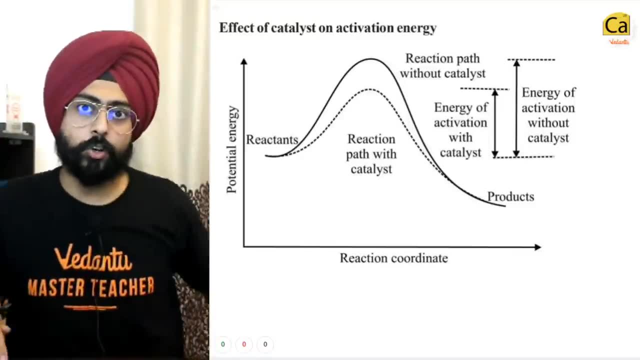 for you to get mangoes, which is easier, yeah, Otherwise you would have to wear a mask and you know, prepare yourself, wear gloves maybe, then put a sanitizer in your pocket, then go out, then tell police I am going to buy mangoes, etc. etc. 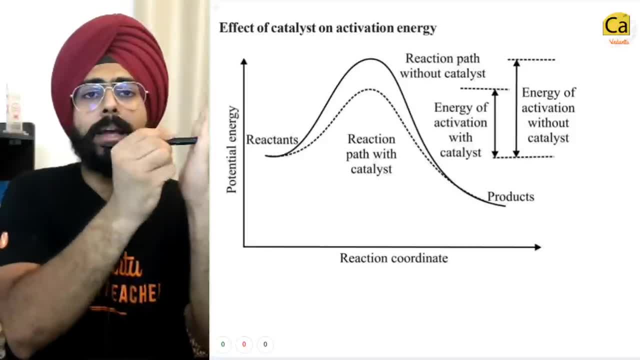 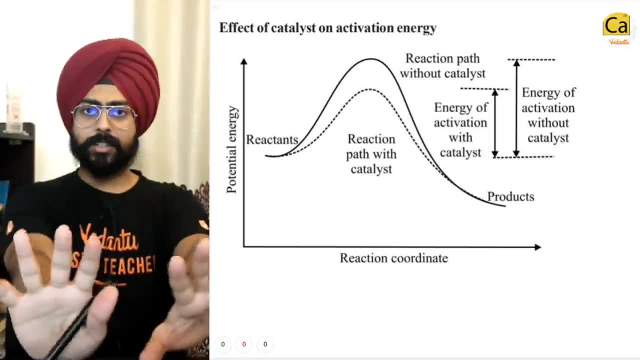 But now, just by using that app, just by using the middle man, Just by using that app, just by using the middle man, Just by using the catalyst, you are able to obtain the mangoes easier. Reaction is still the same: you wanted mangoes, you get mangoes. 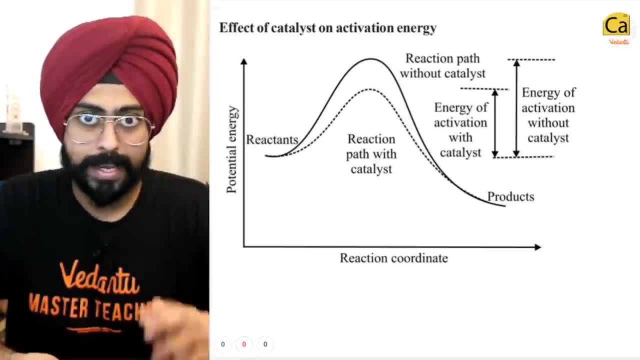 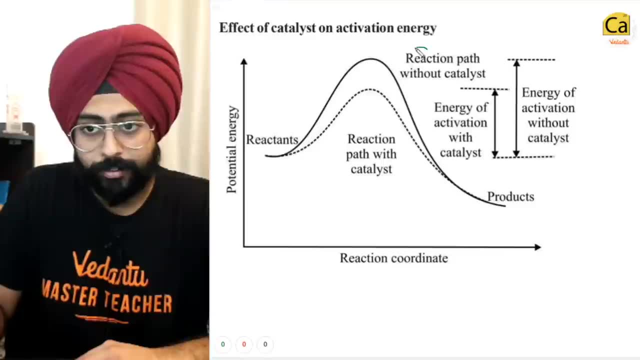 But there is an alternative pathway that is provided ek alag tara ka zariya mil gaya us kaam ko poora karne ke liye. fine, So if the path without the catalyst took a lot of activation energy with catalyst the. 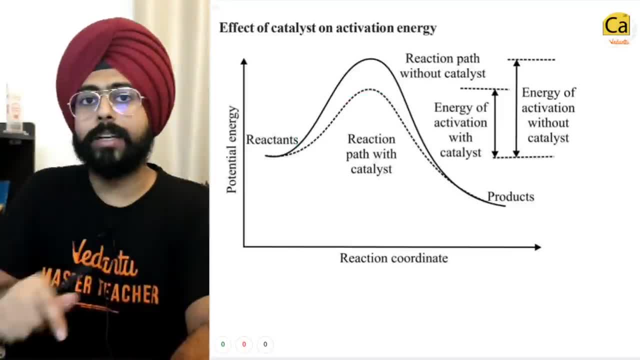 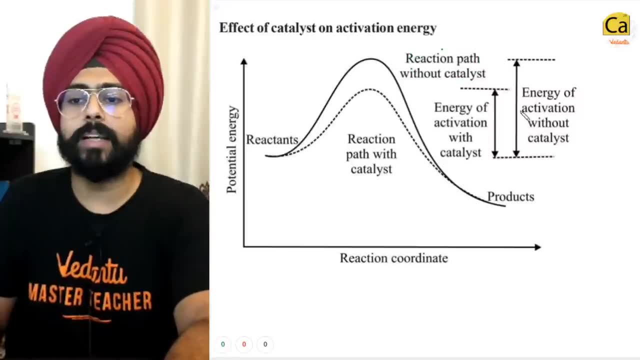 activation energy is reduced. And we just saw from the Arrhenius equation: Arrhenius equation: that if we reduce activation energy, k goes up. very nice, yeah. So reaction without catalyst needs higher energy. So yeah, catalyst just reduces the activation energy, makes the reactions faster. catalyst- 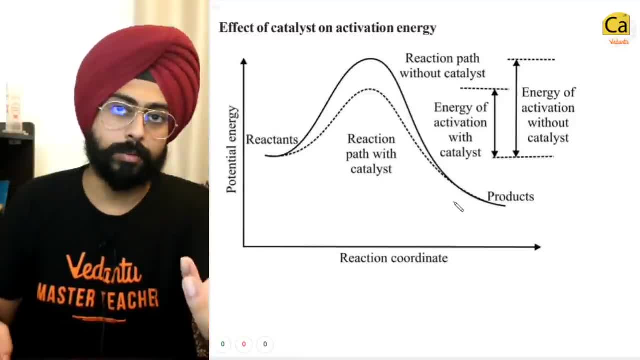 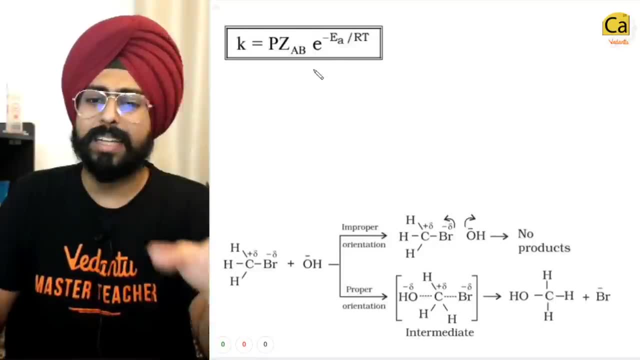 does not have any effect on the equilibrium. as simple as that. Now, the last thing on which hardly any questions are ever asked is pe koi question nahi aata kabhi bhi. still, you can watch it if you want. So what have we done over here? 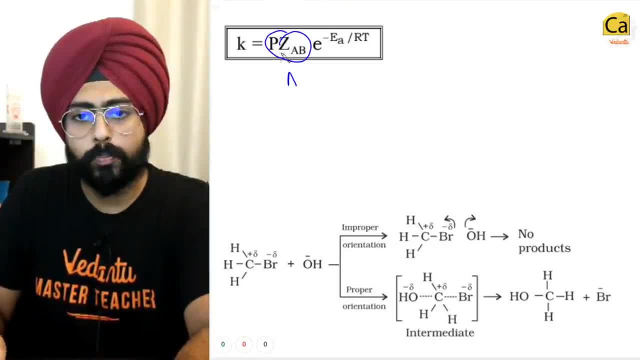 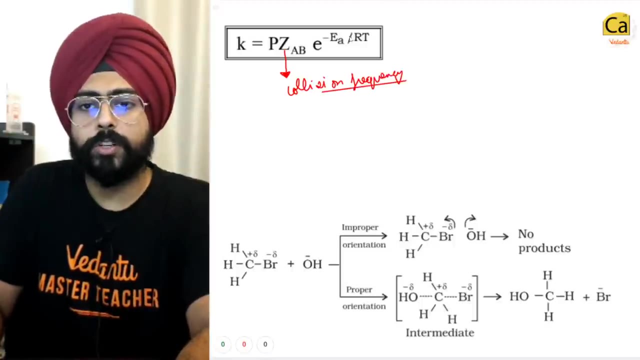 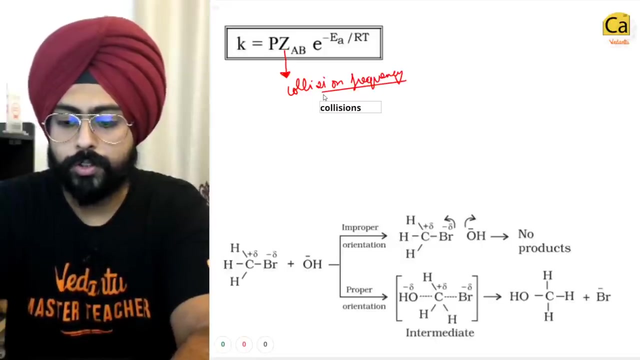 Instead of writing Arrhenius constant a, we have written p into z. what is this p into z? Achcha sochke dekhte hain. see. z is known as the collision frequency. okay, Collision frequency bole to. this is equal to collisions. collisions per unit time, per. 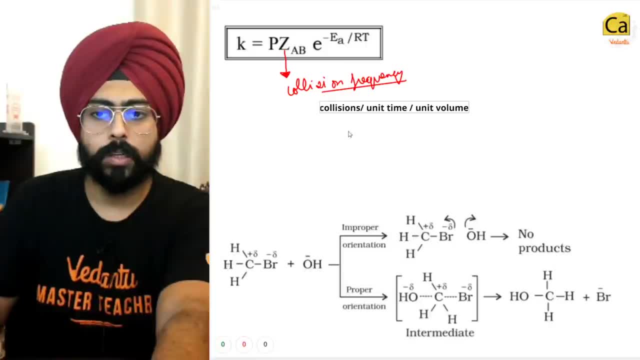 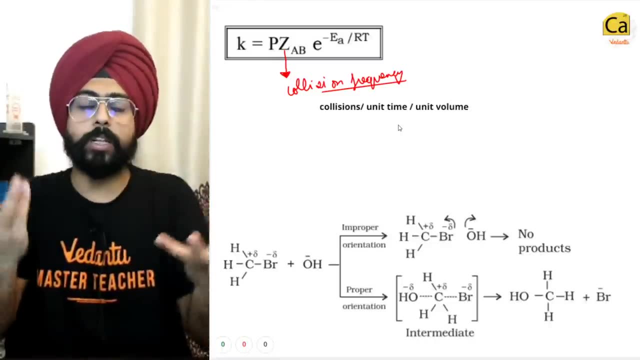 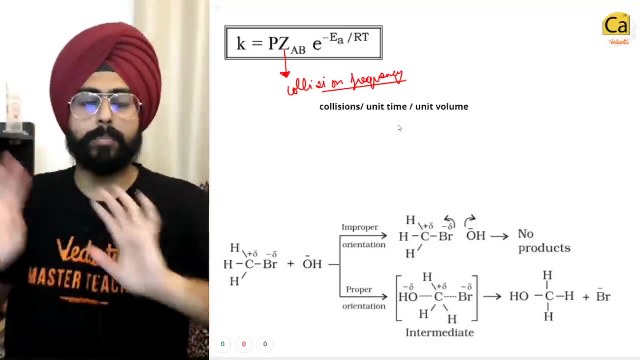 unit volume. So in a unit volume in one cubic meter, let's say how many collisions are happening in one second. this is what it tells us, Because the number of collisions will directly affect whether the reaction is happening or not. we just understood that. 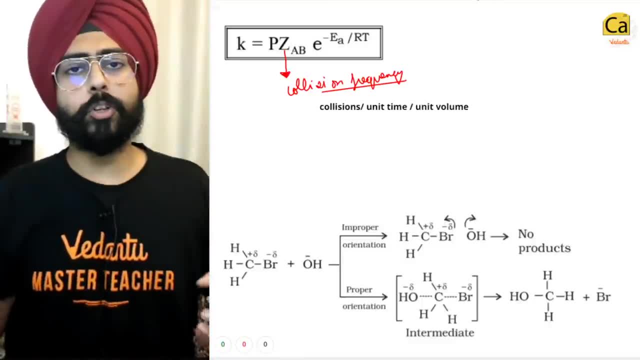 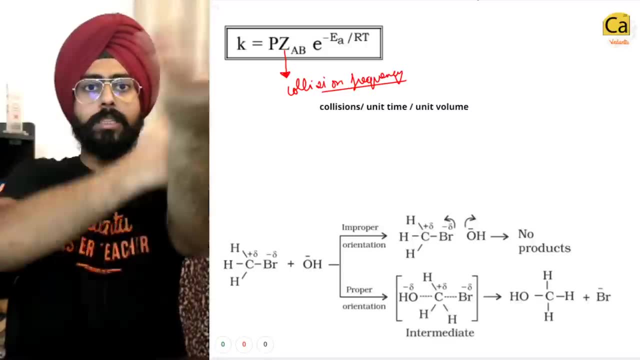 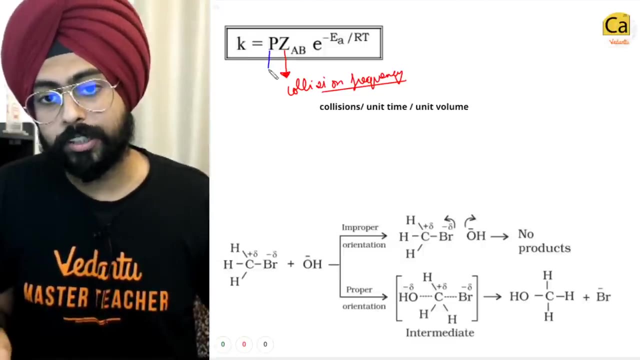 Now the collisions. it's not necessary for the collisions to happen in the perfect manner in the first go. The collisions might happen in a different manner. Yeah, But you want only this collision. So the term p accounts for the probability of the correct collision. okay, 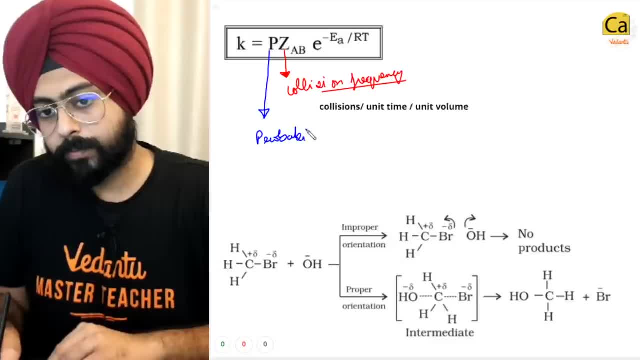 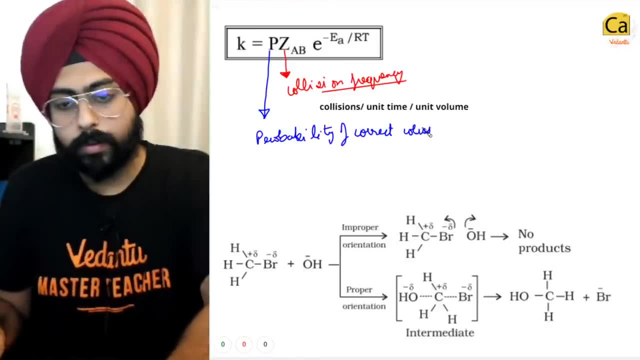 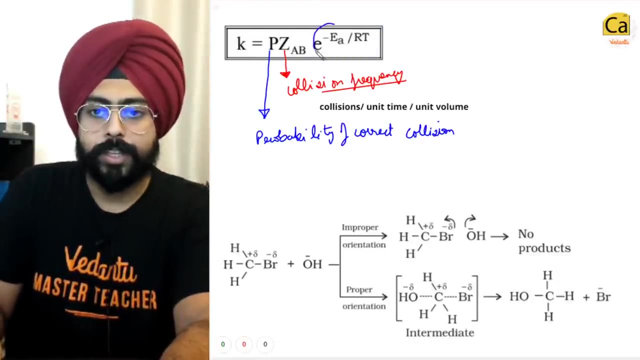 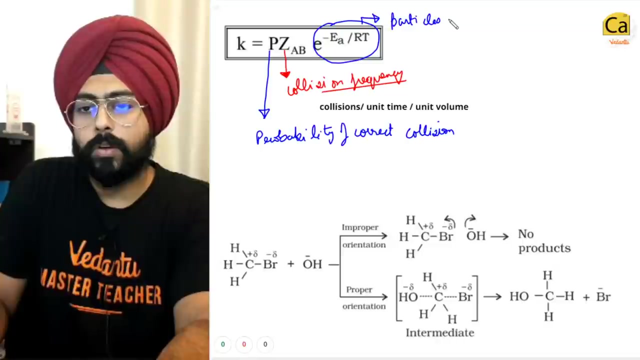 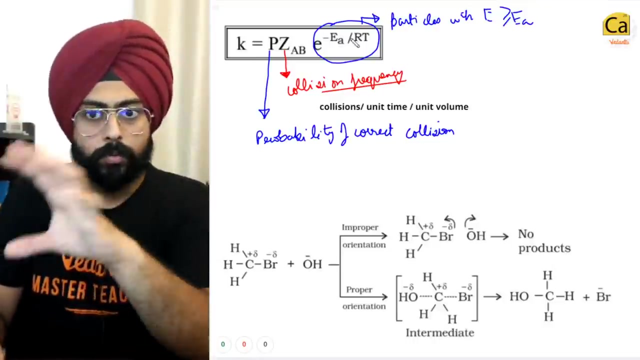 This term accounts for the probability of correct collision. okay, So do you realize this is a very complete idea? Okay, So, in other words, this marks the particles, I would say particles with energy greater than activation, energy greater than or equal to 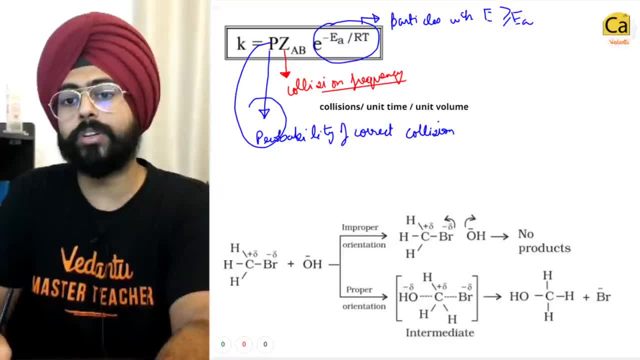 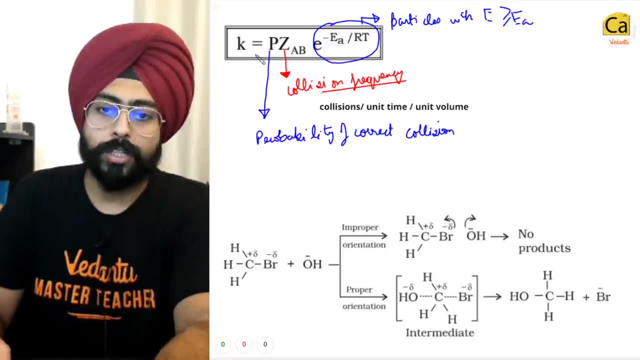 So energy is taken care of, collisions are taken care of and probability of correct collisions is taken care of. This is the more advanced idea of thinking about the rate constant, but more questions are not asked from this. Even if they are asked, they are only in those areas. 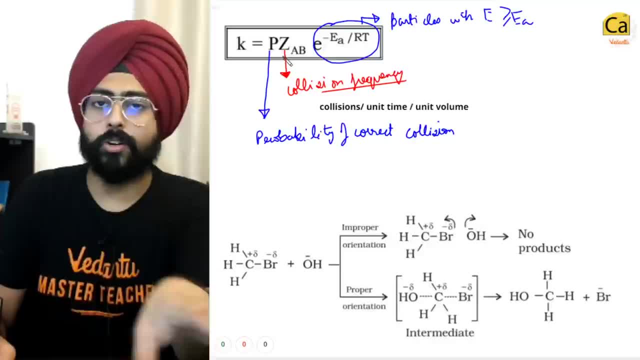 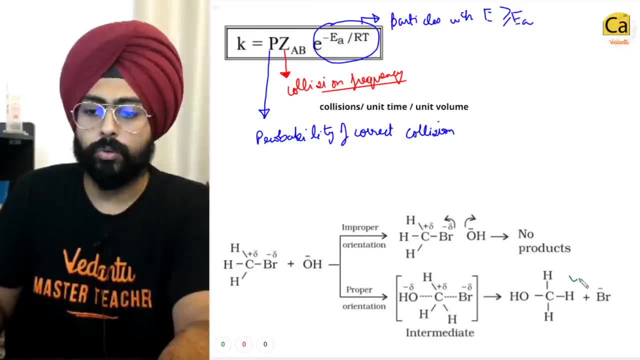 In those advanced level books. in examinations, ideas from this point are not asked generally. Okay, So this is just an example of how improper orientation would give you no products, but proper orientation would give you the products. This is an example of SN2 reactions, by the way. 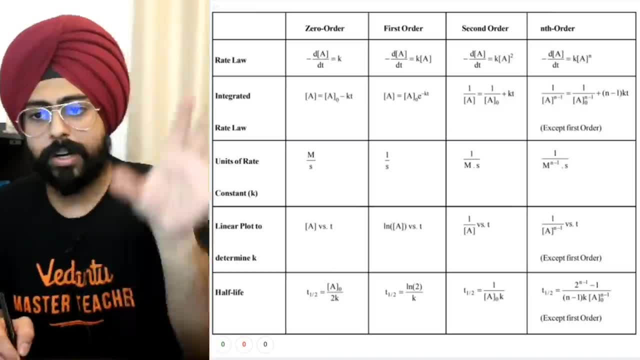 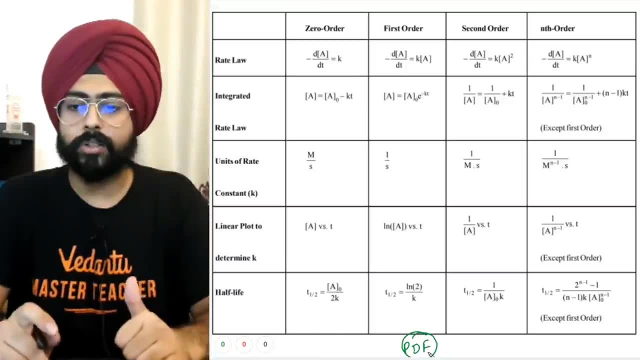 Fine, Technically speaking, the theory is over. This is one table over here that I have. I will give you the link of the PDF in the comment section of this video. later on I will put the PDF link in the comments. So this is a summary sort of a thing, okay. 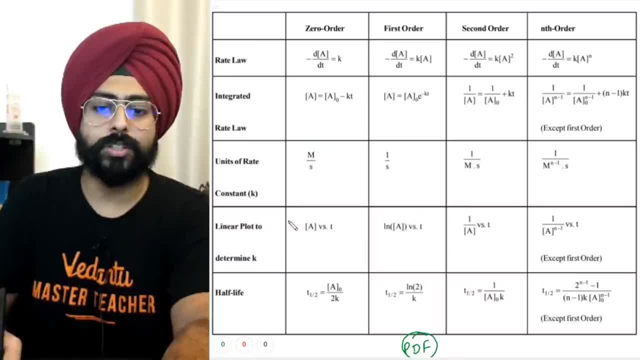 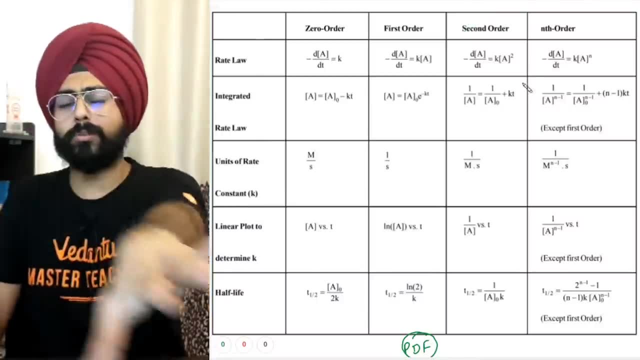 For zero order. what will be the rate law? integrated rate law units plot? what does it look like? half-life formulae: second order, nth order, etc. etc. But these you don't need to remember. 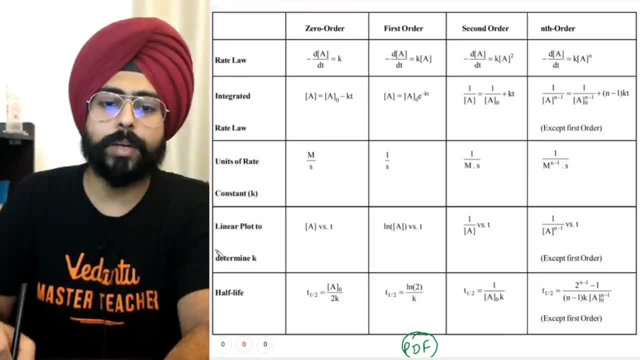 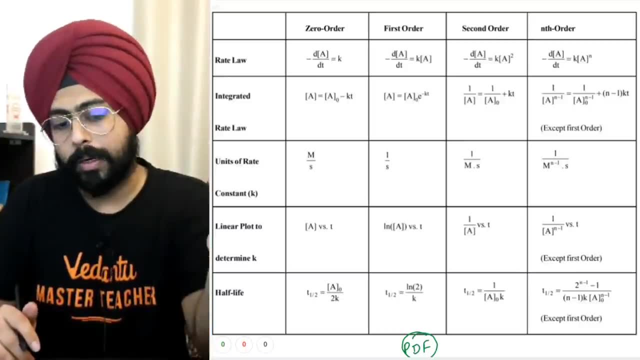 This is over here. Now, before ending today's class, there is a special message that I have for you guys. It is an advertisement. I am already telling you, but advertisements are what allow us to keep classes for free, because some people pay for it. 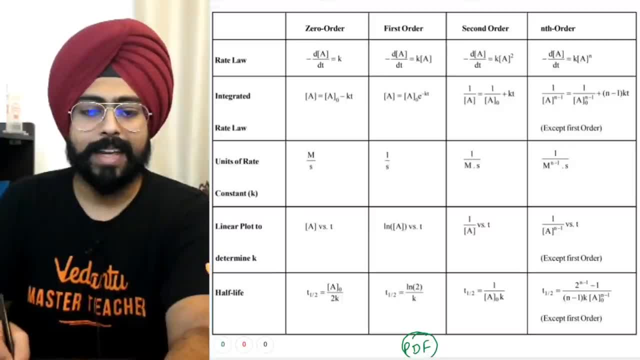 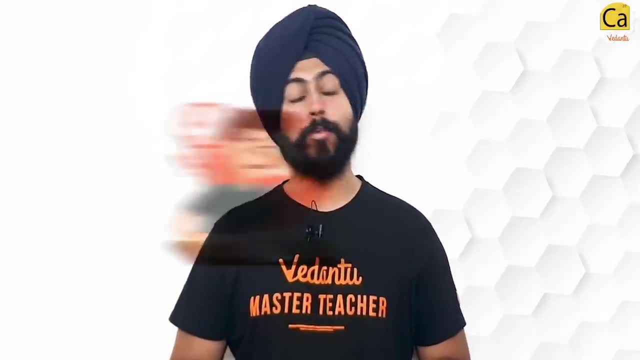 Yeah. So just a quick advertisement for all of you guys, and then I will chat with you. Exams are really close and at this time, if you're not satisfied with your preparation, I'm sure you're stressed out, Don't worry. 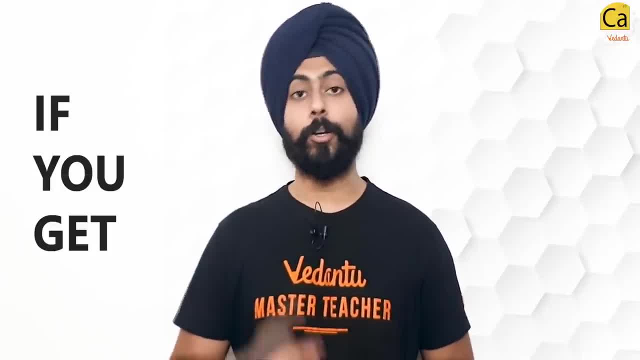 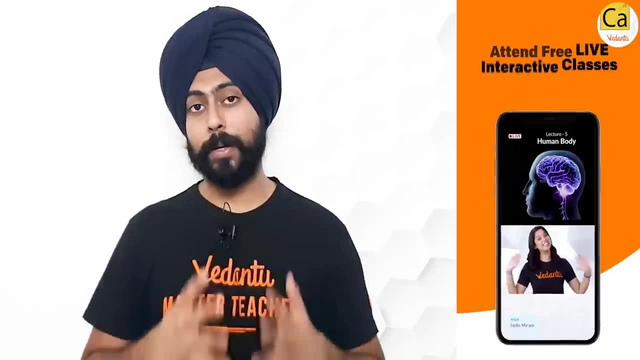 Lots of improvements are possible in this short span of time if you get good guidance. And for that, Vedantu brings you crash courses for J&E. These live sessions will happen on Vedantu's patented platform, So your interaction with the teachers will be really good. 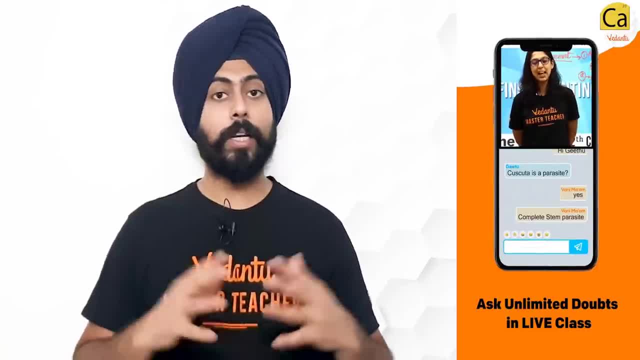 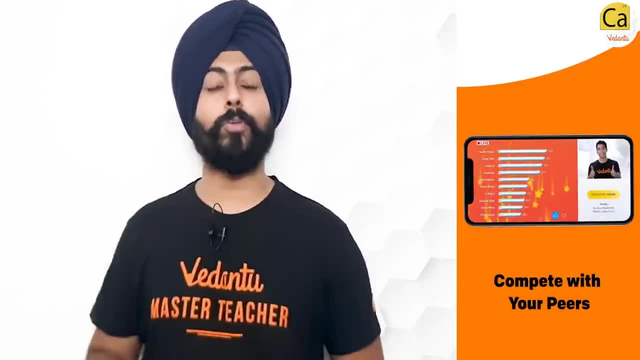 And you can solve your doubts Much better. As a part of this course, you will get a lot of study material, short notes for theory, short videos for revision, basic level, advanced level, multiple choice questions, previous year analysis, etc. 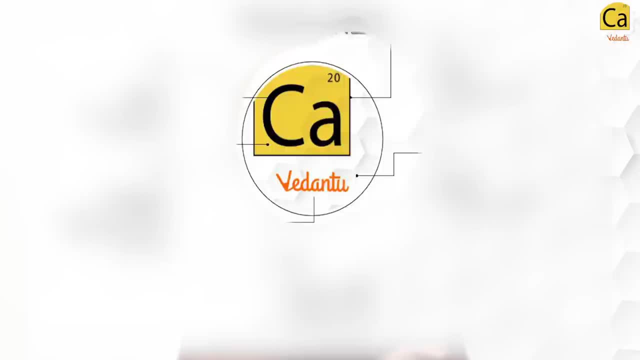 You will also be a part of the test series. in this course. You'll get to take lots of mock tests regularly so that you can analyze your progress throughout this course. Also, all the live sessions. their recordings will be made available to you so that you. 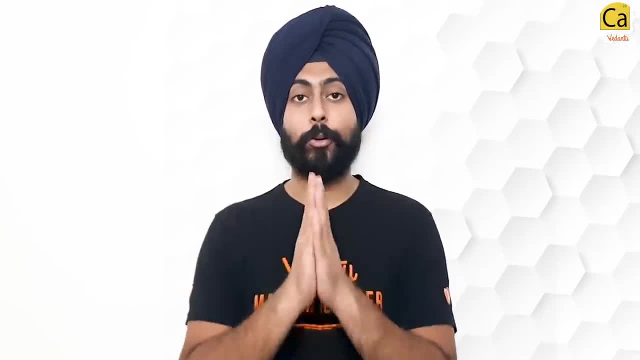 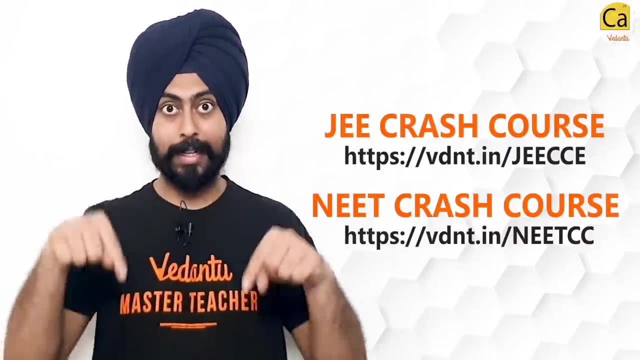 can revise them again anytime you want. Now, If you want to enroll for these courses, the links are right here on the screen. You can type them in your web browser. These links are also down in the description box. Since you're a regular student at catalysis, I will give you a discount code. 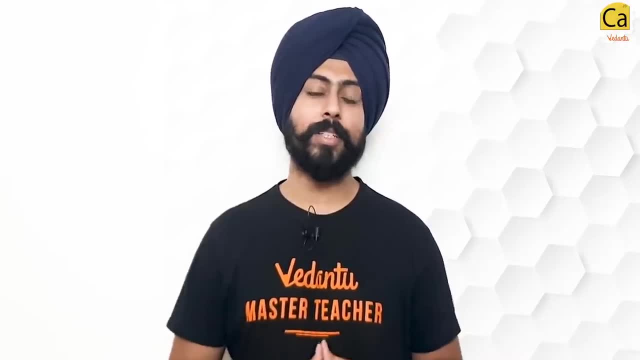 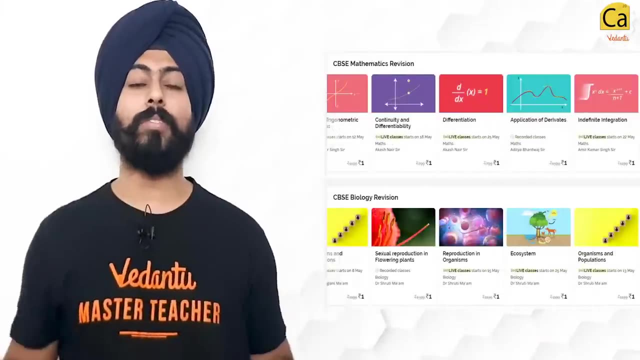 Use this to get a really good discount. I know these advertisements can become annoying and irritating at times. Well, only because some of you choose to purchase these courses, we at Vedantu are able to provide so much free education. Thank you so much for your support. 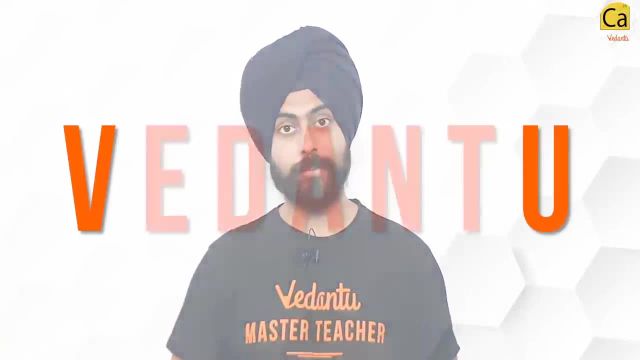 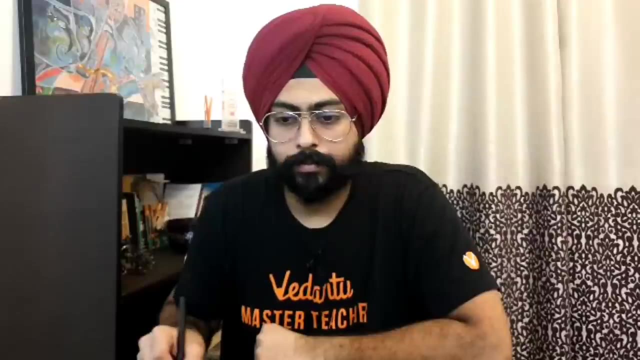 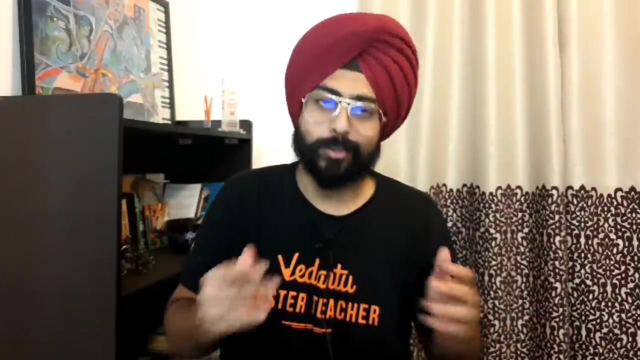 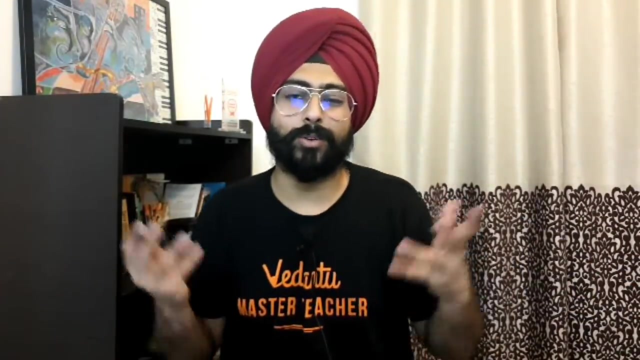 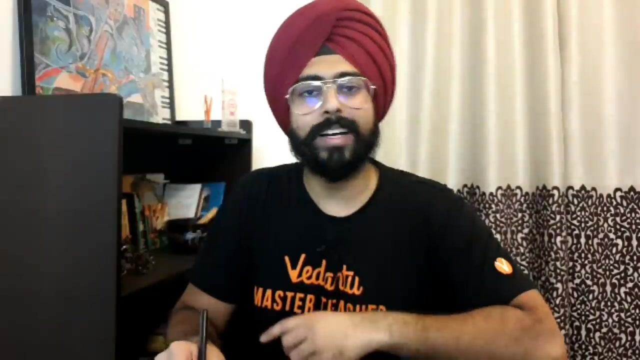 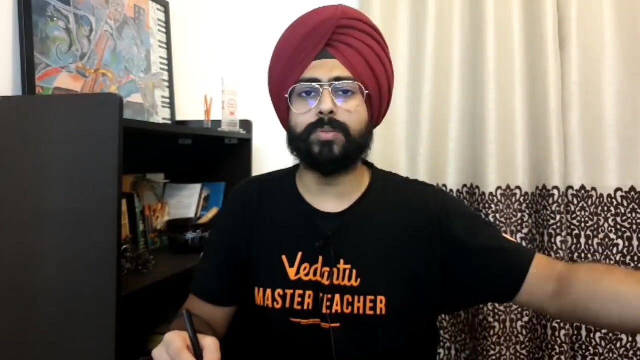 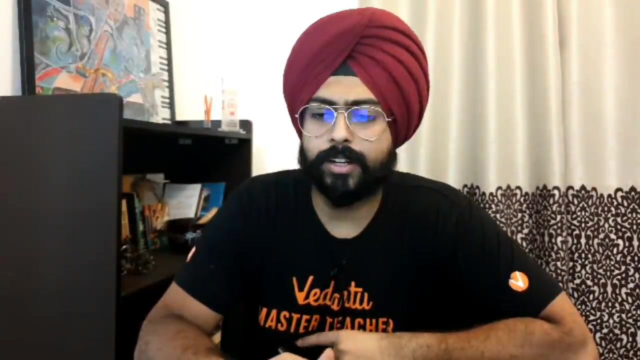 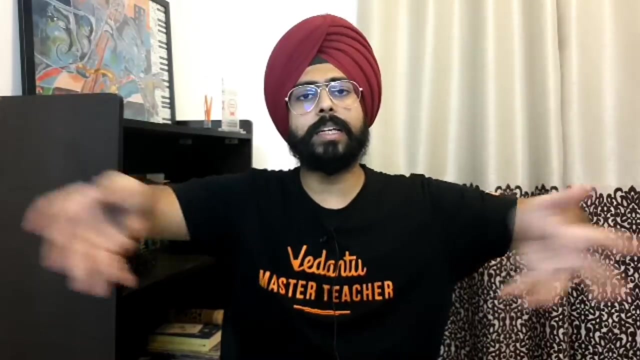 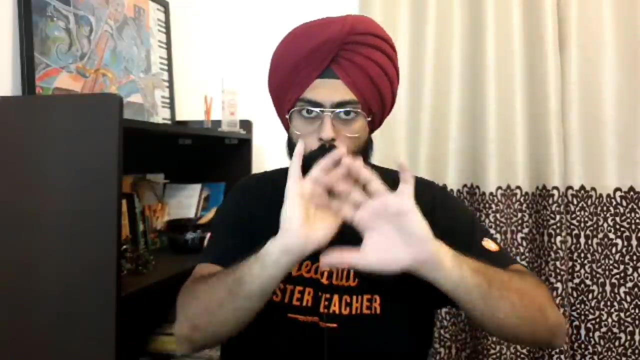 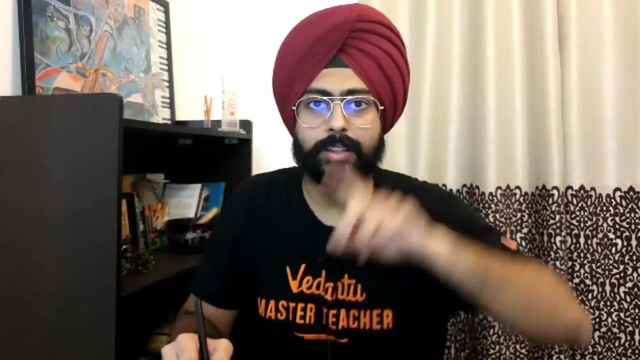 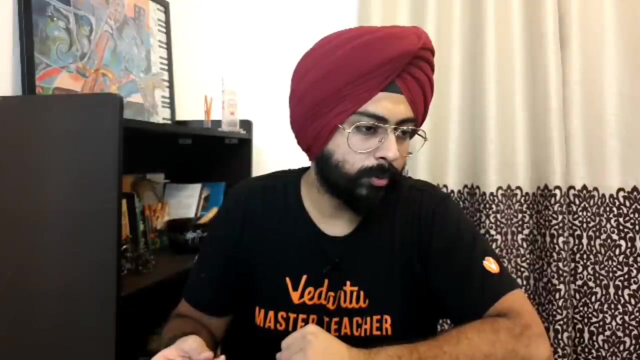 Because we love you. We are nothing without you. Vedantu Bye frequency and correct probability that we talked about in the end in the PZ. Sahiba is saying, sir, SN1 and SN2 have first order molecularity. so, Sahiba, SN1 means substitution. 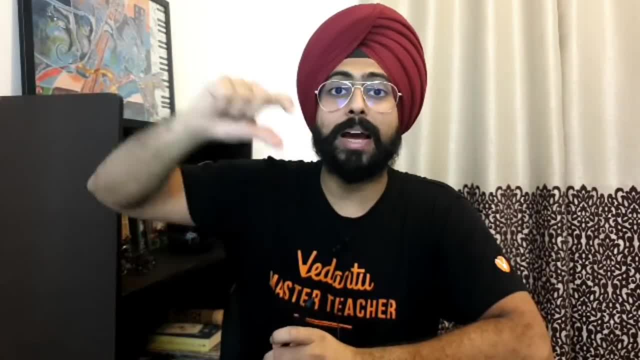 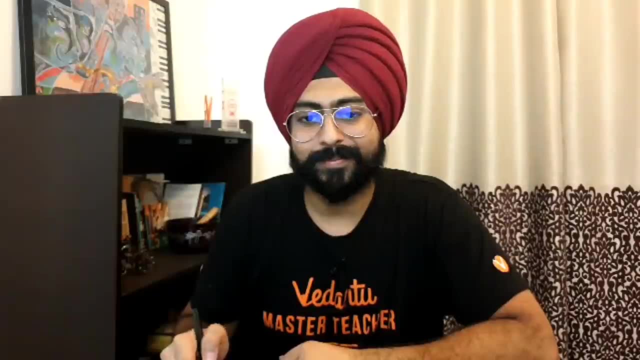 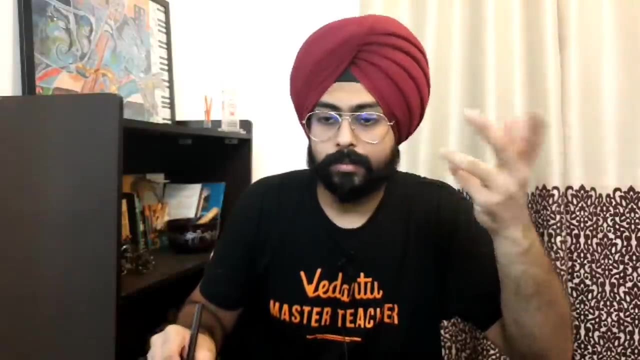 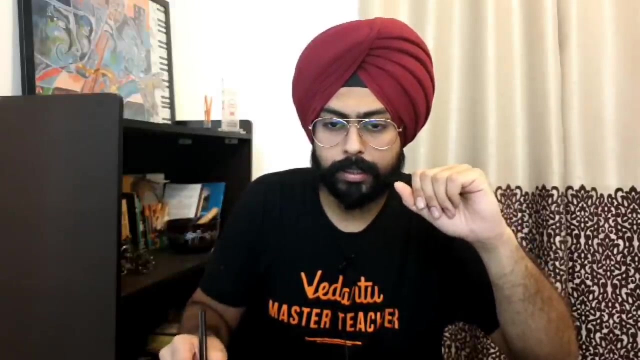 nucleophilic unimolecular. SN2 means substitution nucleophilic bimolecular, So the 1 and 2 over there refer to molecularity of the rate determining step. Incidentally, the order is also 1 and 2, but ideally speaking it refers to the molecularity. Chalo ji is link ko copy kar dete hain Awesome. 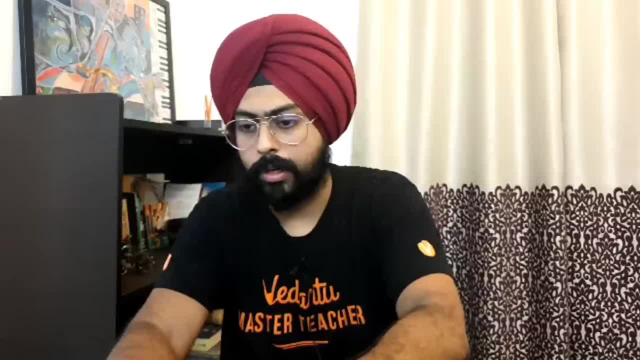 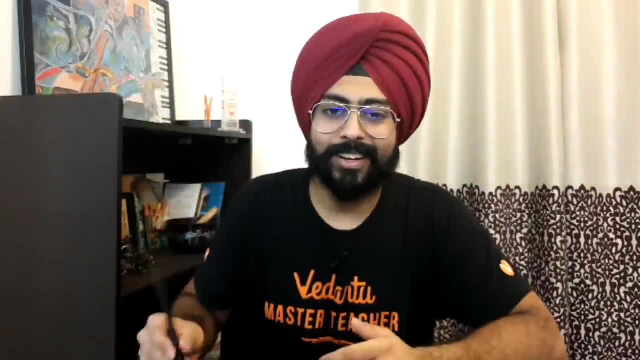 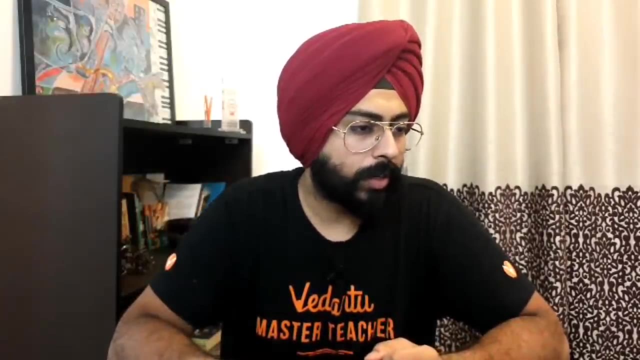 so now I can paste it in the chat box 220 times. Okay, Yeah, And I will also put that in the comment section of this video. Is NCRD enough for organic chemistry theory, part Mohit? it is almost enough, but we have epic GOC online. 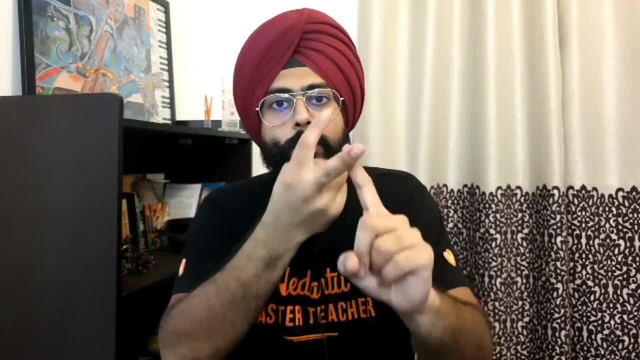 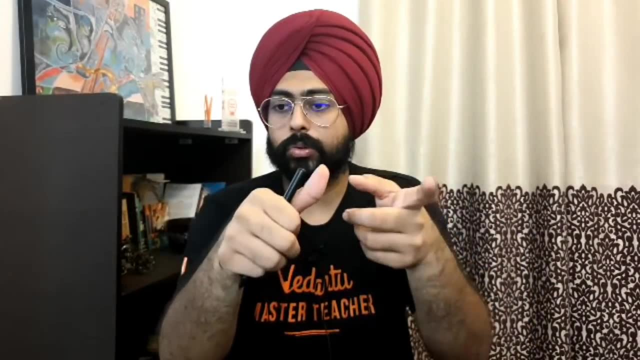 I have taken classes for general organic chemistry- very beautiful. I have done quick revision of GOC. I have done quick revision of alcohols, quick revision of aldehydes. ketones Amines is coming up and in June we will also do carboxylic acids and alkyl halides and whatever is a 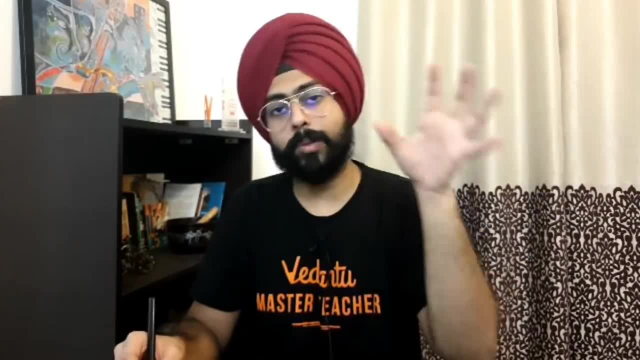 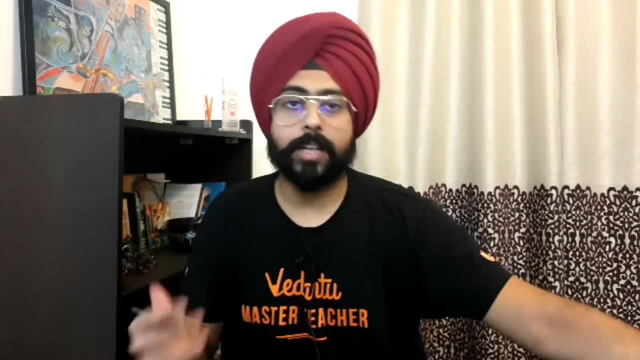 little bit more, So don't worry about it. organic will be covered in revision over here. but if you are in eleventh class or if you have just joined twelfth class, then NCRD is just the basic- Cool Awesome. 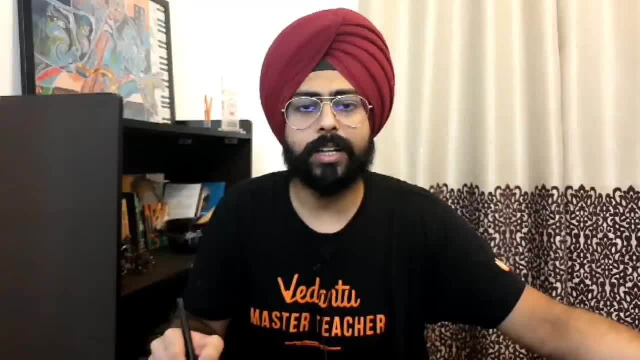 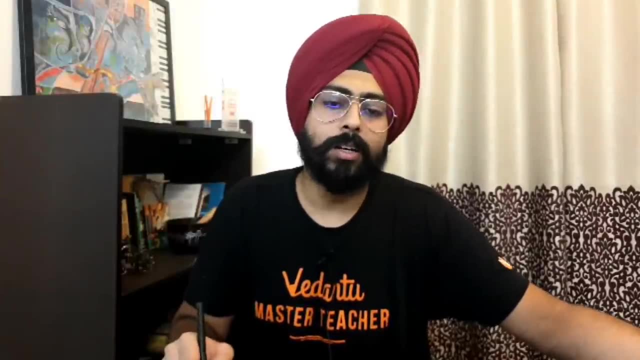 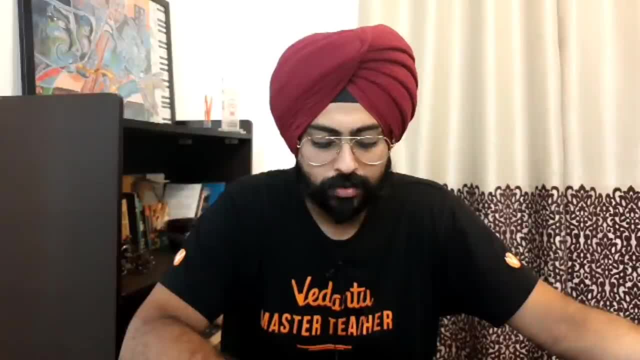 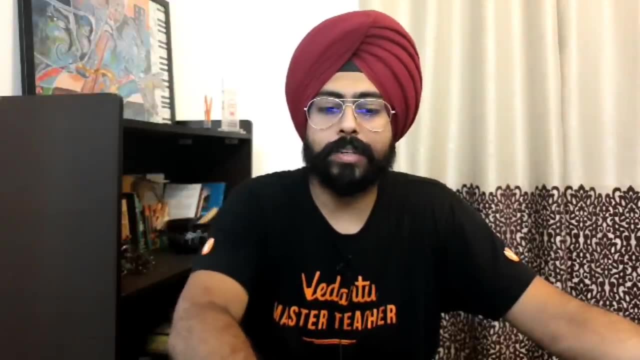 calculate the order of the reaction B Dixit is doing. See for calculations of how to do things. I have given you the hints today, exact how things are done. I will tell you tomorrow. There are multiple ways to calculate the order of a reaction. the best one of them. 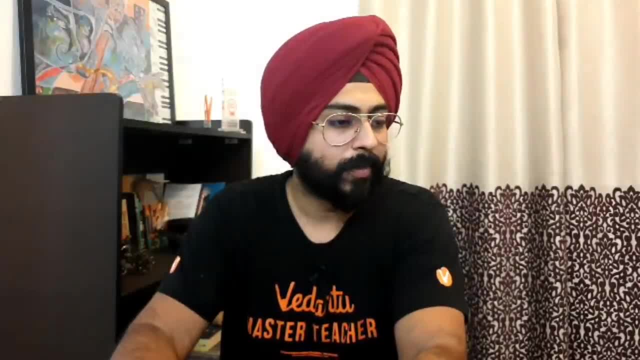 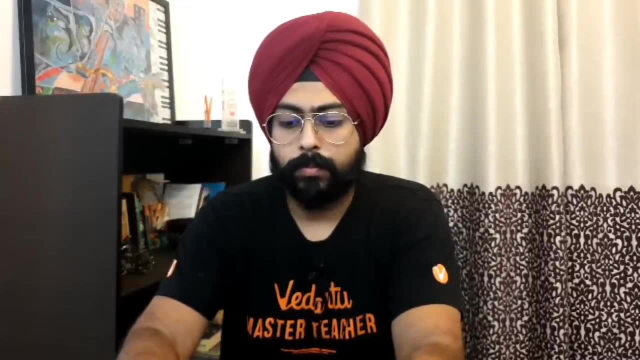 is trial and error. Okay, Cool, I am just putting the comment of the PDF. Okay, Now let's open our papers, okay, Okay, Okay. so now we are done with dashing up theory etc, and I have started planning for tomorrow's high schooler. hopefully that's sufficient, That's. 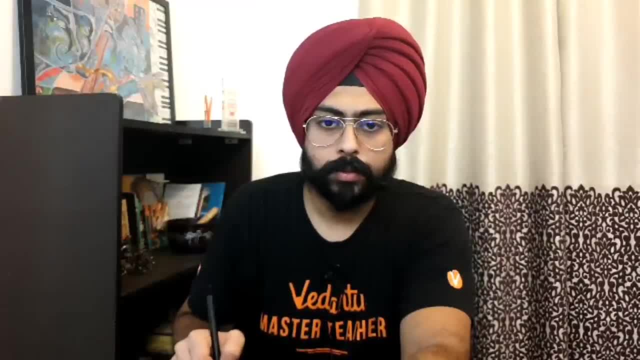 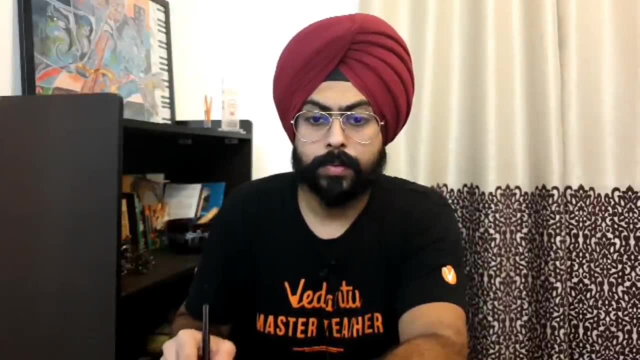 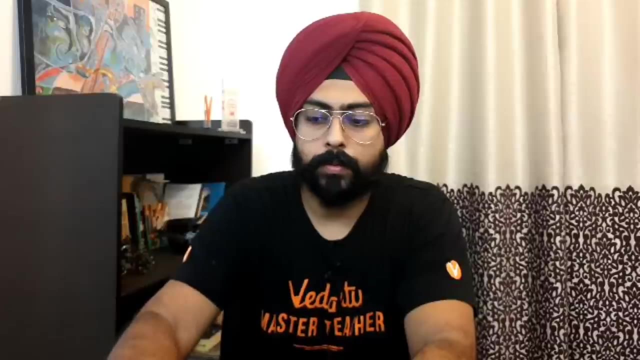 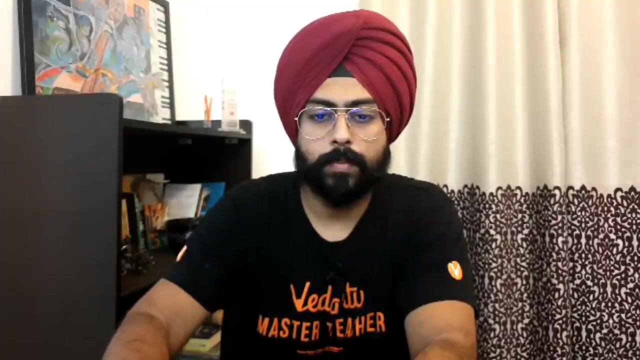 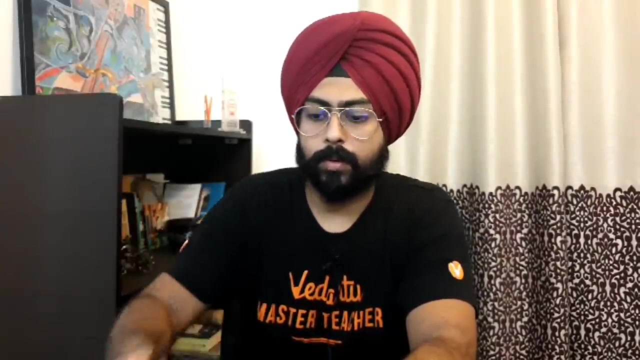 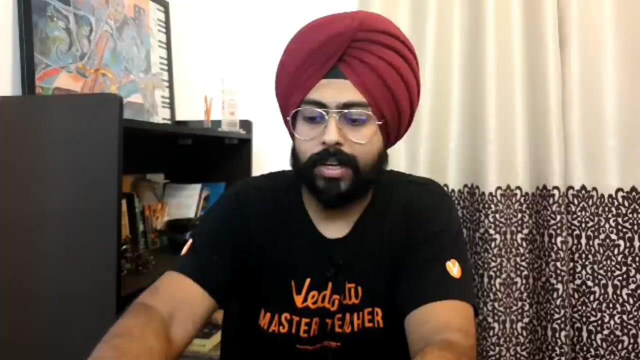 It's just. it's just Just two minutes. my comment is almost done. Anyway, later on I will cut the chat part of the class Because it has to be like a quick revision video, so I have to write it. Chemical Kinetics in 20 minutes yo. 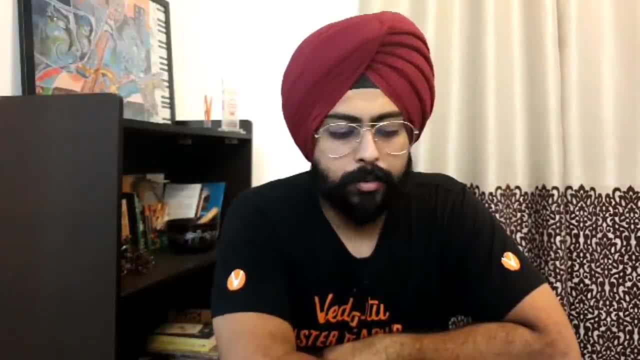 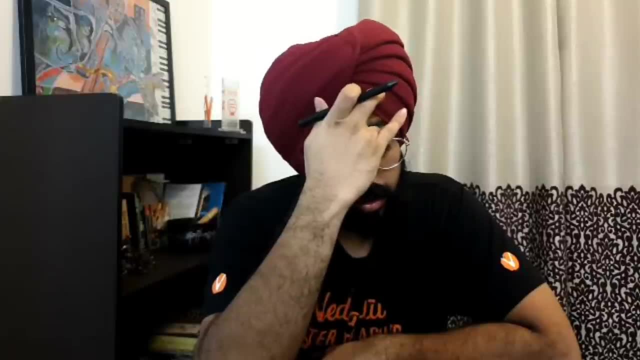 Bilal. I am not sure about the Eklavya classes, man, Because they would happen closer to JEE Advanced. Let's see, something is going on at Vedantu. If there is any more announcement I will get to know. I will announce it as well. 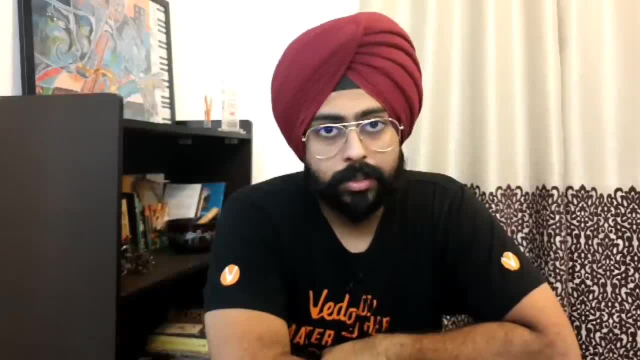 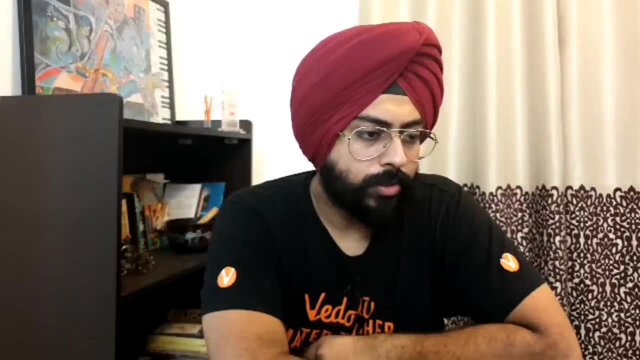 But in our Art of Deduction series we are doing the tough questions that people from Eklavya also do. Madhavi annotations: They used to be in New York YouTube Long back now. I don't think they allow annotations on YouTube. 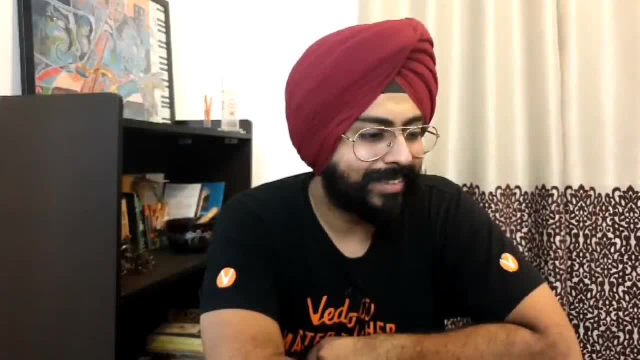 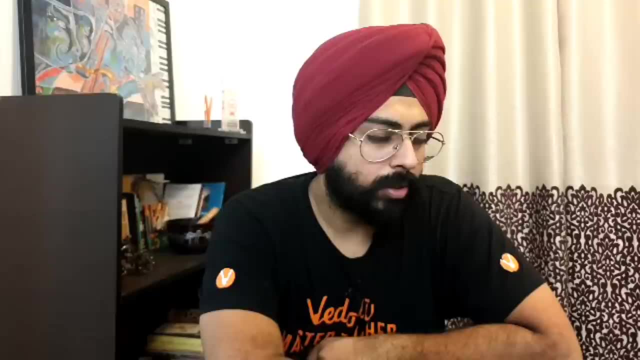 Oh, Mishika is saying the end caption of the ad was lit. Thank you so much, Mishika Sanskar. thanks man Meenal, just great, going on. Diabol-H reduces which carbonyl compounds See. Diabol-H is there to reduce compounds which are more reactive. 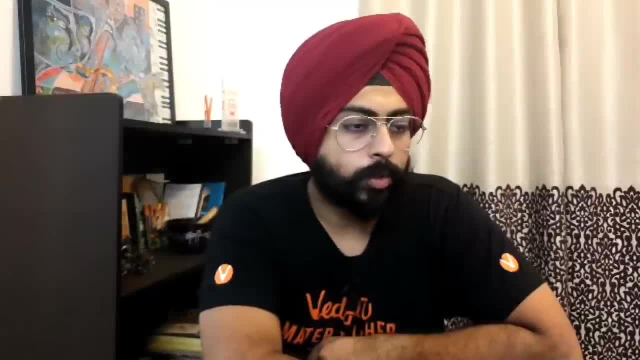 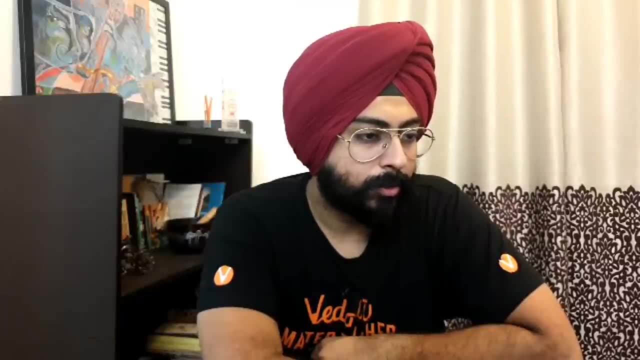 Because Diabol-H itself has less reactivity. So revise it once. See for yourself, Aldehydes. Okay, fine, Tanuj is saying: will you give me your bike for one day? No, Tanuj, sorry, You earn your own money, take your own bike. 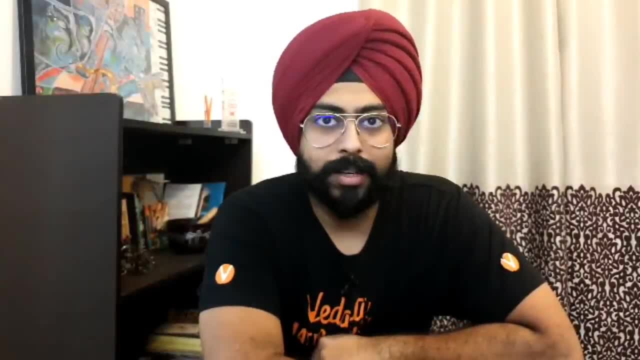 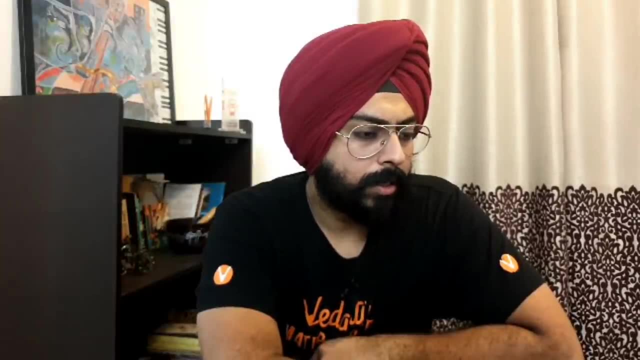 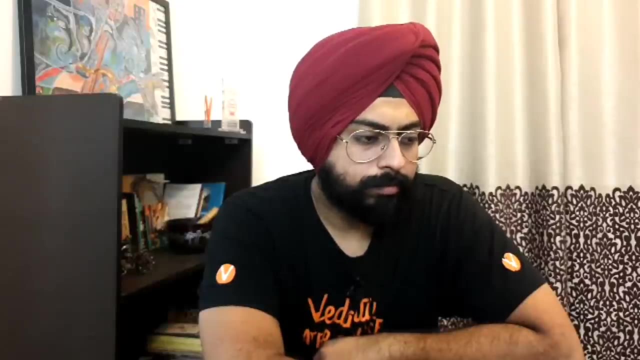 Then we can exchange for some time If you have a bike of your own. Aryan says the interface. Okay, Aryan, I will definitely take your point and send it across. Do one thing, Bro, just do one thing. 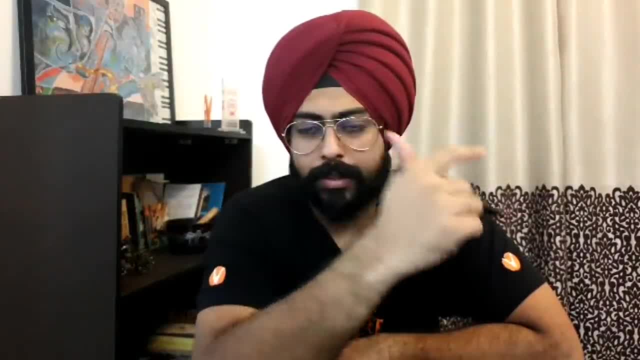 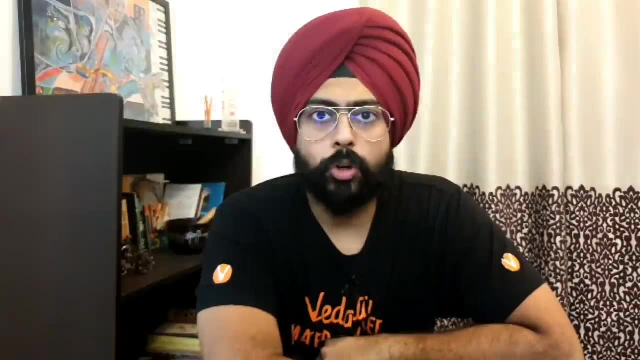 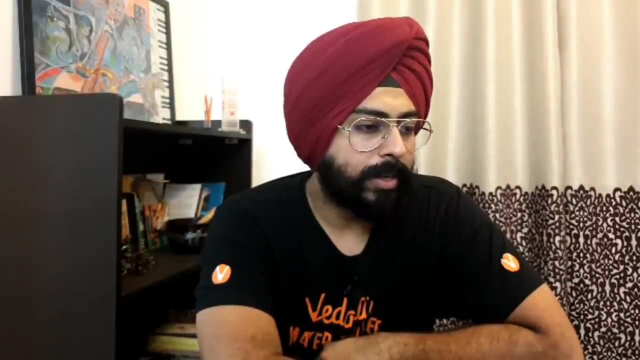 Give me your email id. Just comment down your email id in this video and I will forward your concern to the tech team. Okay, Kewri, I am not sure, but there are lots of chemistry teachers at Vedantu. Will they mention whether the reaction is pseudo first order or not? 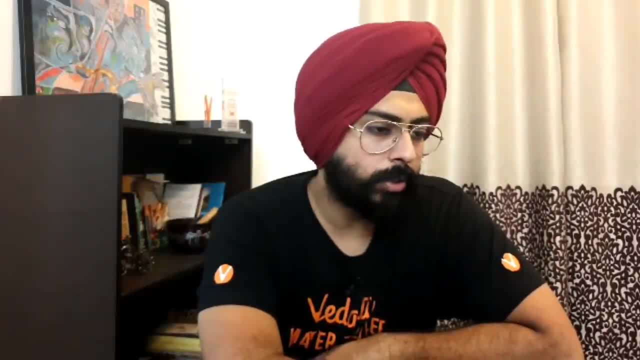 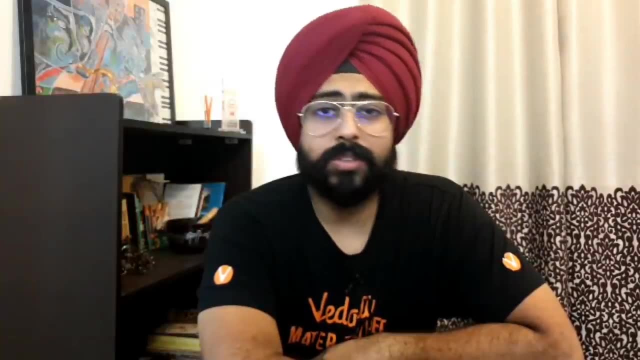 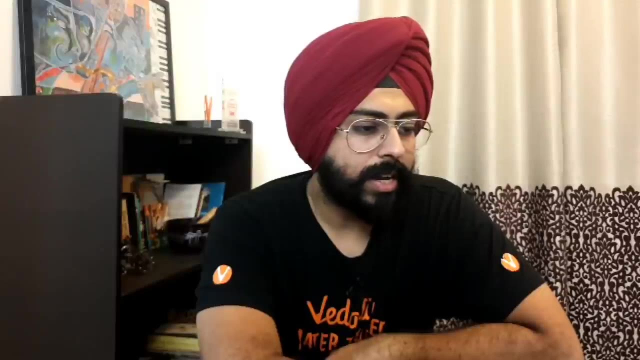 Parikshit, they will give you a hint. They will definitely give you a hint somewhere. Okay, Why am I not in crash course? Because I am here at catalysis. I can't do 20 things at the same time. PDF of this class. Srinivas, I have put it in the comment section down below. 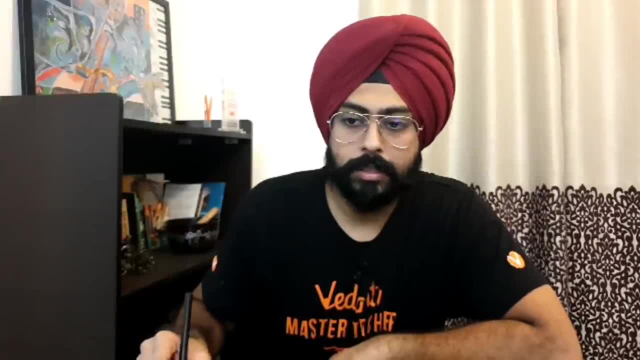 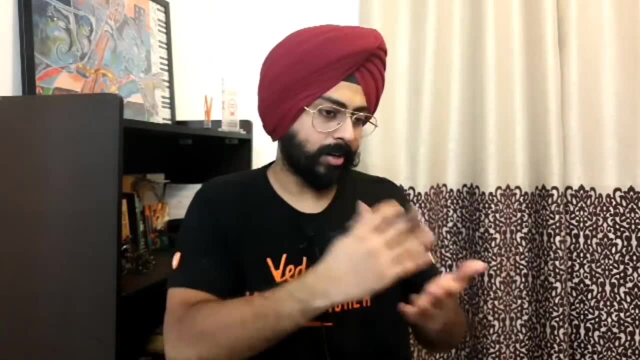 You can check out the comments of this class. Okay, So friends, thank you so much for joining in. I will take your leave. I had a lot of fun today. This was a quick session. I will cut out the chatting part of this so that later on I can change the title to chemical. 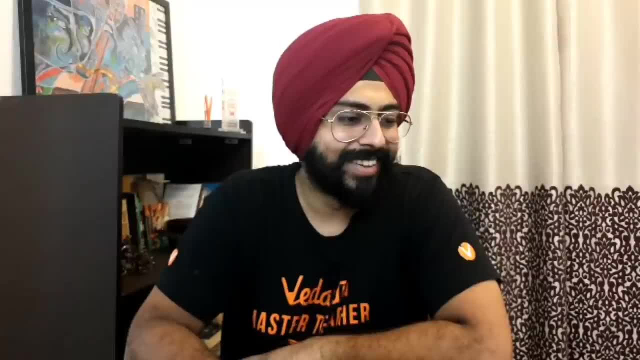 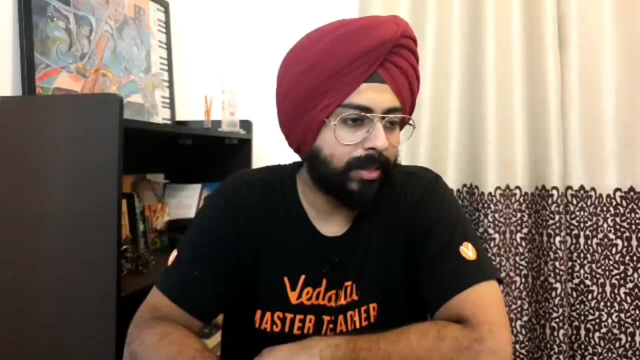 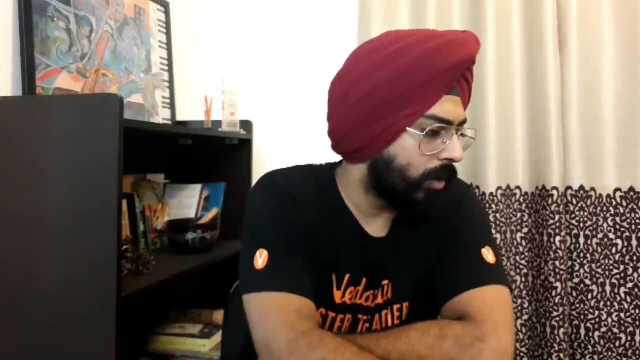 kinetics in just 20 minutes. Yo, It's yo. Okay, Gautam, I have already answered that. MCRT for organic. Okay, Abhi todhi dil pehle hi bataya maine Electrochemistry Tridha is towards the end of this month.